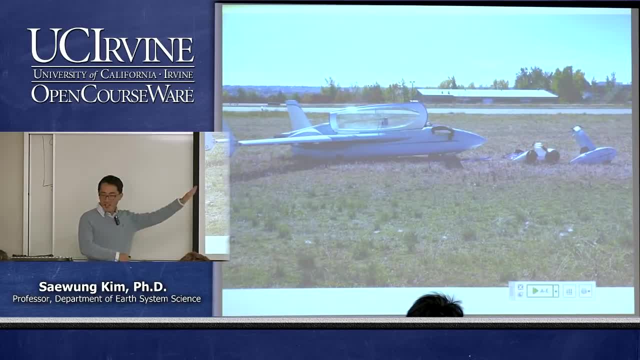 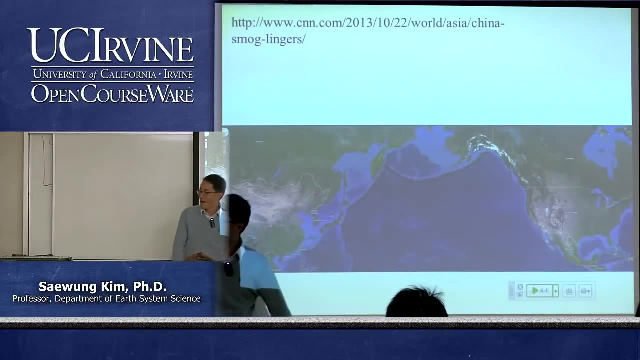 happened that you guys four weeks of the hard work kind of gone, if I died or something. So this was your lucky day, right? So feel lucky. So we talked about it's late October, so winter is coming, So we are right here. And then 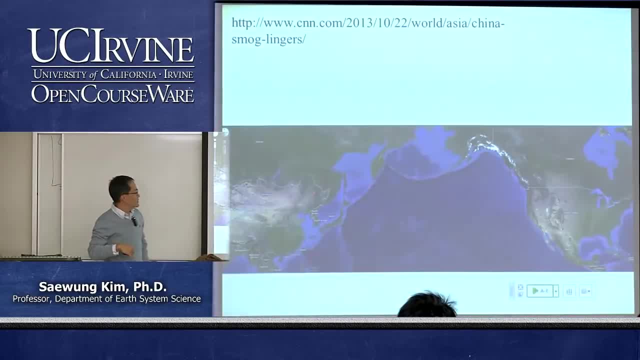 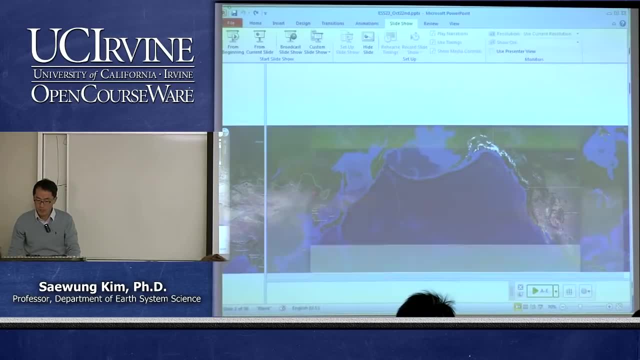 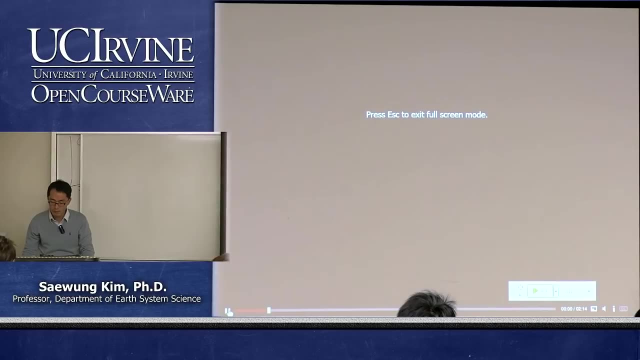 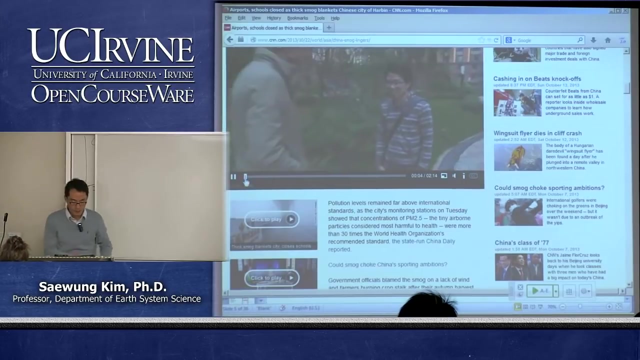 we will just take a look at the news coverage that happened yesterday in the Harbin, China. So let's take a look at this News coverage. people, We start our class. What's going on? Yeah, this is not good. 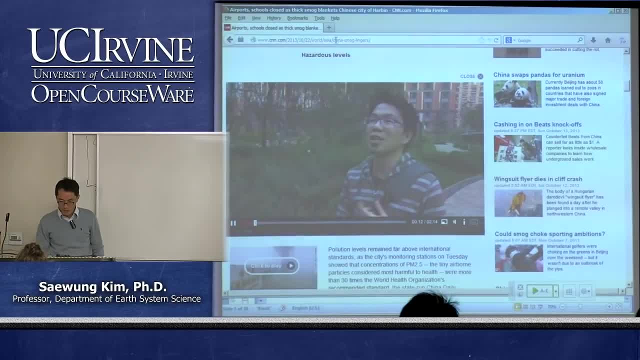 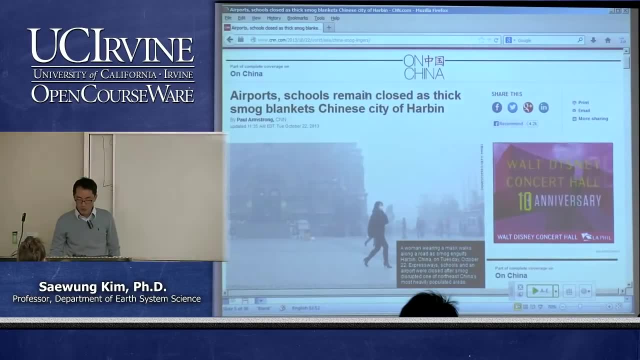 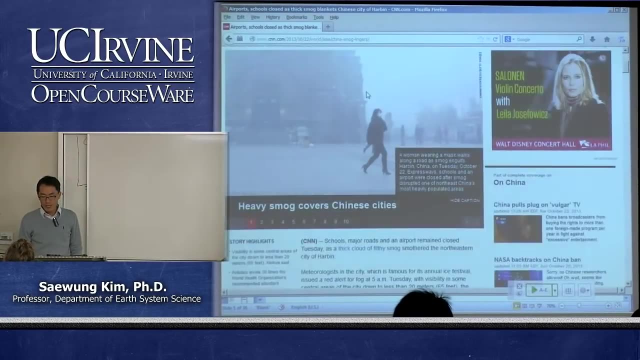 Let's try again. We may need to watch the commercial again, but whatever. So this is the before we actually watching this video clip. So this is kind of big, kind of London type smog event out there. And then if you read this news article, what it is saying, 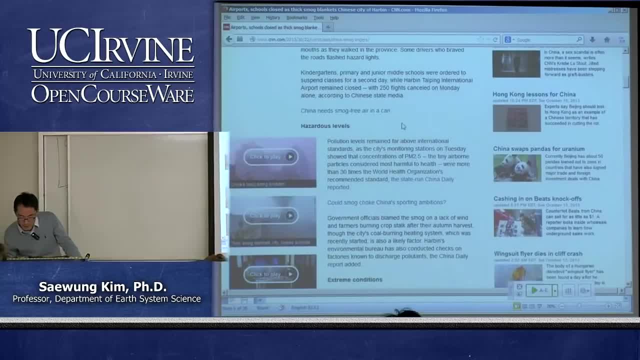 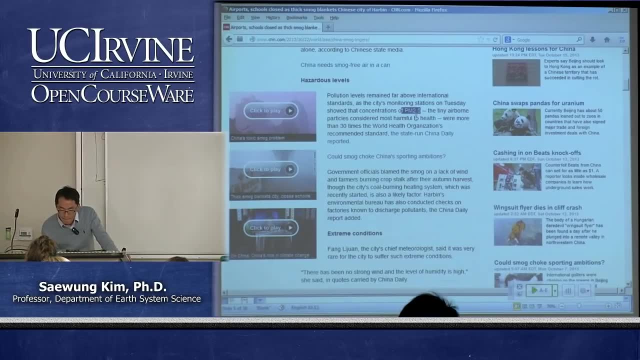 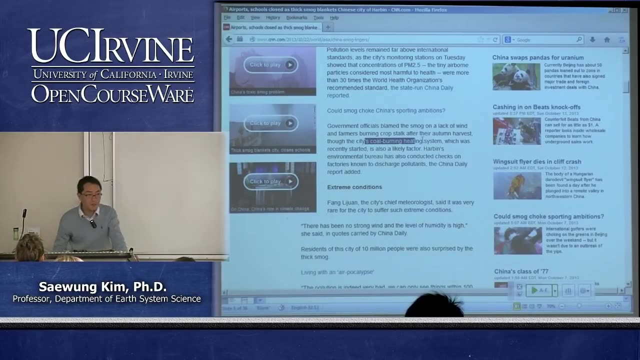 is that? let's see where it is. So it's talking about PM 2.5.. It's obviously particle pollution. And then there's a coal burning heating system. That sounds familiar. It's about the London type smog again. And then they are burning crop, So burning again, And then there's a 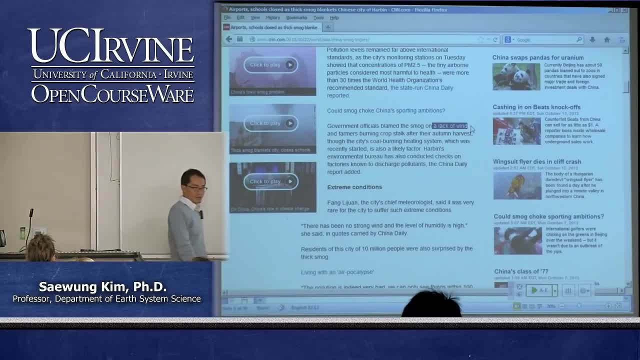 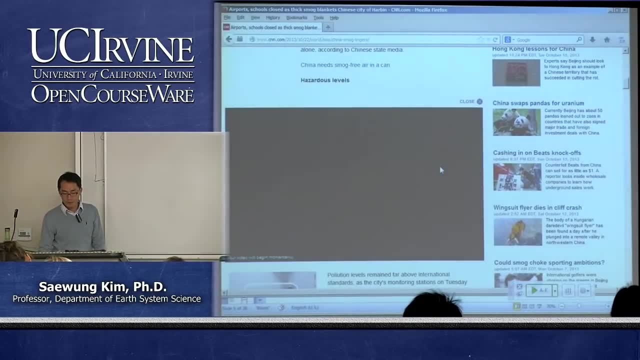 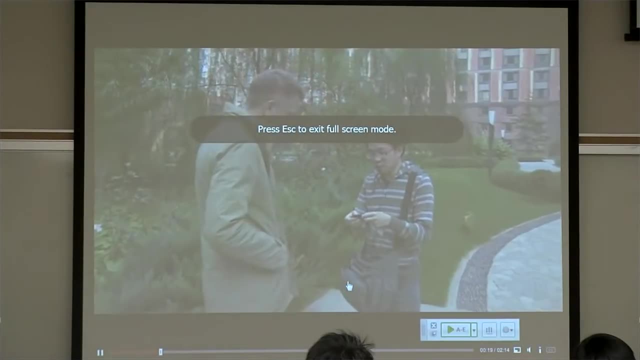 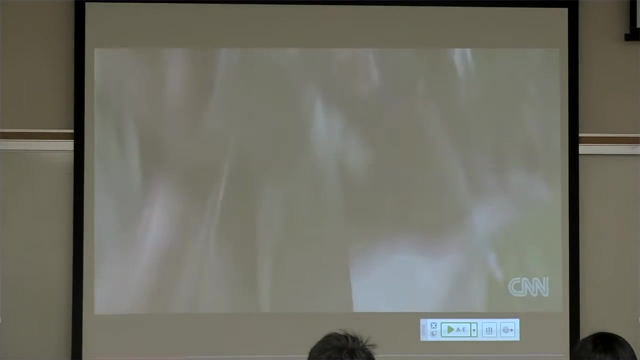 lack of wind, So that's high pressure system, So it's combination of emission and then meteorology too, right? So let's watch this coverage. It's quite simple because it's basically just like this sort of magic tip here. So my idea is to always take- obviously already taken. 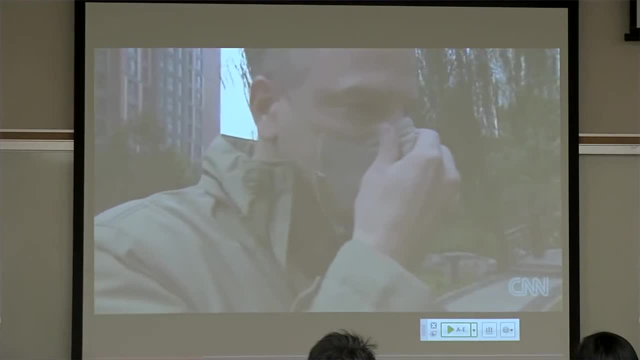 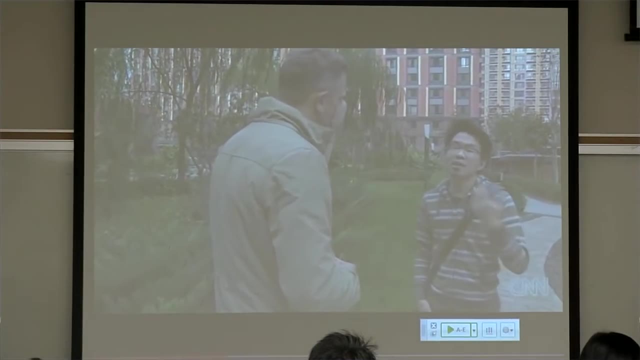 Imported from the US. it's designed to filter out particles and gases for long term health benefits. You can't go back in time, right? If you go back in time, the damage is done. The damage is done. Yeah, It's always done. 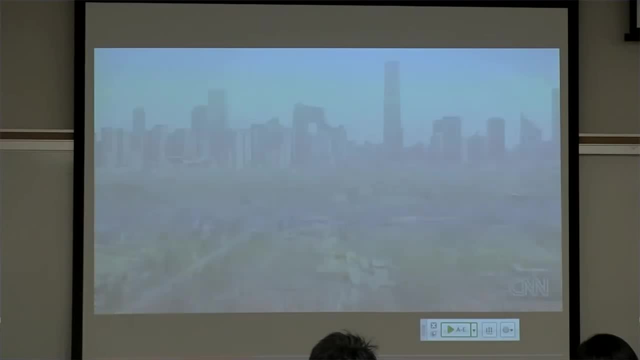 Yeah, So the difference between a blue sky day here in Beijing and a polluted one can be dramatic. Right now it's rated as very unhealthy by the US Embassy monitoring site, But in Harvard in northeast China, the pollution is off the charts. 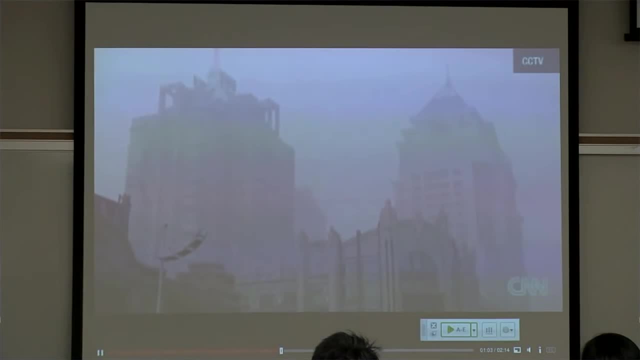 Dense acrid smog brought this northern city of 10 million to a standstill. Schools are shut, dozens of flights cancelled, highways closed, visibility down to almost zero, Pollution- 40 times the WHO recommended standard. The local government blamed it on. Harvard's coal-powered central heating turned on over. 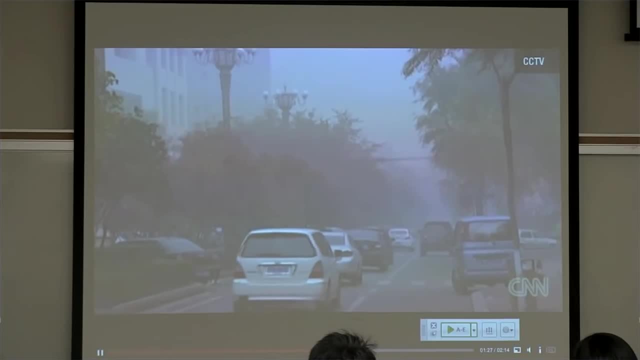 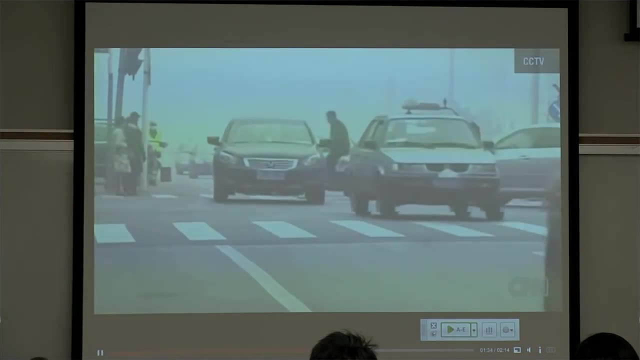 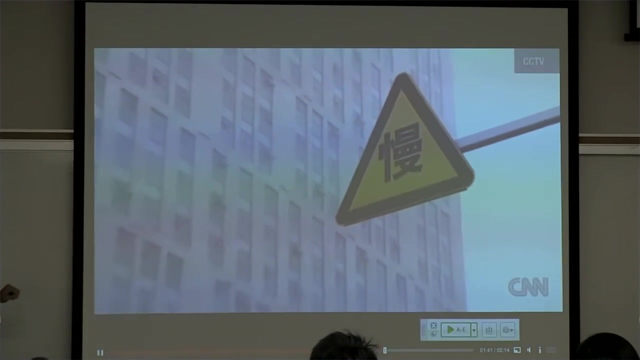 the weekend. But critics say China's pollution is a terrifying side effect of the country's decades-long obsession with growth. Wary of social unrest, Communist Party officials have announced new stringent measures. They want to meet their own acceptable standards by 2020.. 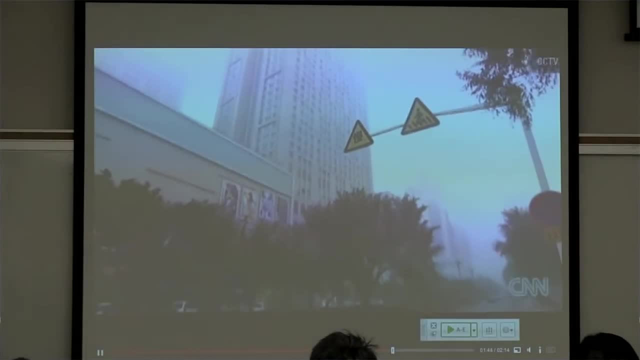 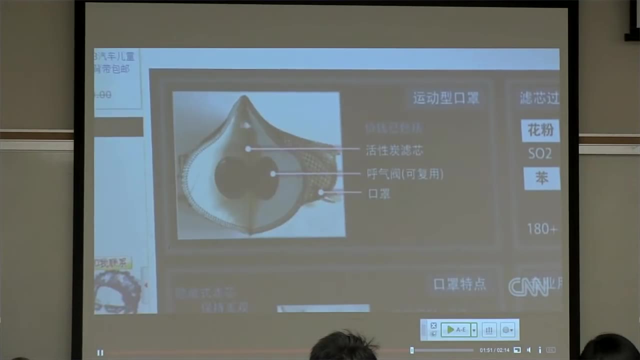 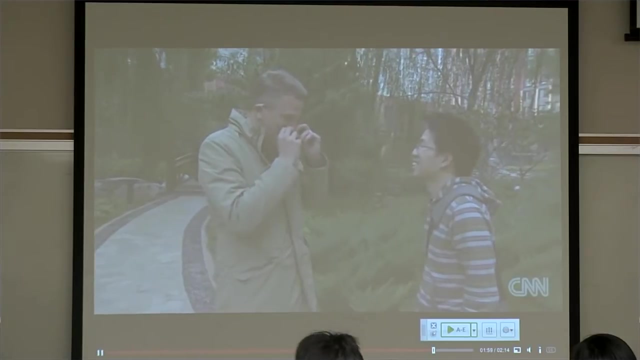 The WHO's standards by 2050.. You have to breathe in through your nose, and That's good news for now's growing business. They're struggling to keep up with demand, catering to all kinds of tastes, Selling a product for the new reality of China. 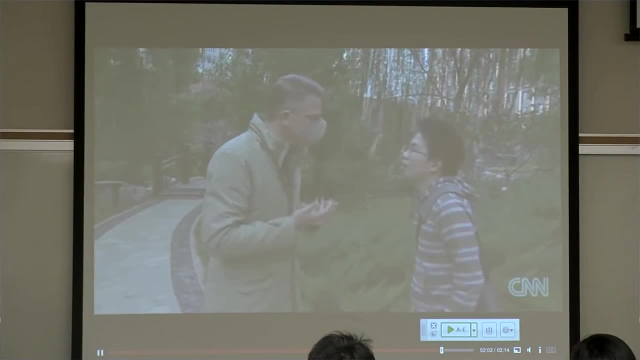 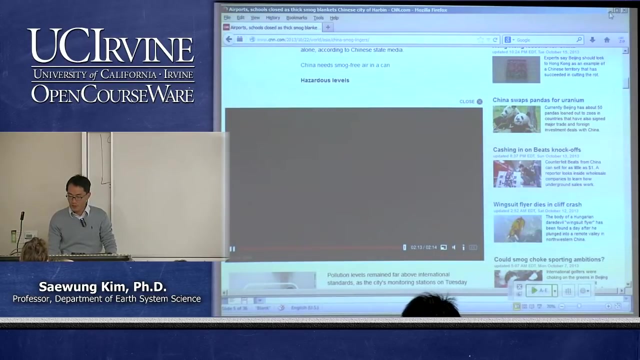 Do you think people are getting used to wearing something like this? Um, I think it's okay. It's a reality that could last for decades. David McKenzie, CNN. Well, uh, already, business is out there, but it's hard time to keep up the demand. 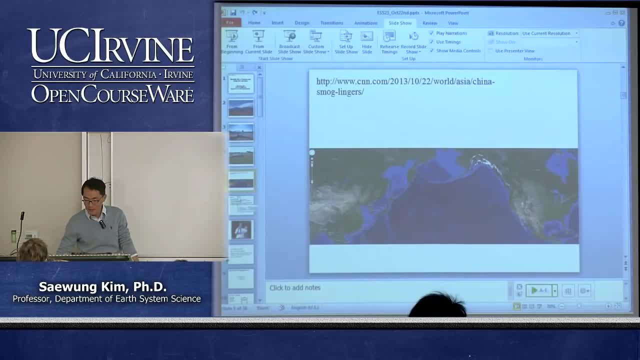 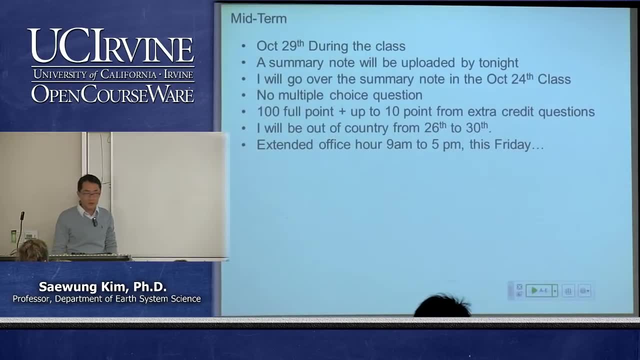 so you can just- you have a good idea- just go for the business. So that's what's going on in the world out there and then, uh, this is what's going on. what will be going on next week. 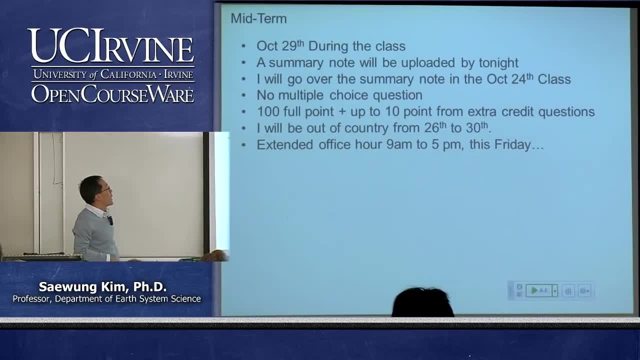 But at the same time, this uh today there will be a uh midterm, so October 29th during the class right, And then, uh, a summary note will be available. It will be uploaded by tonight. so I already finished to uh uh, finalize the uh midterm. 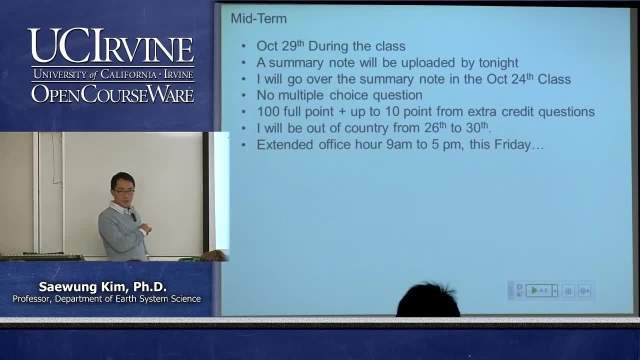 questions, And then there will be no multiple choice questions. And then, uh, I will go over this summary note this Thursday, right? And then there will be 10 points of extra credit questions. And then, because I will be out of country between basically this Saturday to next Wednesday, 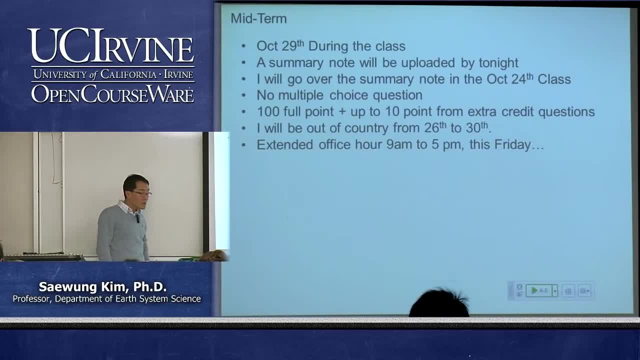 so I will extend my office hour this Friday 9 am to 5 pm. So if you have any question, feel free to visit my office this Friday. All right, Any other questions about midterm Ready, Not even prepared. 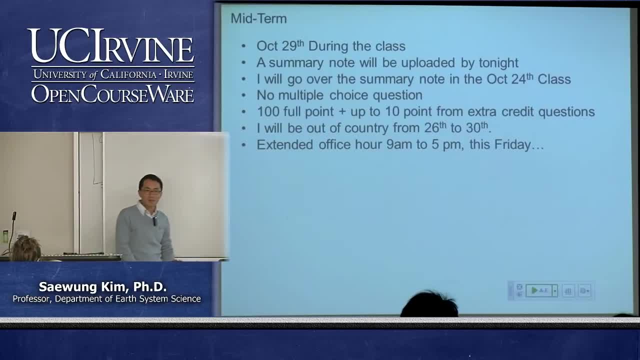 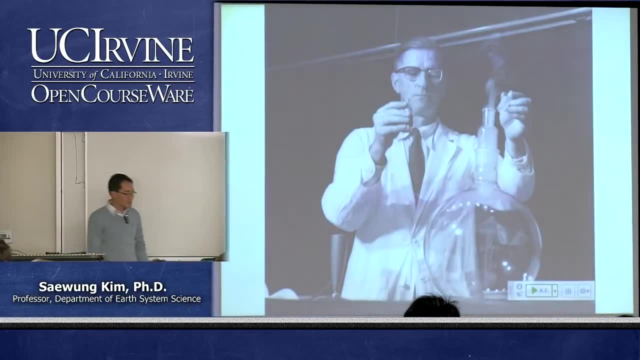 Anything, You have plenty of our time, No question. Okay, So we have talked about chemical reactions of gases And particles, That's about the air pollutants, right, And then, uh, from this lec—today's lecture and the next one, we will discuss about how. 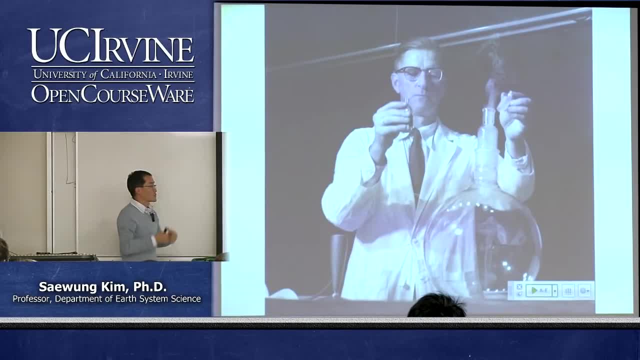 those air pollutants are moving around in the atmosphere. So this is kind of an iconic photo about uh studying um chemical reactions, uh that uh is happening in the atmosphere in the context of air pollution. So, uh, as a chemist- just—I call myself a chemist- 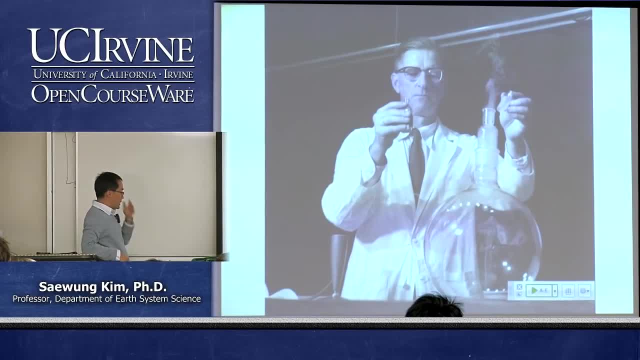 And then what we are interested in is that what's going on in the atmosphere in terms of reaction. So we assume that atmosphere is a sort of chemical reactor And then we are studying chemical reaction in gas phase and particle phase, uh happening in the atmosphere. 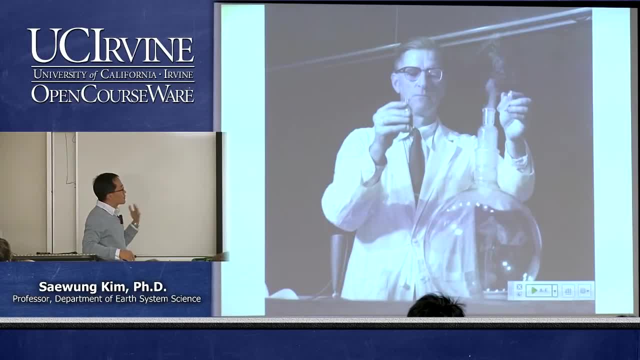 Basically, we can uh make the uh small glass bulb like this, And then we can make the uh chemical reactions uh, just like what's happening in the atmosphere. But if you think about the Earth, anybody knows about, uh, about the radius of the Earth. 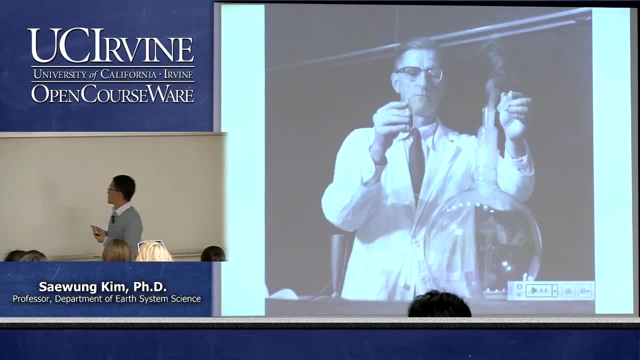 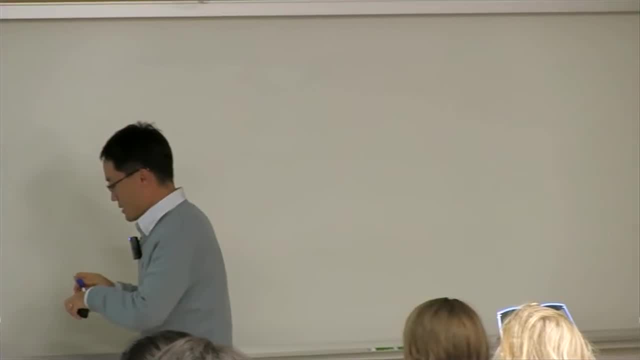 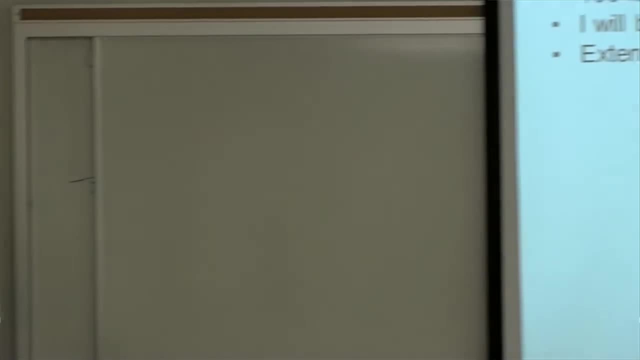 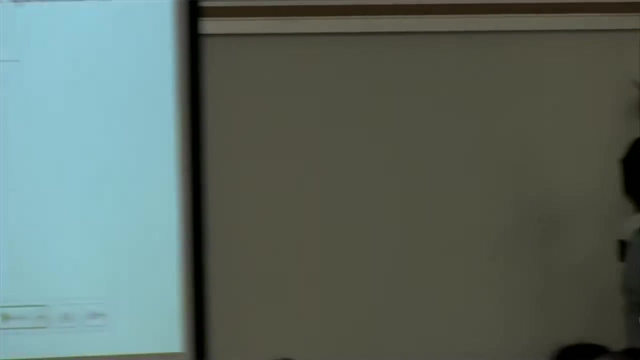 6,400 kilometers, So a diameter is 12,000 kilometers. So this is not good at all. Let me use my. So diameter of Earth is 12,000 kilometer, So let's assume this is Earth, This is center. 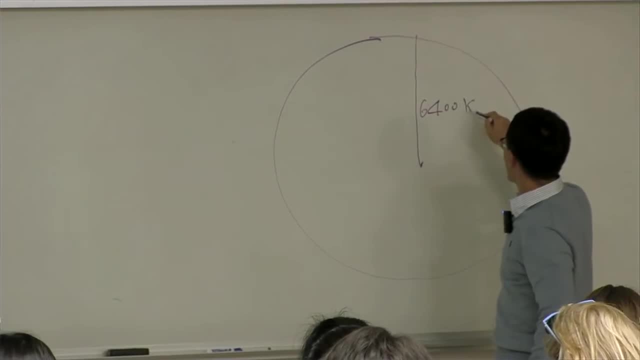 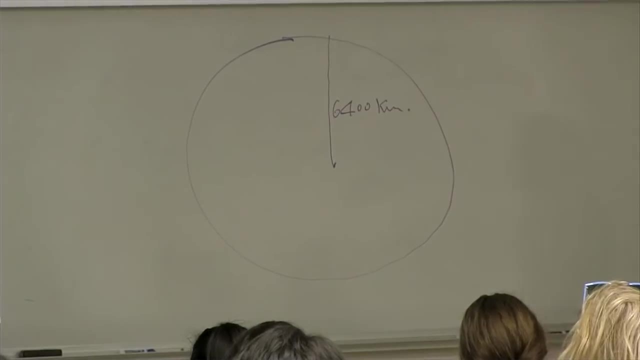 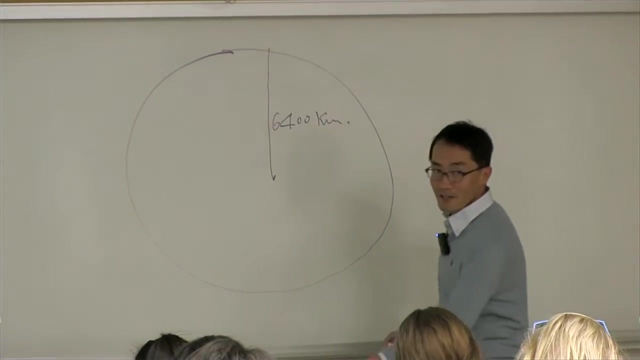 So this is 60—6,400 kilometers. Anybody knows that? uh, height of the atmosphere or troposphere, Anybody. Any guess, 10 miles, 10 miles is a good number, 10 kilometer, let's say. 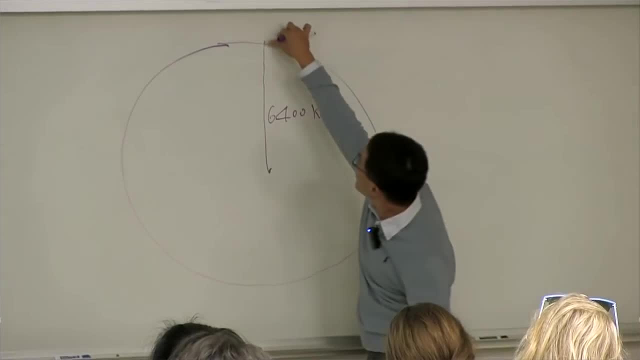 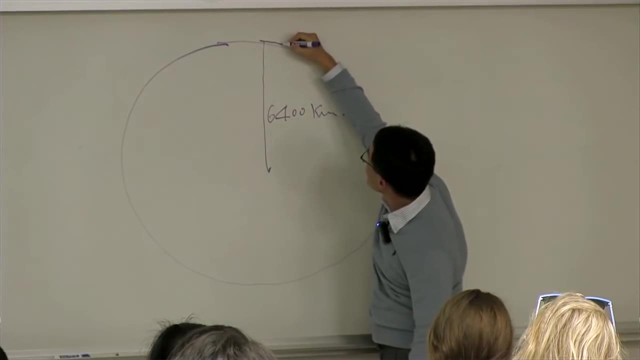 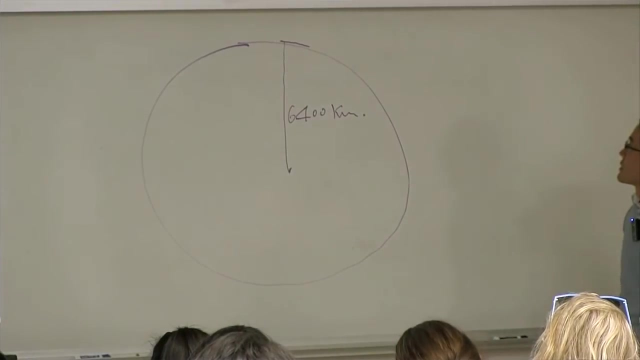 So 6,400 to 10 kilometer. What's the fraction of this thing? Probably something like this, right? So atmosphere is like this big surrounding the Earth, right? And what's the size of the core with respect of this thing in terms of pollution, pollutant emitter. 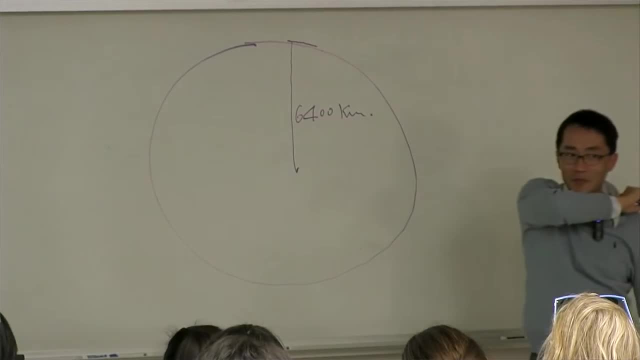 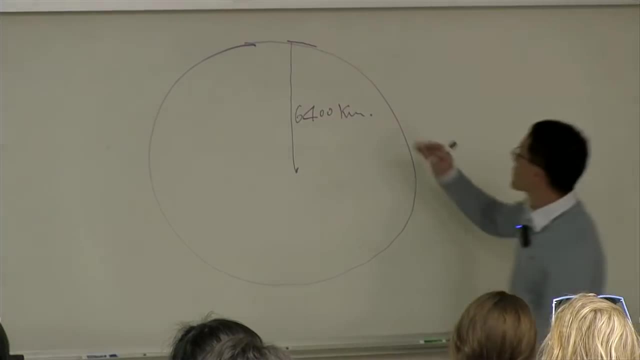 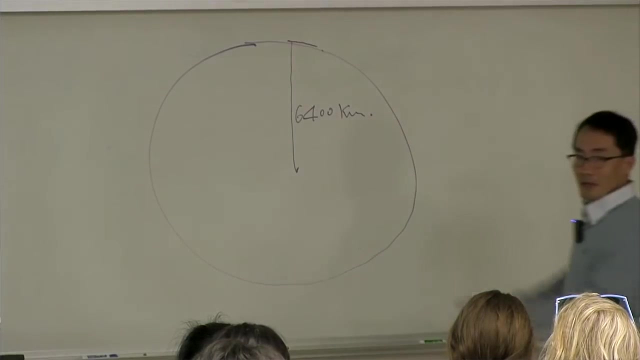 Kind of a tiny bit of the uh point. Probably this point is probably over-exaggeration If you think about the scale, right? So all those pollution is happening very, very tiny scale, And then atmosphere is kind of big, big, big chunk of air surrounding the Earth. 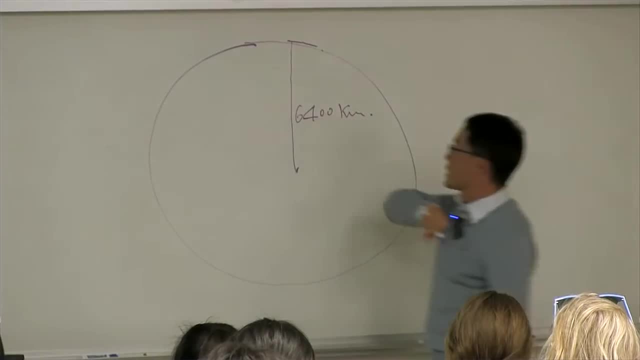 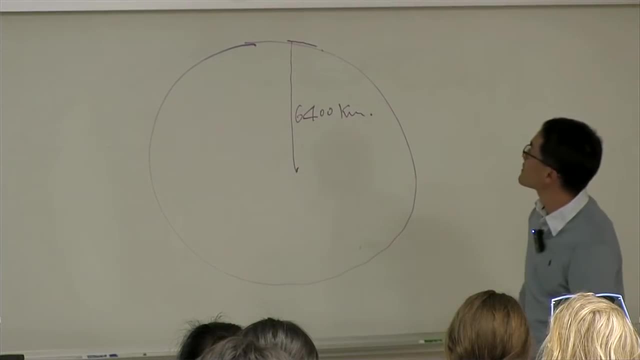 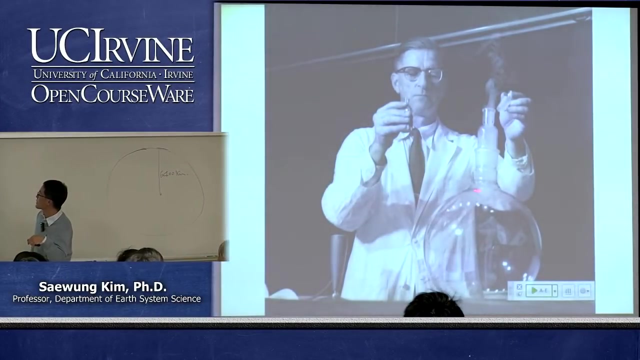 although it is very, very thin layer compared with the Earth's radius right. So basically, what I want to say is that it's very different. from Where is it From this? uh, glass ball. Basically in glass ball. if something is happening, it's going to be mixed up pretty quickly. 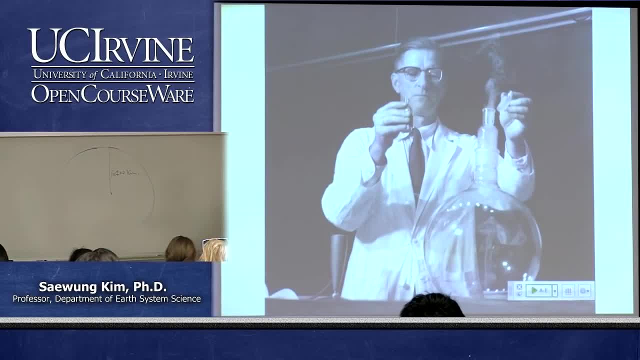 But in this kind of big picture of what's going on in the real atmosphere, then, uh, air pollutants, actually, kind of transport is very important because our pollution emission happens really really tiny scale And then our atmosphere is quite big dimension, Uh, dimension of the, uh in terms of space, right, 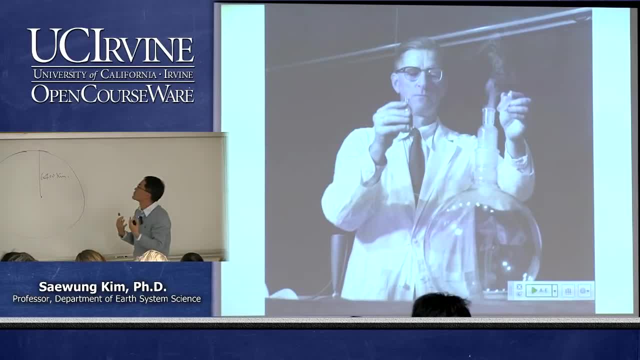 So, um, emission and then uh reaction in the atmosphere is one thing, And then how those air pollutants are transported in the atmosphere is another thing, right? So we will uh discuss about how air is moving around in the atmosphere. 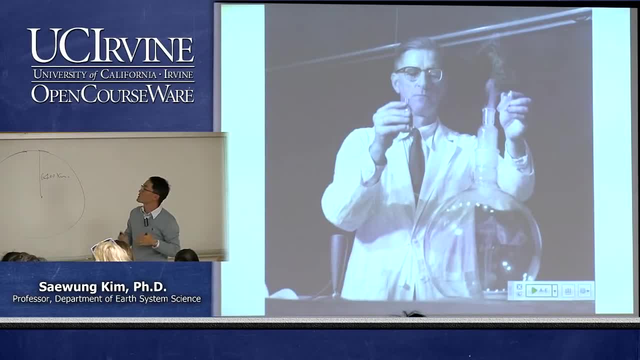 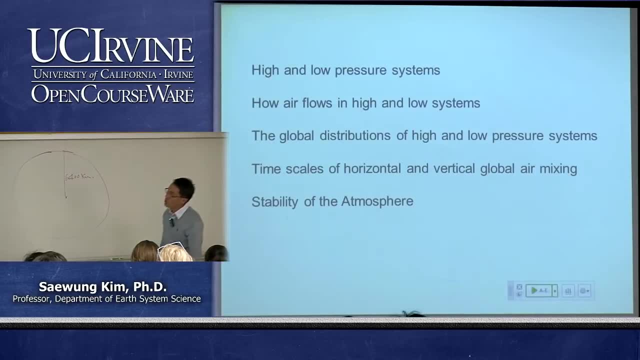 Basically, that dictates how uh trans, uh air pollutants are transported from one place to the other place. Okay, So we'll talk about high pressure, low pressure system today, And then, uh, today mostly uh, we'll talk about horizontal uh air flow uh in the atmosphere. 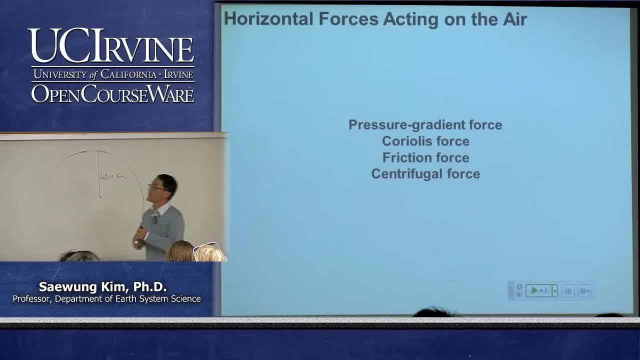 So to understand um air, um movement, uh in the horizontal scale, we need to understand uh about four different forces, But uh, most important forces is the pressure gradient force, Coriolis force and then friction. 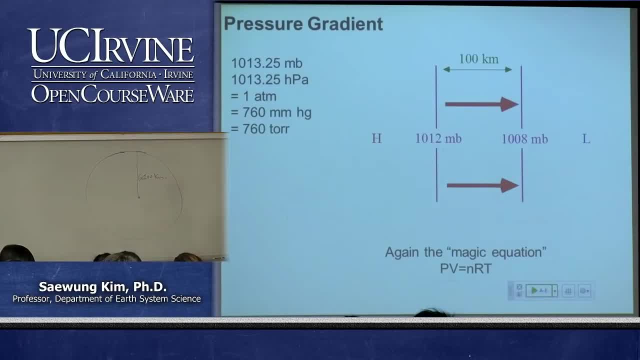 So let's discuss about that pressure gradient first. So whenever we uh watch the uh weather forecast on TV news, um the uh weather person usually talk about how pressure- high pressure system is coming, low pressure system is coming, things like that. 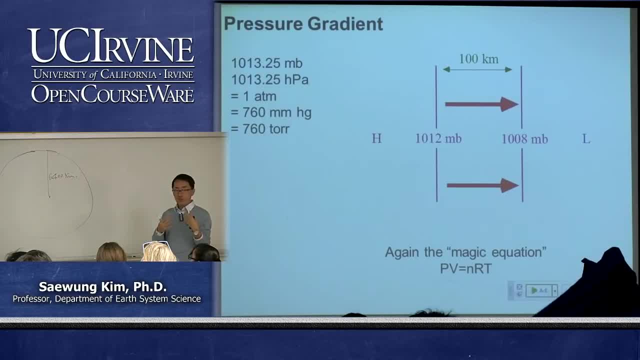 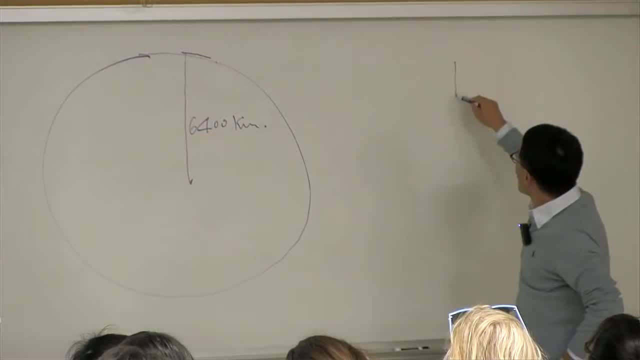 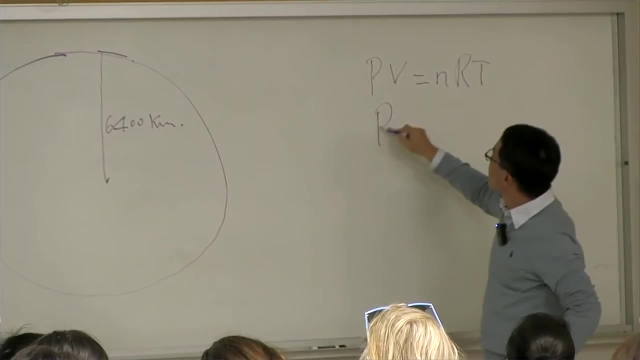 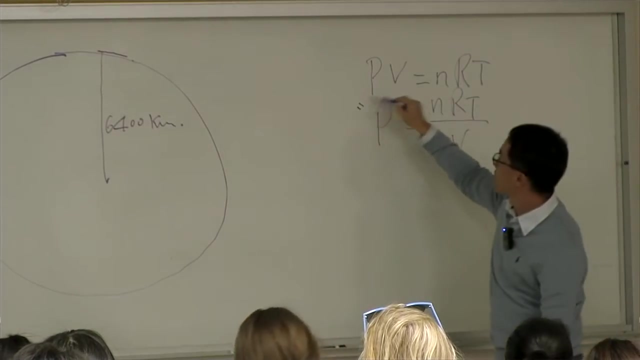 So that's basically same uh term that we were using when we discuss about uh uh, ideal gas law, So high pressure. It's basically that ideal gas law is: Pb equals nRT. And then let's arrange this equation with respect to pressure. 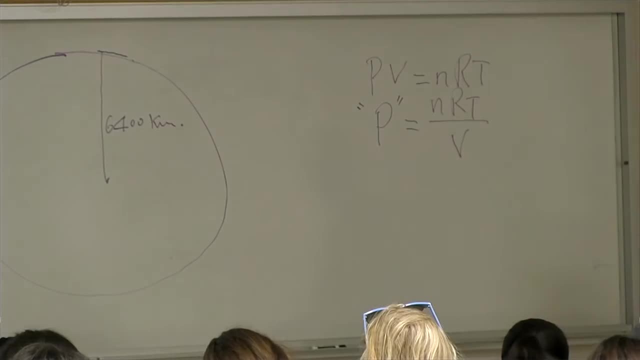 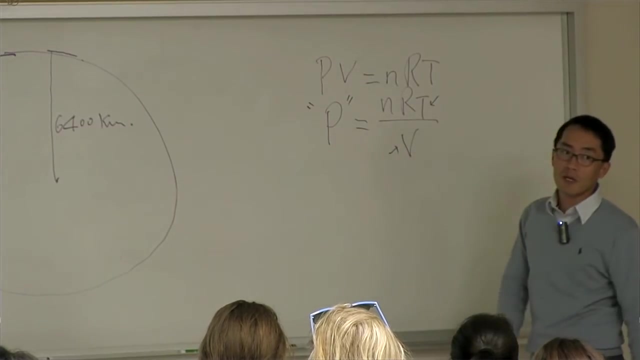 So high pressure, low pressure is all relatives right. Higher pressure or low pressure, lower pressure, right? So basically, if we assume temperature is same, volume is same, then what dictates the higher pressure and lower pressure Which is so? this is constant right. 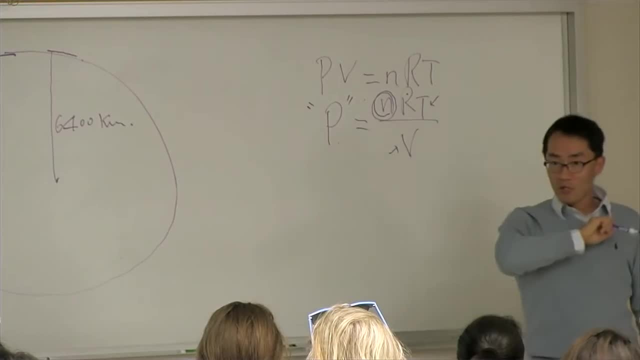 So it'll be dictated by n, which is number of molecules in the atmosphere. So high pressure system and low pressure system, if you assume just like that, and then there will be more number of air molecule in higher pressure system region than the uh low pressure region, right? 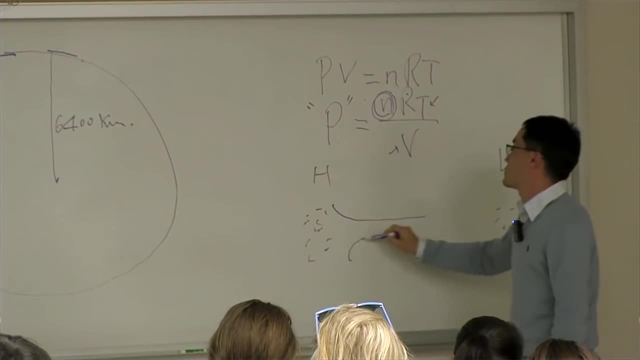 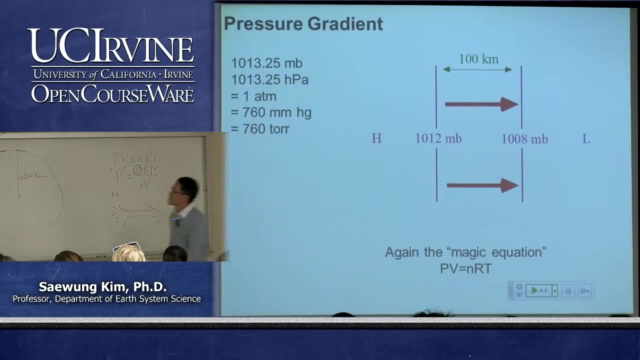 So what's gonna happen? Air molecule is gonna be moving. It's gonna be moving from high pressure system to low pressure system, right? It's pretty straightforward, right? So that's basically pressure gradient. So, basically, air is gonna be moving from high pressure- uh- region to the low pressure region. 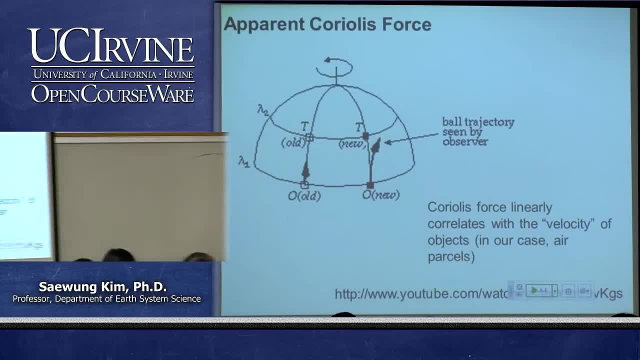 So that's pretty straightforward. But so, uh, the story is not that simple, Because air, uh the earth is rotating, So we need to uh factor in this uh earth motion into the uh air motion too. 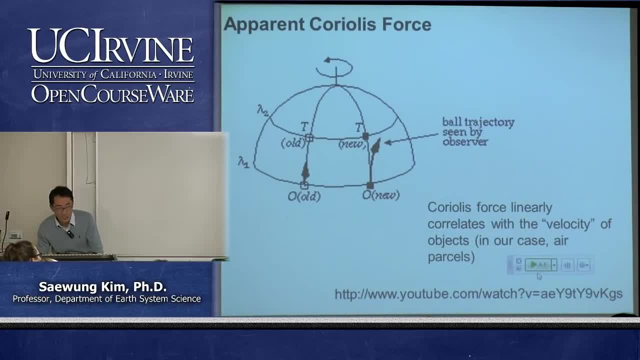 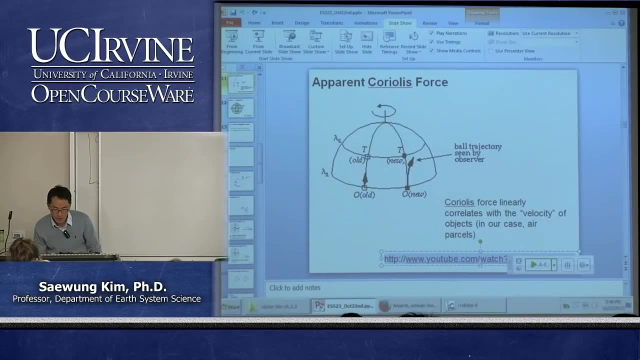 So, uh, because it is a little difficult to imagine kind of an earth scale rotation, just uh with a whiteboard, So let's watch this uh video which is pretty good on to explain how earth rotation is affecting air motion. 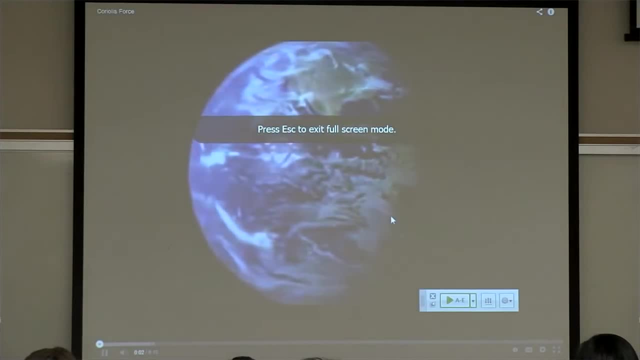 In this view of earth from space, it is clear that the earth is rotating. However, as an observer on the surface of the earth, the only indication our planet is rotating is in the observation of the sun during the day and the stars during the night. 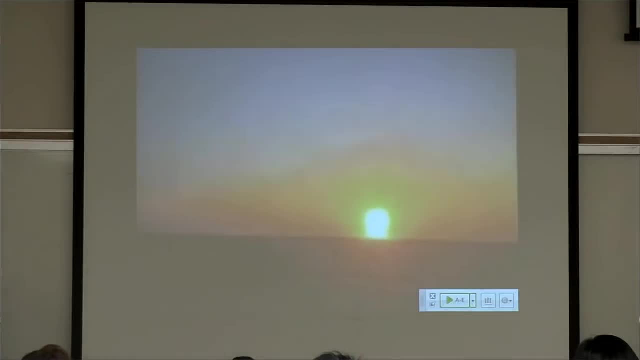 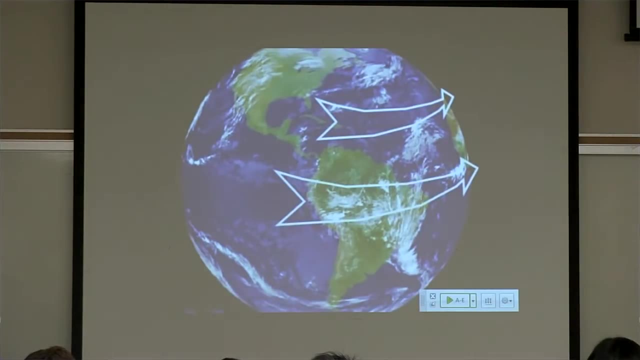 Every day, the sun rises in the east and sets in the west, But we are completely unaware that we are traveling to the east at hundreds of miles per hour. So just how fast are we moving? Well, at the equator, the rotational velocity of the earth is an incredibly fast 1,018 miles an hour. 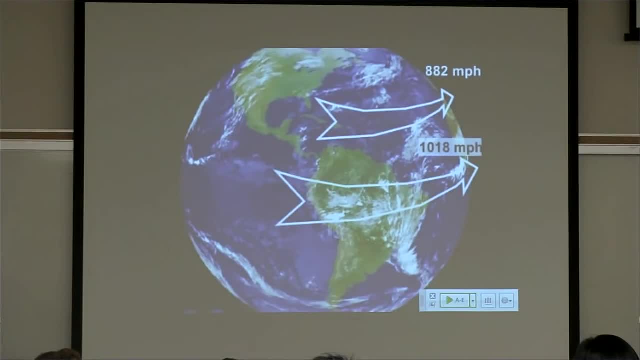 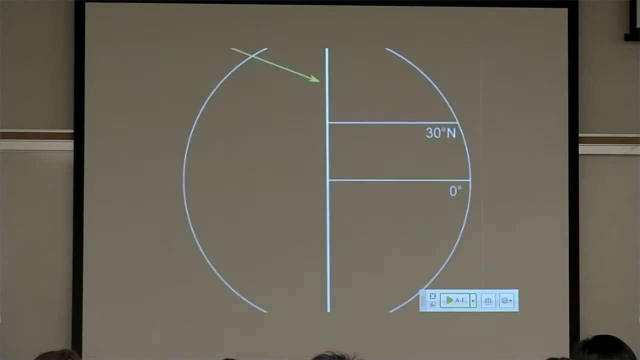 If you were to travel from the equator to about 30 degrees north latitude, the rotational velocity would have slowed considerably, to about 882 miles an hour. Well, why? Well, as you walk north or south of the equator, you are actually getting closer and closer to the earth's axis of rotation. 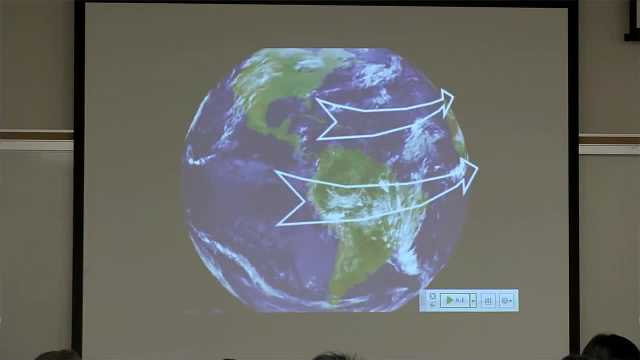 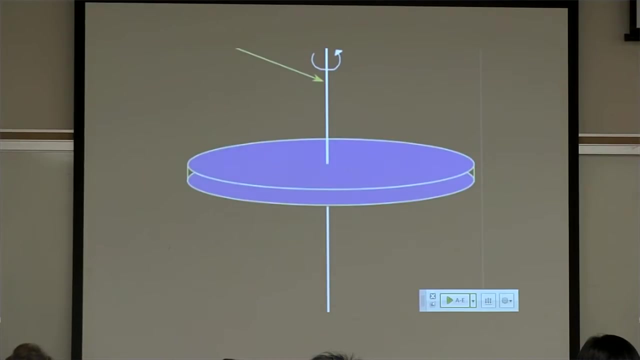 Because the surface of the earth is solid. the rotational velocity will decrease as you walk north or south of the equator, Because you are actually getting closer and closer to the earth's axis of rotation. To understand this better, let's imagine that we take the earth a sphere, and flatten it out into a rotating disc, like a merry-go-round. 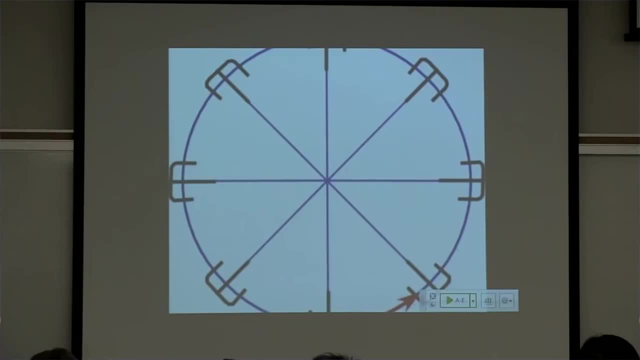 If you were to stand on the edge of the merry-go-round, the rotational velocity would be large and you would feel like you are going to fly off. However, if you stand in the middle, the rotational velocity would be much less and you would feel like you are barely spinning at all. 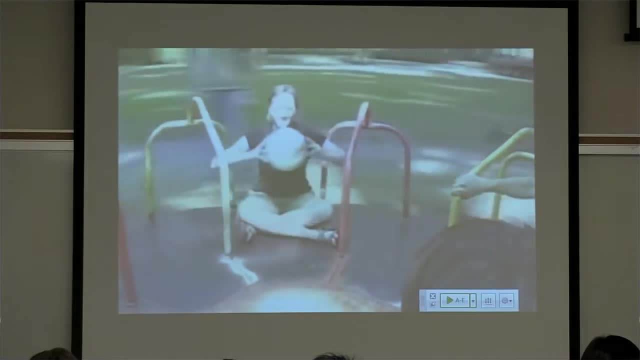 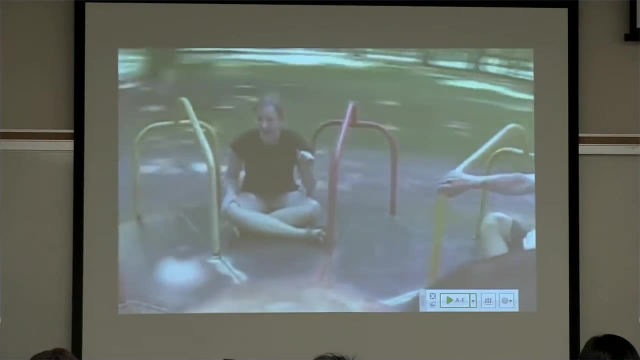 Now what if we were to have two people sit on opposite sides of the merry-go-round and try to throw a ball to one another? You can see that as the ball leaves the hands of the person throwing it, it becomes independent of the rotation of the merry-go-round and therefore follows a straight path. 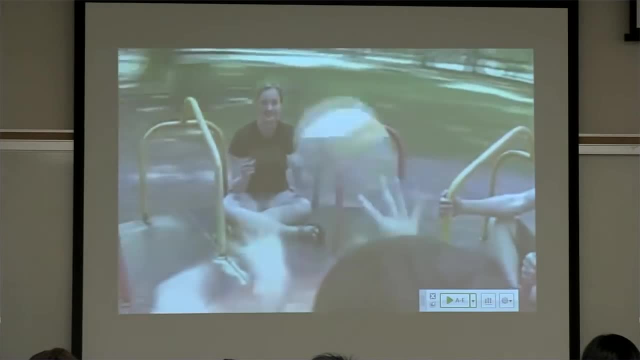 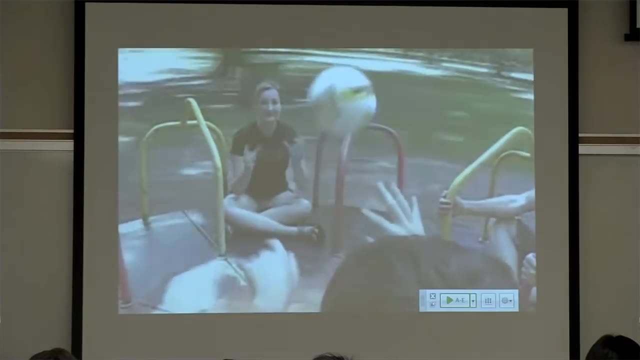 But because the person trying to catch the ball is still rotating with the merry-go-round, they are quickly moved out of the ball's intended path. Because the merry-go-round is spinning counterclockwise, this deflection is to the right. If it were spinning clockwise, the deflection would be to the left. 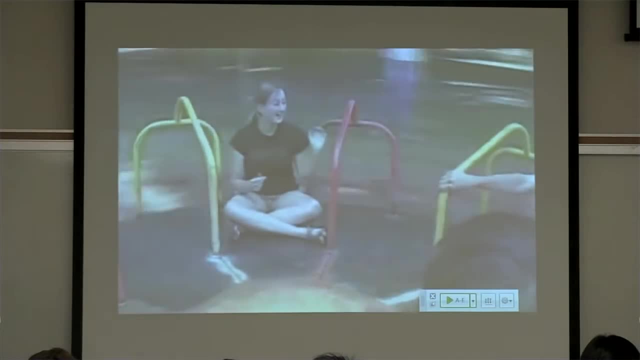 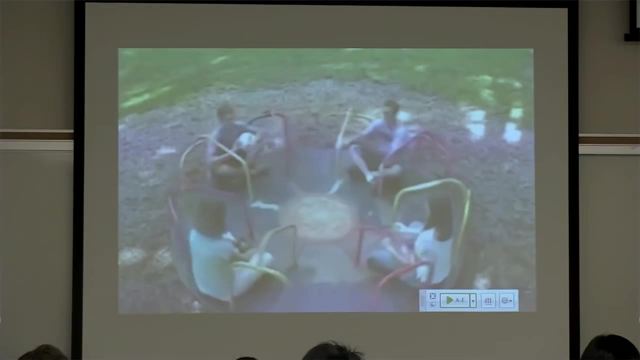 Now to an observer above the merry-go-round. the path of the ball appears straight. However, to people on the merry-go-round, the path of the ball curves to the right of the intended motion. This experiment demonstrates how the rotation of the merry-go-round appears to cause a deflection in the path of the ball. 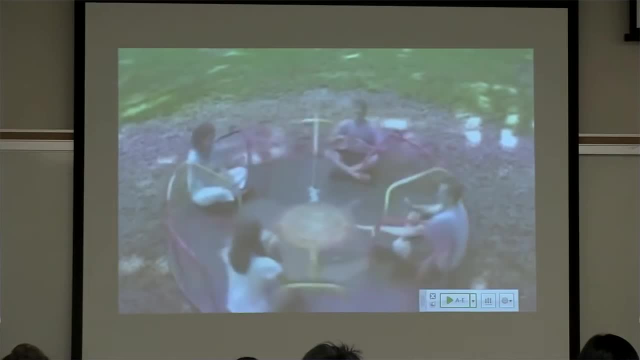 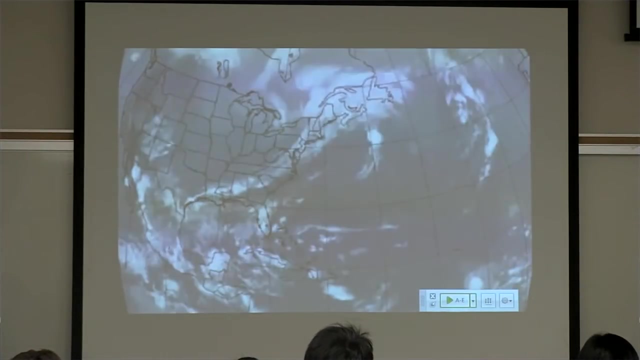 This also demonstrates how air movement on the Earth's surface can be deflected by the Earth's rotation, a phenomenon called the Coriolis effect. How do we relate the effects of the Coriolis force to air motion in our atmosphere? To answer this question, let's first investigate what would happen to a parcel of air. 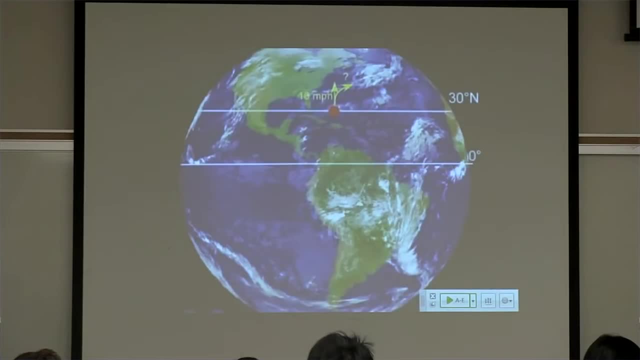 that was initially at rest with respect to the Earth. At 30 degrees north latitude, the parcel is traveling to the east with the Earth. But if we were to shove this parcel at 10 miles an hour to the north, what would happen to its motion? 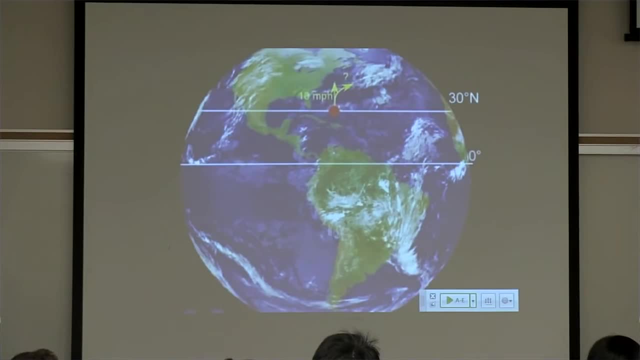 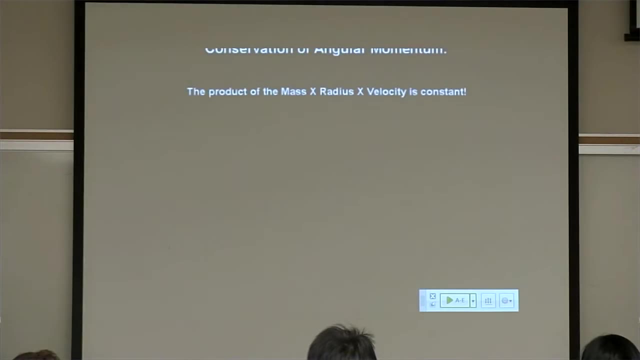 We have already seen from the merry-go-round experiment that the ball would be deflected to the right. But why? The answer lies in understanding something called the conservation of angular momentum. Angular momentum is the product of the mass times, the velocity times, the radius of a rotating object. 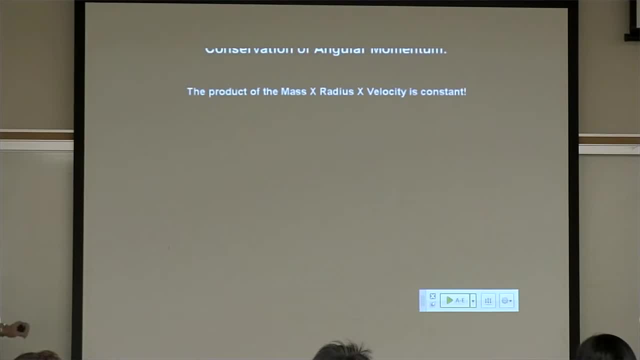 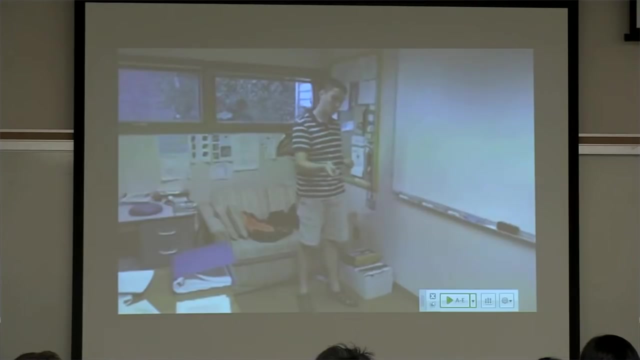 The conservation of angular momentum tells us that for a rotating object, the product of its mass velocity and radius is constant for that system. What does this mean? Think of a ball swinging around on a string. If you shorten the length of that string, the rotating ball spins faster. 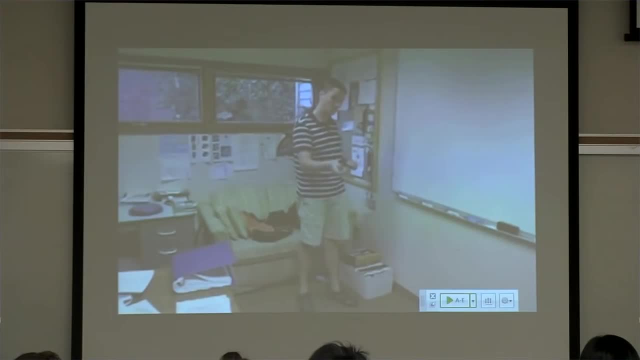 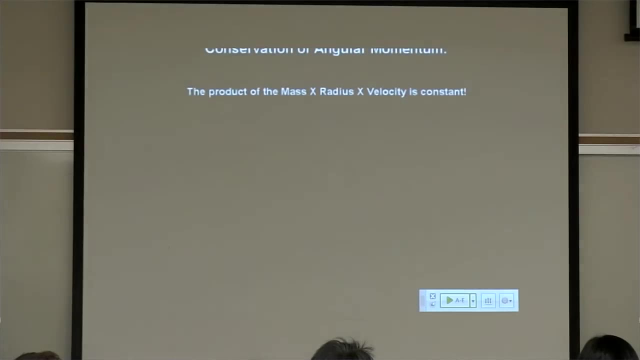 Angular momentum, however, is conserved because as you decrease the radius or the length of the string, the velocity or the rotational speed of the ball is increased, so that the product of the velocity times the radius times the mass stays the same. As an example, let's consider a ball that weighs 1 kilogram on a string that is 1.5 meters long. 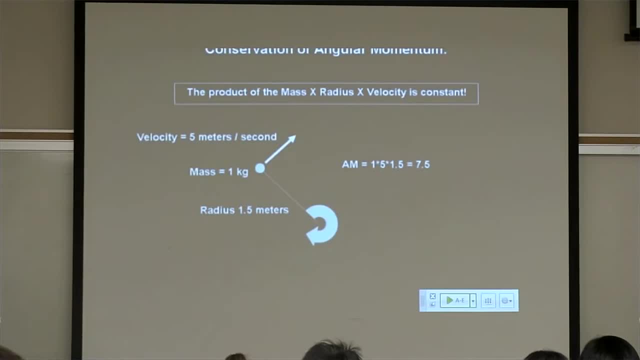 spinning at 5 meters per second. When we calculate the angular momentum, we find its value is 7.5.. If we shorten the string, we know that the ball will spin faster. So if the radius of rotation is reduced to 1 half meter, the rotational velocity must increase to 15 meters per second, so that the product of the mass times, the velocity and radius, remains at 7.5.. Now how does all this apply to this parcel that we shoved north? Well, as we moved it to the north, the rotational speed of the earth will decrease. 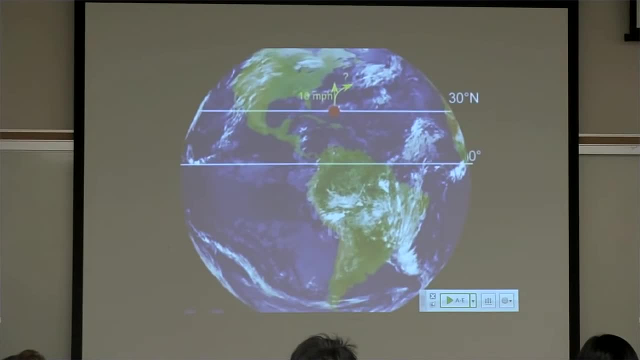 However, because the parcel of air is actually moving closer and closer to the axis of rotation, its rotational velocity must increase by the conservation of angular momentum. If you were standing at 30 degrees north and watching the parcel as it moved, it would appear to be deflected to the right. 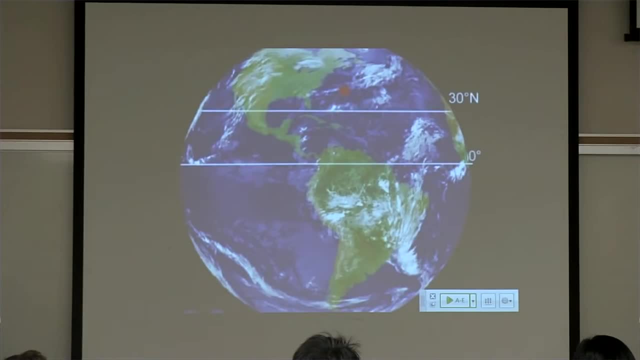 This apparent deflection is the direct result of the Coriolis force. What is really interesting is that if the parcel continues to be deflected, it would trace out a path along the earth's surface that kept its original speed of 10 miles an hour. 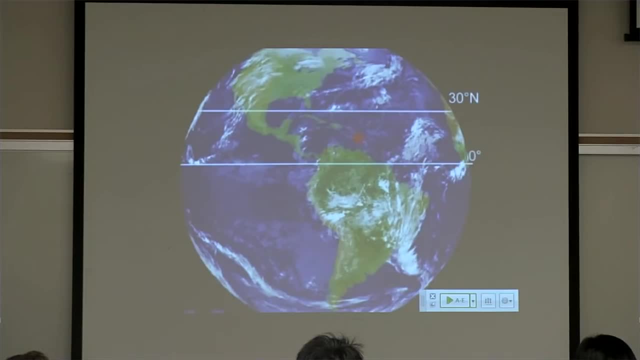 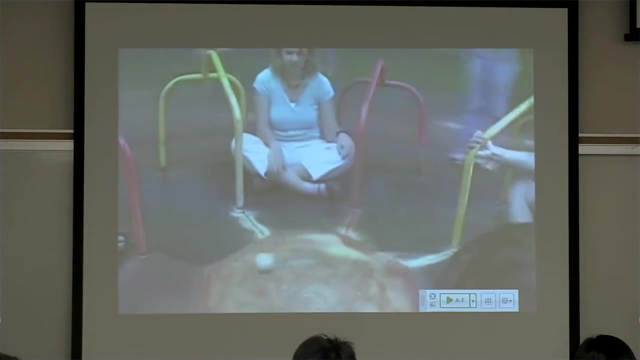 constant with respect to the rotation of the earth. Therefore, the path of the parcel would eventually trace out a circle, much like the path of this baseball on the merry-go-round Watch, as Amanda pushes the ball out to the center and it makes a complete circle back to her other side. 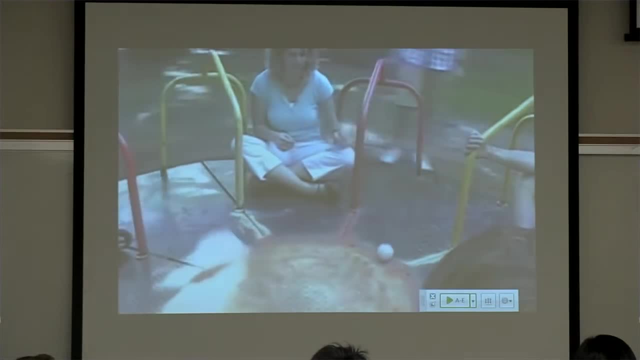 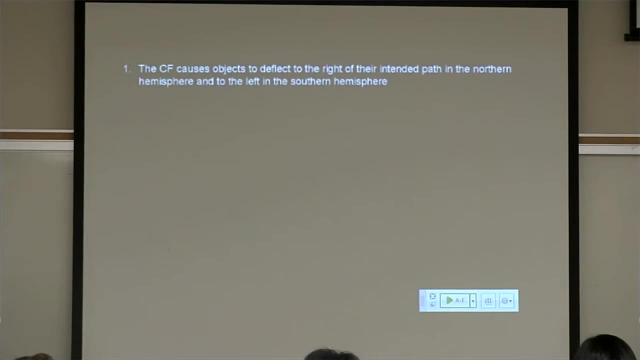 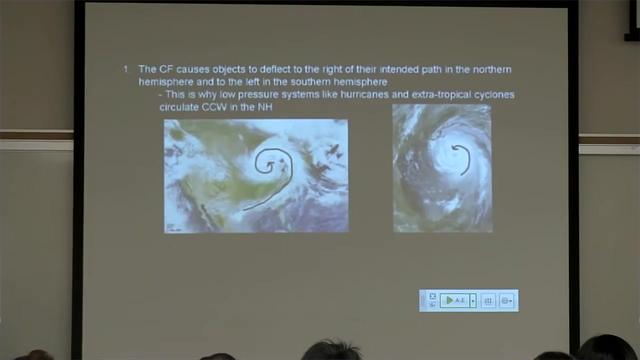 Some important facts about Coriolis force. First, the Coriolis force causes objects to deflect to the right of their acute attack in the northern hemisphere and to the left in the southern hemisphere. This is why low-pressure systems like hurricanes and exotropical cyclones circulate counterclockwise in the northern hemisphere. 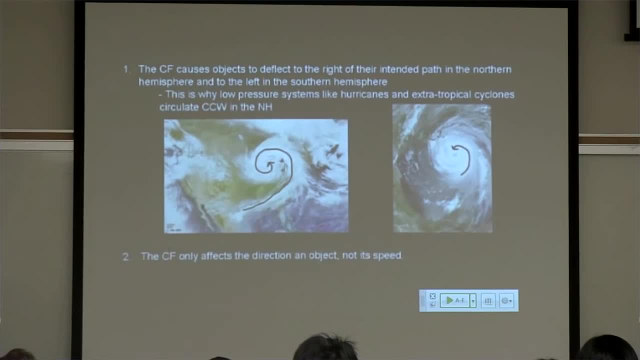 Second, the Coriolis force affects the direction of an object, not its speed. Third, the strength of the deflection. The strength of the deflection is proportionate to the speed. For example, the faster an airplane flies, the more the pilot must adjust the flight track to account for the Coriolis force. 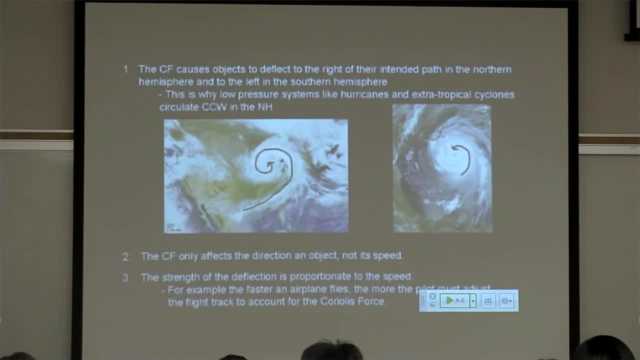 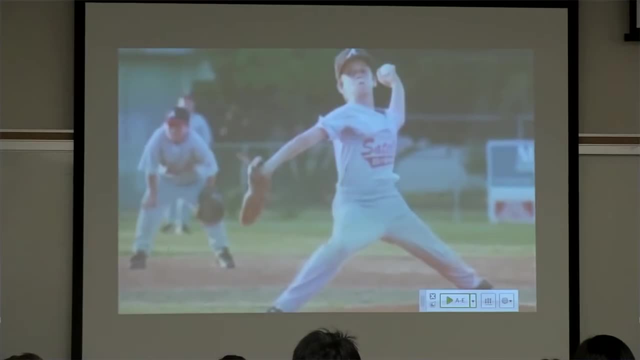 And finally, the Coriolis force is zero at the equator and maximum at the poles. To leave you with an interesting fact: the effects of the rotation of the earth are negligible at very small scales. For example, if a pitcher were to throw a pitch at Wrigley Field to home plate at 100 miles an hour. 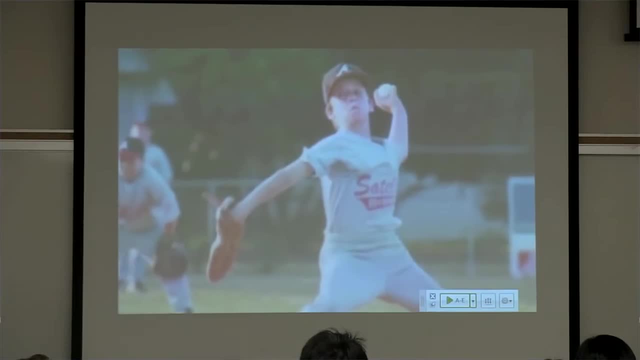 the deflection of the path of the ball is very small, only about 900 microns, which is about 0.9 millimeters, or about the thickness of your fingernail. However, for an intercontinental ballistic missile, if shot a few thousand miles at 1,000 miles per hour, 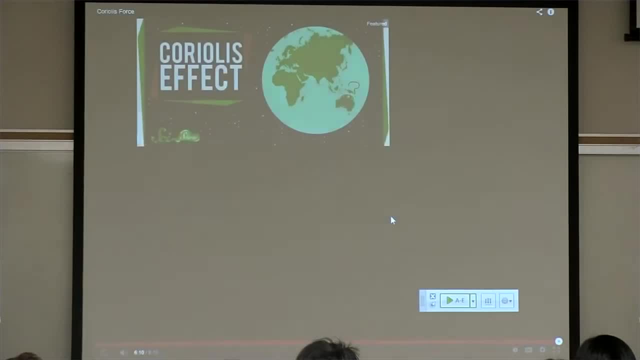 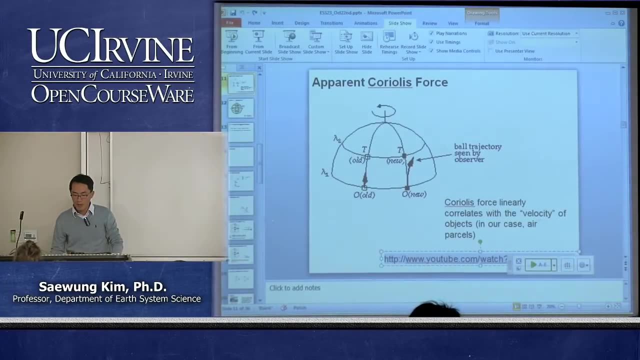 the deflection is hundreds of miles. So that's the basic summary of the Coriolis force. So how many of you actually heard about the Coriolis force before? Four, Maybe about one-third, So this is now a really familiar concept. 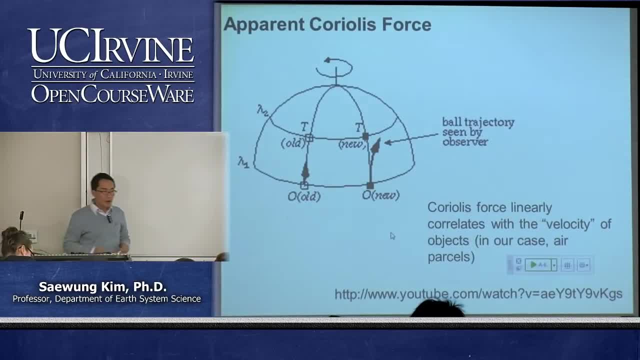 So basically, the bottom line is that the air motion is triggered by this pressure gradient from high pressure to low pressure system. But once it starts to move, then, because the earth is rotating, it is affected by the earth's rotation, And then we call that force as Coriolis force. 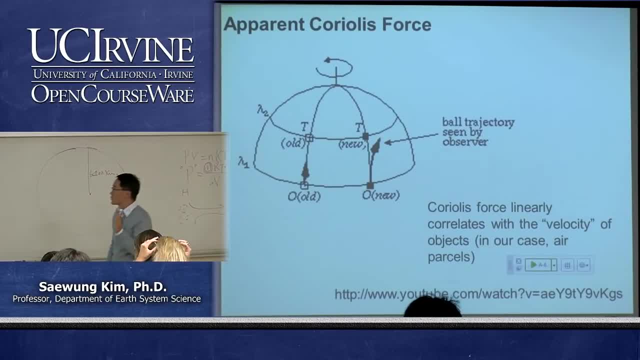 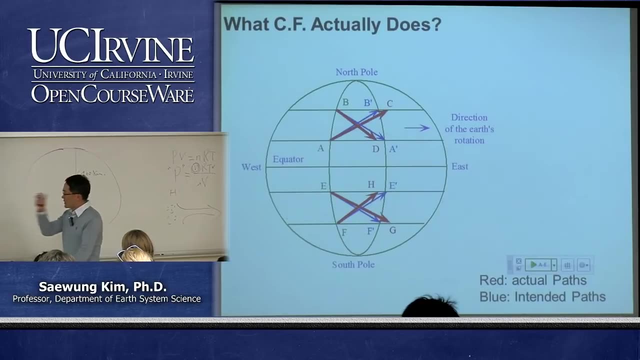 So basically, as the person on that video explained, the Coriolis force is always exerted to the right-hand side in northern hemisphere and then left-hand side in southern hemisphere. That's all you need to remember, And then so this is kind of a summary again. 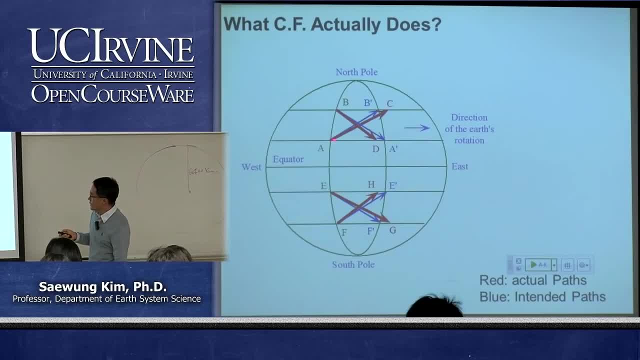 So from northern hemisphere. if a pressure gradient line is dictated, air motion from this point A to point B. here because of the earth's rotation it will be diverted a little bit towards the right-hand side again. And then the same thing from here to here. 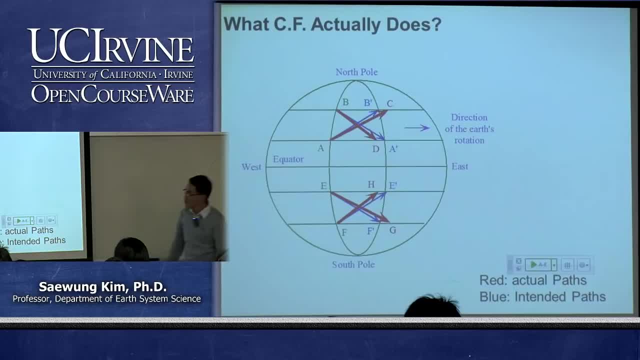 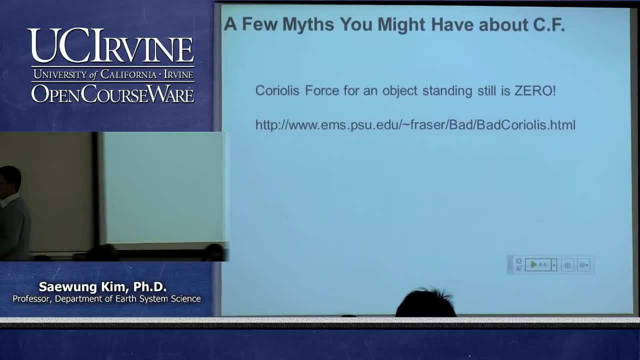 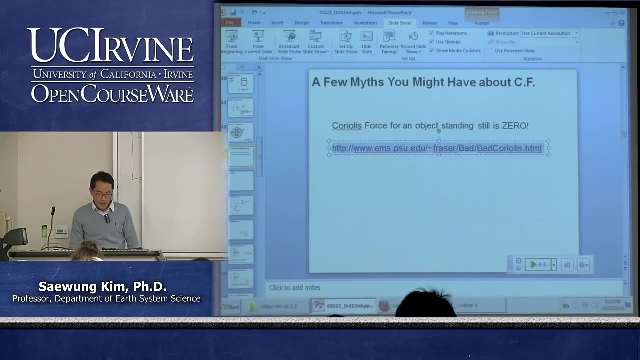 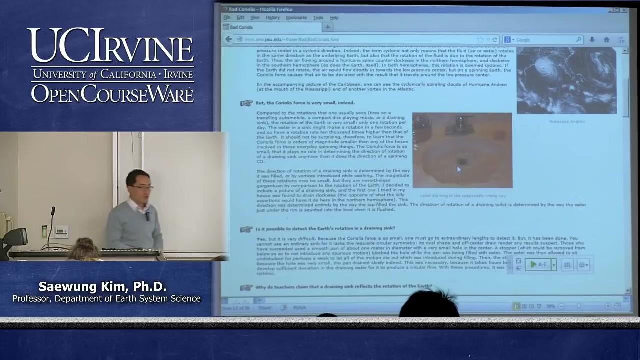 it is also diverted to the right-hand side due to earth's rotation. okay, So among of you that already heard about Coriolis force, and then have you guys heard about this rotation of the drain? The water is circulating here. It's governed by the Coriolis force. 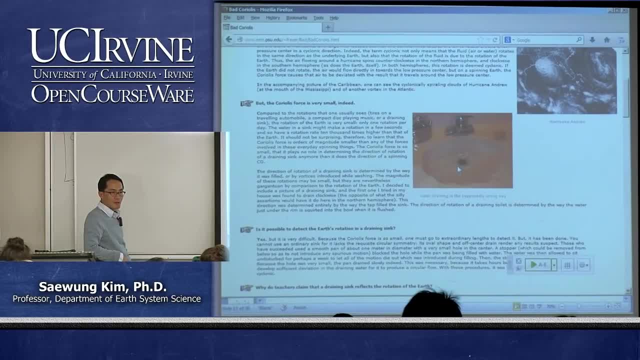 How many of you actually heard that theory? Most of you. That's wrong. That's bogus theory. And then, as the video explained, that Coriolis force only affected on large-scale phenomenon, not this kind of a small-scale phenomenon. okay, 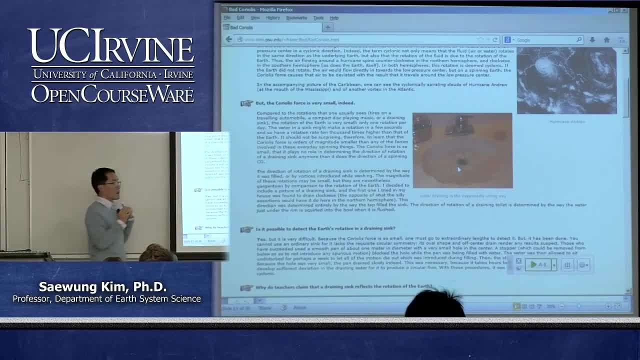 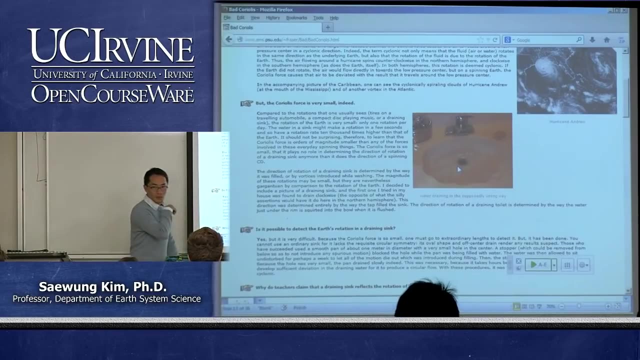 So that's the only thing that only a force that affects on the large-scale phenomenon like high-pressure system or low-pressure system. It's at least couple of hundred kilometer motion of the air or whatever, but not this kind of a small-scale problem. 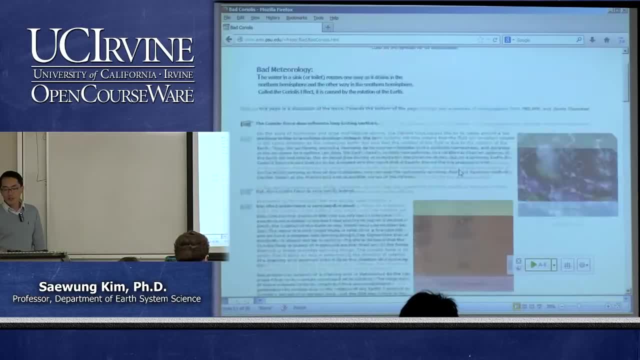 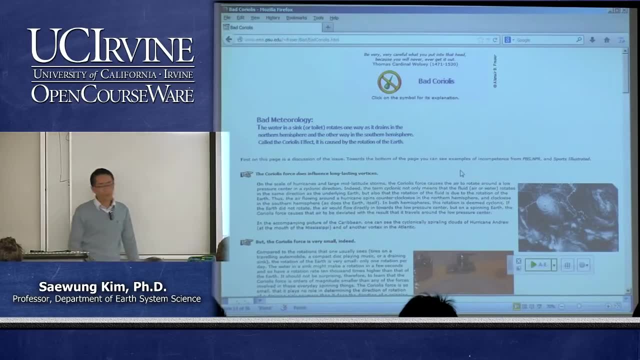 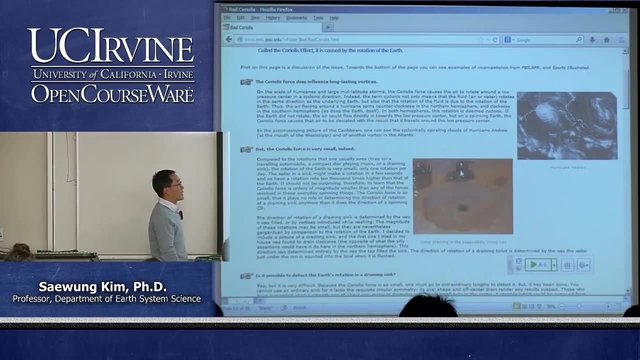 So if you want to know further about this, then you can just read this website. This is kind of a website written by a meteorology professor at Penn State University and then he attacked couple of the misconceptions, of the scientific kind of misconceptions. 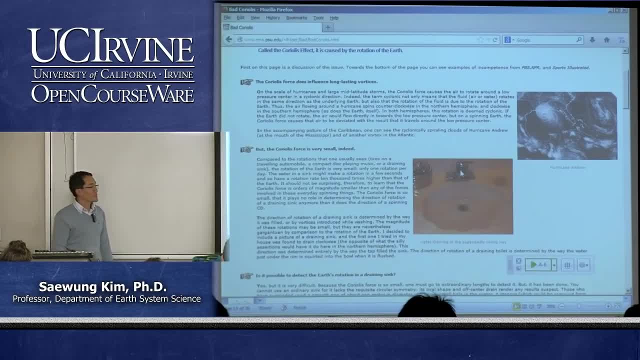 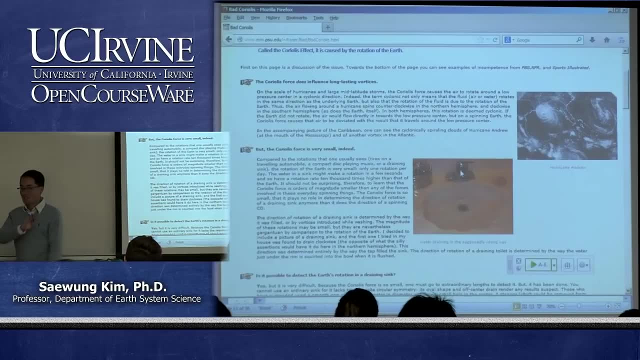 among the public out there. It's kind of surprising actually. I even thought, even in South Korea, I even thought that this is affected by the Coriolis force. but that's not right, That's simply wrong. so wrong about it. 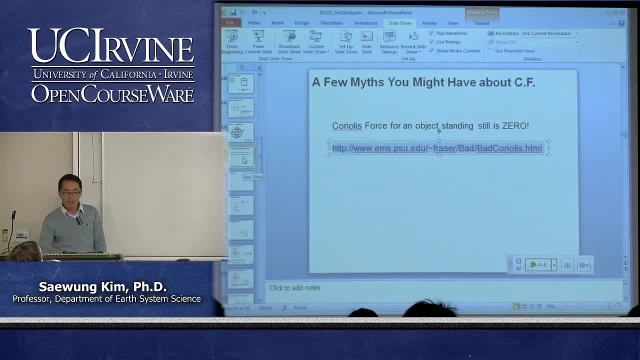 So that's one thing you need to remember. And then the other thing is that Coriolis force is only start to affect on the motion once motion gets started. So if some object is standing still, there's no Coriolis force is affected on there. 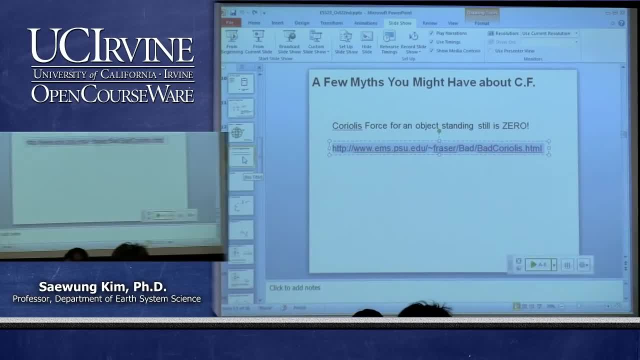 So we need some mechanism actually to initiate air motion- In this case pressure gradient, Initiate the air motion. then, once it is air motion initiated and then it is kind of a large-scale, then it is affected by the Coriolis force. 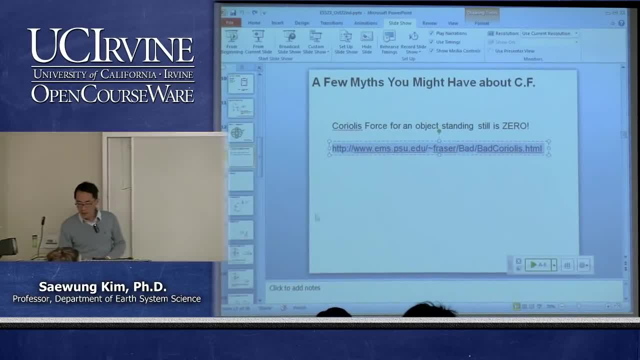 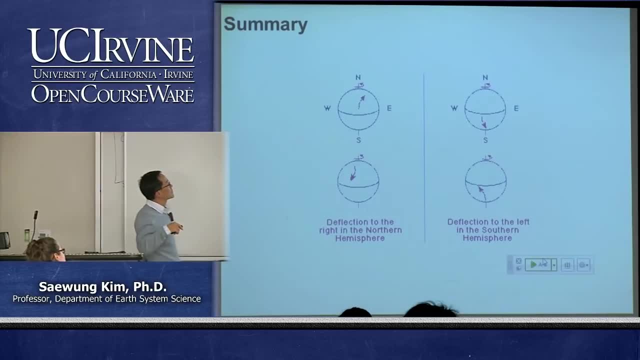 So that's the thing you need to remember for the Coriolis force. So let's go ahead Again. summary: So because of the rotation, the northern hemisphere going right, right and then left and left, okay, So let's put together this pressure gradient. 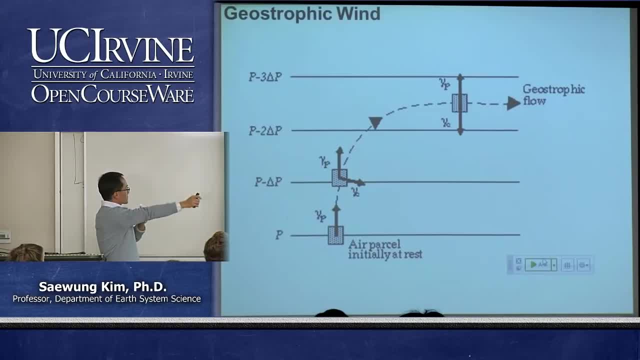 and then Coriolis force, all together, right. So basically, let's assume this is high-pressure system and then, as you can see, the pressure gets lower. This line. so this is the same pressure. This is the line indicating the same pressure. 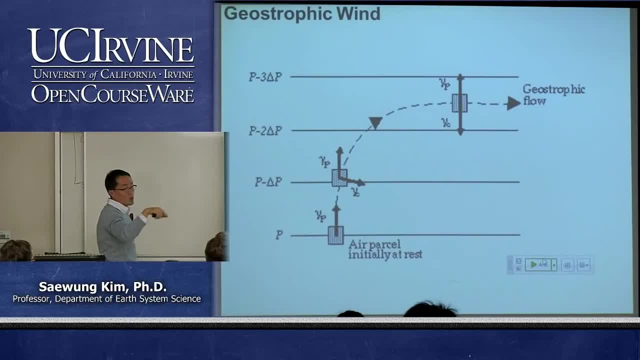 So pressure out here is the high pressure towards the low pressure, right? So because of this pressure gradient force, the air motion is initiated right here. Then, once it starts, then Coriolis force will be affected. right Then either air will be moved to your right-hand side. 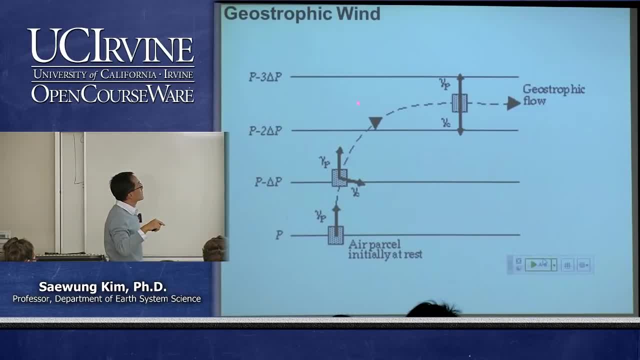 if we assume this is northern hemisphere, Then finally it just balance between the pressure gradient and Coriolis force and then it will just follow this pressure gradient line right. So we call this air motion as a geostrophic wind set right here. 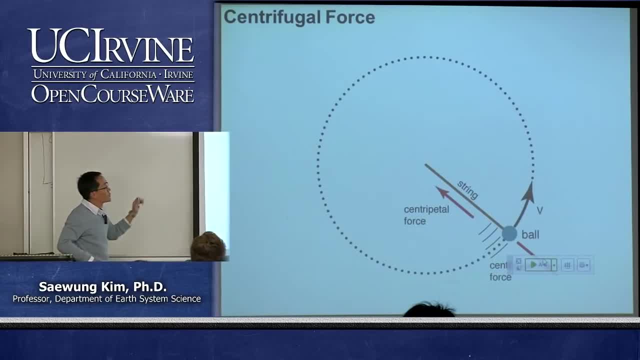 But, as you see, as you saw that video clip, so Earth is rotating and then Earth is round. So once this, usually this pressure gradient line is the round shape. So another force we need to, another two forces we need to consider. 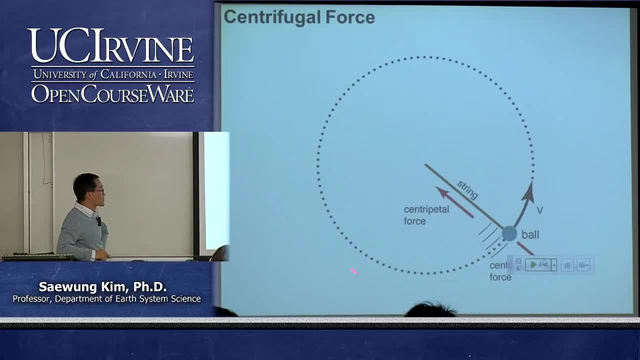 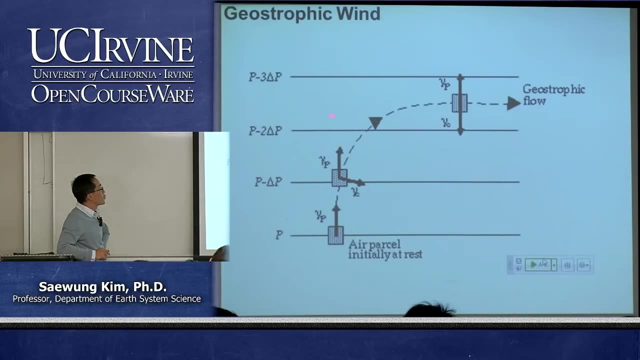 once it is making the rotation motion like this centripetal force and centrifugal force, but those two forces also balance each other, So it just makes this circular motion. So this kind of a wind, a geostrophic wind, is going to be happening. 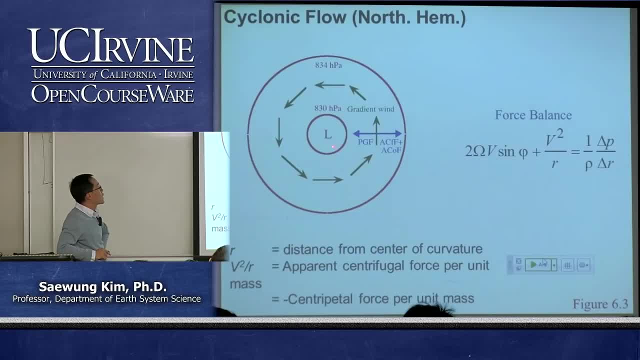 if Earth is flat, but Earth is round. now the high pressure and low pressure system are making this circular motion. So if we assume this is the center of the low pressure system, then obviously the high pressure is going to be outside of this pressure system. 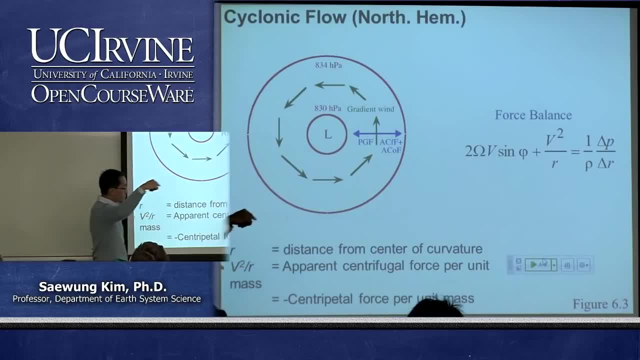 So the pressure gradient initiates air motion towards from high pressure to low pressure side, And then, if it is northern hemisphere, what's going to happen is that it's going to be turning right like this and then making this geostrophic wind which is following pressure gradient line. 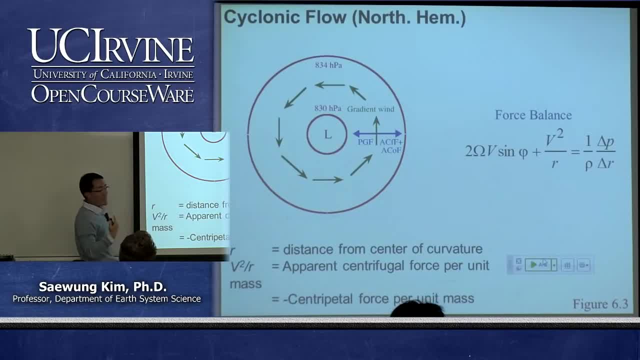 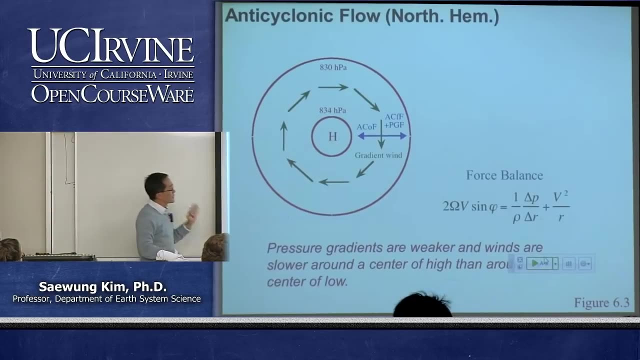 like this: If you are math geek, you can solve this equation to actually visualize this thing. Probably not many of you guys are math geeks, so ignore this equation, alright. So this is a low pressure system case and then a high pressure system case. 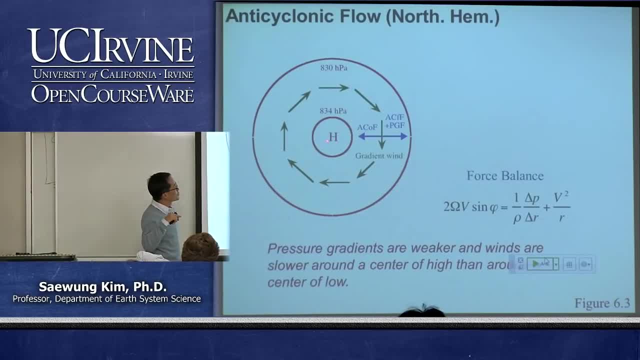 that air is going to be moving from high pressure to the low pressure, Then, when air motion gets initiated, and then air motion is going to be affected by Coriolis force and then it will turn right and then making this circular motion Right. So this is geostrophic wind. 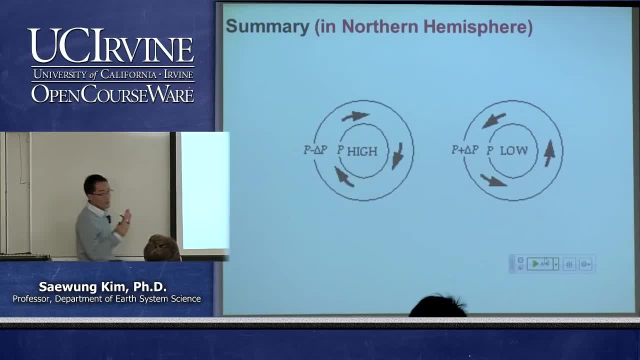 Okay. So again, this is summary. It's turning clockwise. Is that clockwise? Yes, clockwise in high pressure system and then counterclockwise in low pressure system in the northern hemisphere. It's going to be exact opposite in southern hemisphere, right? 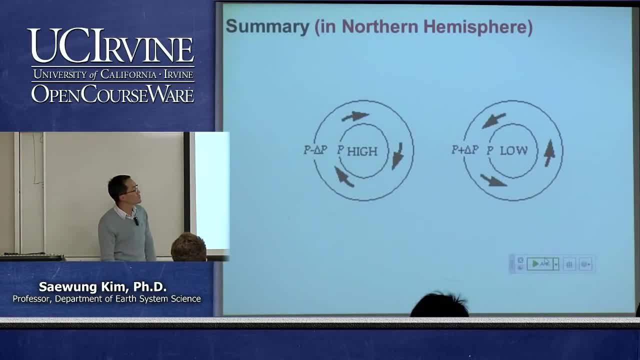 And then this is air motion that we assume that there's no friction. So air motion that is happening in the high altitude, like 5 km above the surface or 10 km above the surface, there will be no friction between the air masses and then air masses. 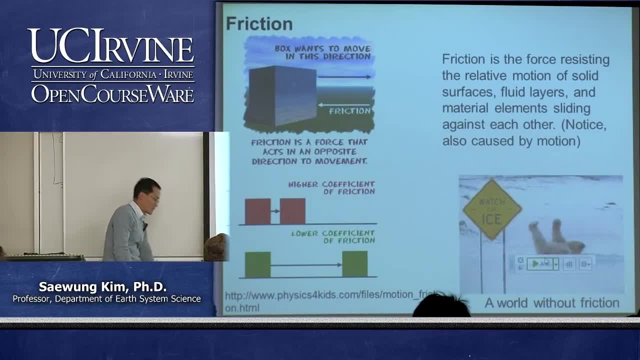 But if you assume the air motion in the surface, then there's significant friction between air and then land surface. So basically, friction is that force. if you want to move this block to this side, and then friction is going to affect it to the exact opposite direction. 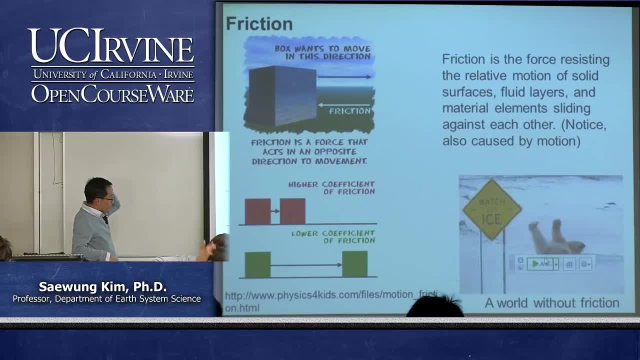 of the actual object is moving Right. So that's basically the reason we can walk on the surface. We use the friction actually. then we can walk on the surface Right, And then if there's no surface, and then we cannot walk, so even the polar bear. 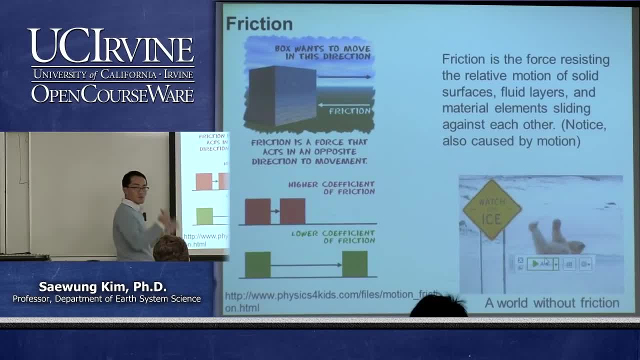 is going to be just sliding away here and there If there's no friction. so friction is kind of an important thing to maintain our life. And then if we use the friction to stop the car, so brake system is pretty much the thing that we use, the friction. 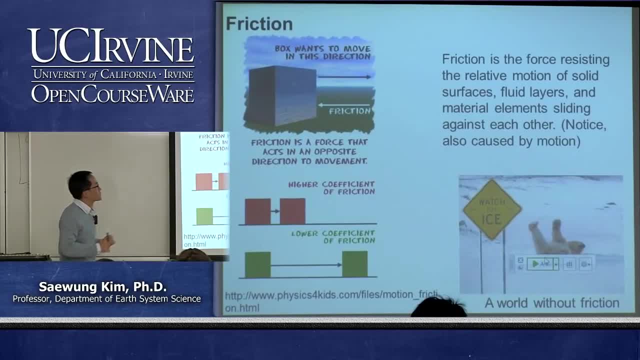 and then it just stops the wheel motion of the car. So friction is an important thing. We often forget about the friction, but friction is happening all the time, Even we just walk around the campus or anywhere, Right, So it depends on the surface. 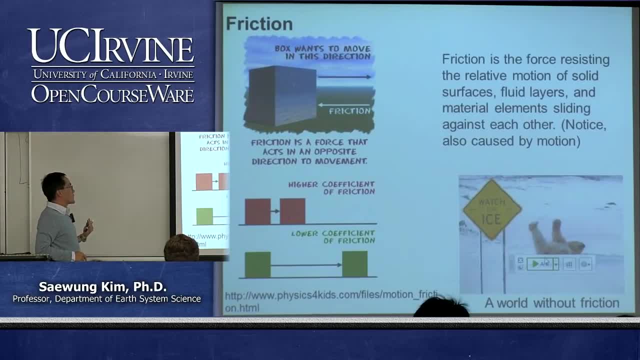 There's high coefficient of friction. That means that so if you just exert the same amount of the force to the object, if your surface has higher efficient of the friction, then actually you ended up moving shorter distance than the surface has lower coefficient of friction. 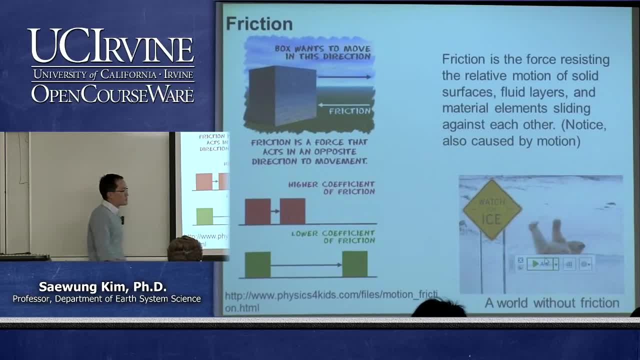 So that's kind of a way to quantify that friction. But what only you need to remember from this class is that there's always friction between air and the surface, And then that's going to be affecting air motion above the surface, Right? So this is the summary. 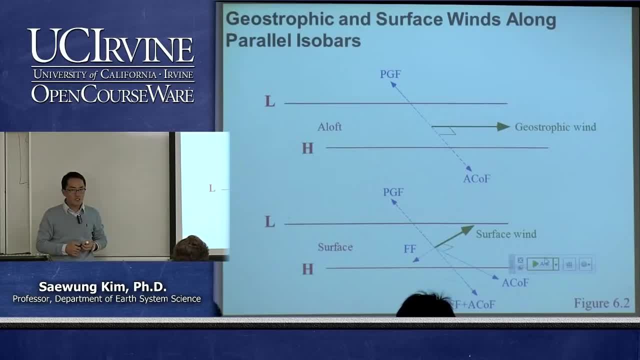 of the friction force that affects on the air motion above the ground. So geostrophic wind is right here. so geostrophic wind is the wind that is happening up in the air, maybe one kilometer above the surface, two kilometer above the surface. 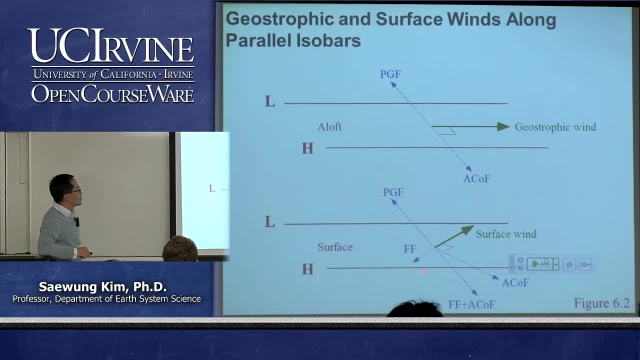 But on the very surface, due to this friction force, it is not really parallel to this pressure gradient line. Rather it is moving a little bit towards the low pressure side. So air motion is going to be moving towards the low pressure side. 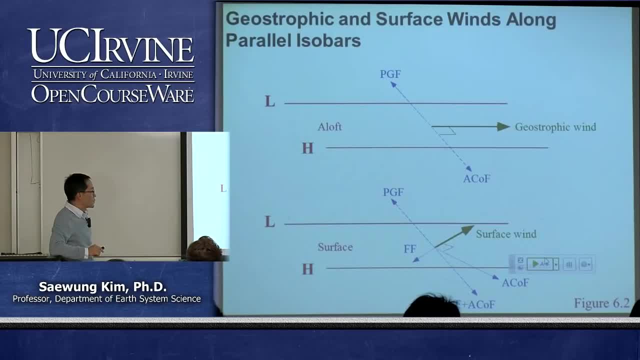 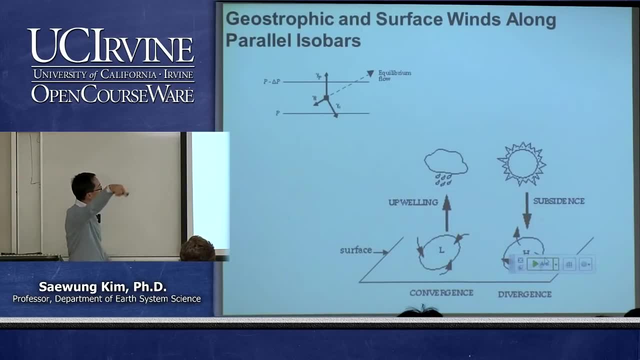 If you can see the balance between a pressure gradient force and then Coriolis force and then friction right here. So this is another summary that on the surface it's going to be moving towards to the low pressure side. And then, if you take a look, 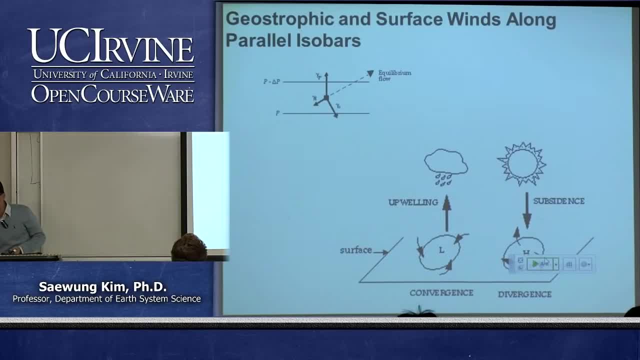 at the high pressure and low pressure system, then this is actually blocking this figure. Then, due to friction on the surface, air is moving towards the low pressure side. So if we have a low pressure system right here, air is going to be. 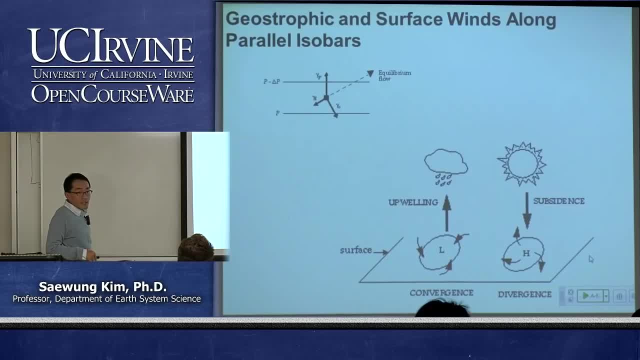 on the surface, air is going to be moving towards the low pressure center right, And then what's going to be happening is that if air- this is all about the air molecule- is moving towards the specific point like that, then there is going to be more air. 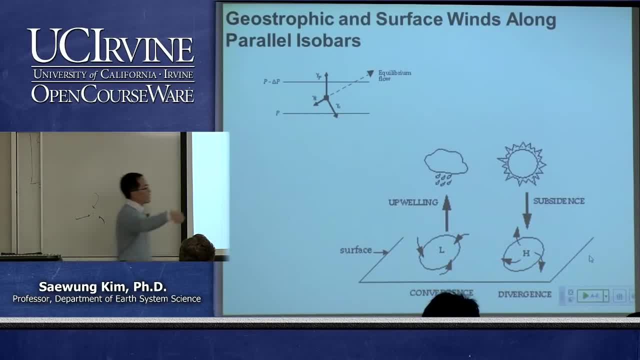 accumulating on the surface than air is going to be moving up from the surface so that more air can be rolling into the low pressure center right. So in the low pressure there will be a welling air motion. It's going to be happening. 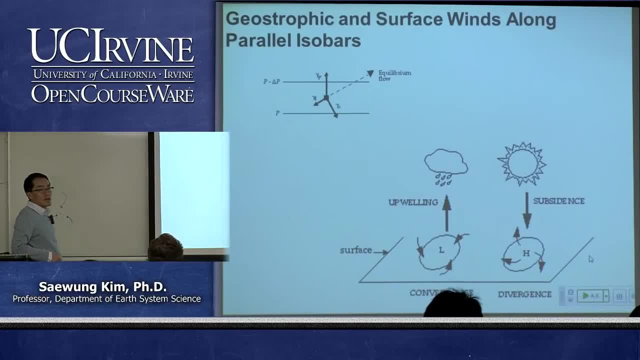 and then what's going to be happening in the welling of the atmosphere is that up there temperature is lower, right, Then condensation is happening, Then you can expect cloud formation and then usually it's associated with the rain, things like that. 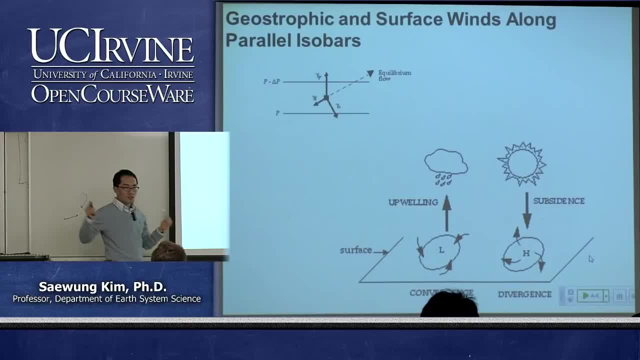 So that's why, whenever the low pressure system is rolling in to the, even in Southern California, there's a cloudy day and then rain is associated with it because of this welling motion, And then, in high pressure system, air is going to be moving out. 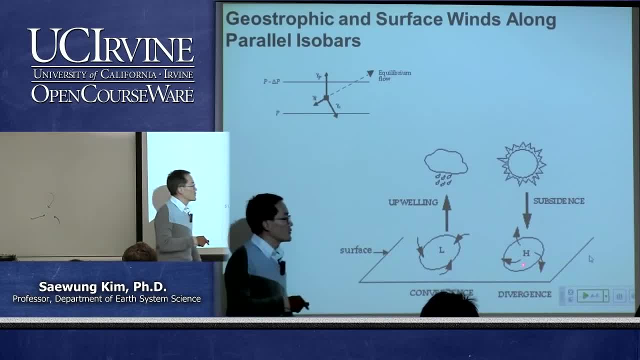 from the high pressure system from the surface right, Then some air should be fill this void, because air is moving out from this high pressure center. So what's going to be happening is that air is coming from the top upper atmosphere. 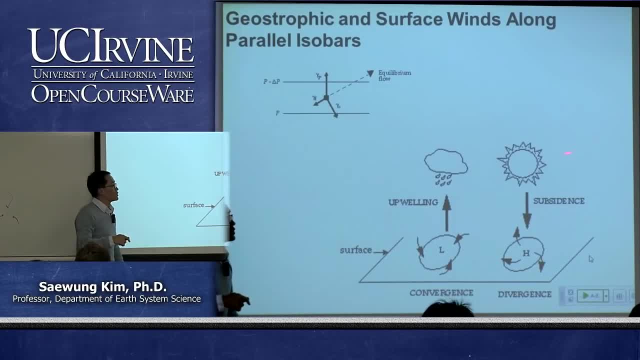 and then subsidence is happening. So that's why we usually observe the clear day in the high pressure system, right? So this is high pressure system on the surface and then low pressure system on the surface, And then. so difference between geostrategic wind. 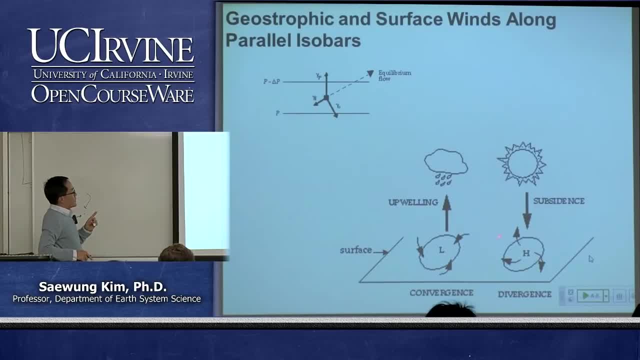 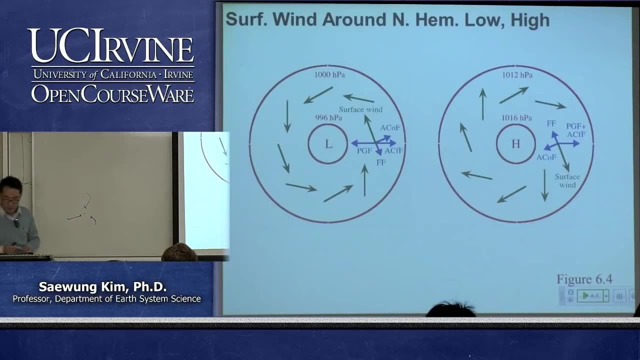 and then surface wind. is that, due to friction, air is moving into the low pressure system, Then moving out from the high pressure system. Okay, This is not working. Here we go. So again, this is summary that a little bit towards the low pressure side. 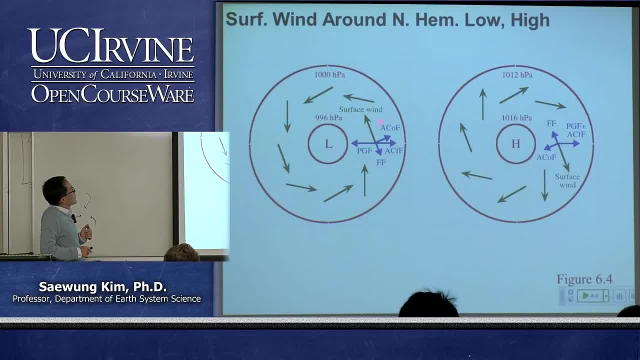 and then this is a little bit towards the low pressure side. So air is going to be coming into the low pressure side center and then air is moving out from the high pressure center. But if you take a look at the direction of the arrow, 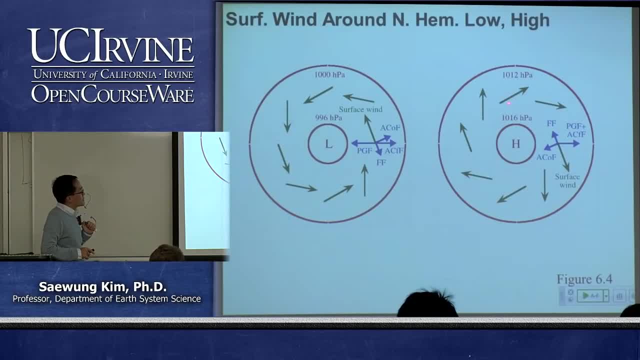 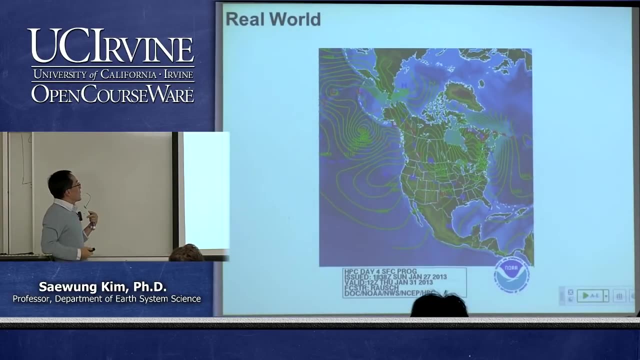 again just the same: that high pressure system- air is rotating clockwise, and then a low pressure system- air is rotating counterclockwise. Okay, So this is real world example that usually there's a, you know, multiple high pressure and low pressure system. Usually the low pressure system over the ocean associated with the rain because of the it contains a lot of humidity in there and the low pressure system is associated with the motion of the air. So maybe twice a year we have a rain in Southern California. 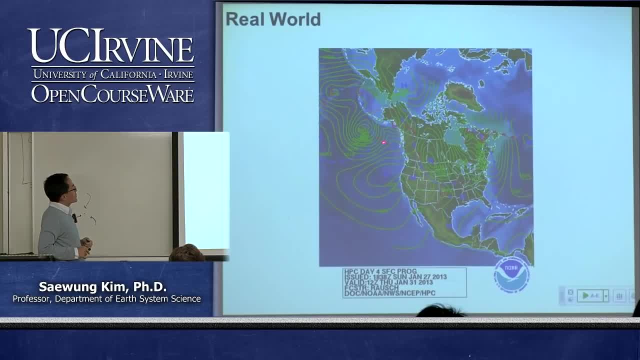 Most of the cases this low pressure system over the Alaska, especially during the wintertime, rolling into the Southern California that actually caused some rain event in Southern California And then this low pressure system is expanding, usually towards the in the Pacific Northwest region. 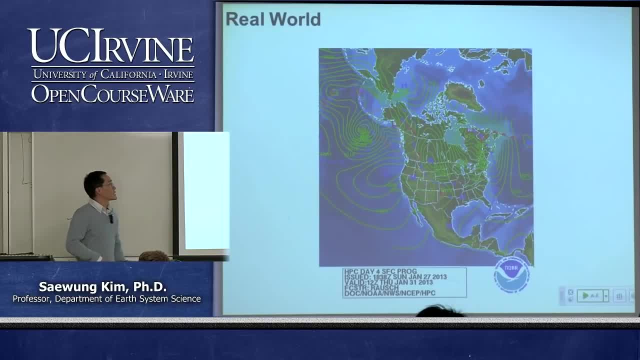 like Seattle and Oregon place like that. So that's why they have rain all the time from October to the April, because of this low pressure system out here in Alaska, Right, So? so if you understand at least low pressure, how surface low pressure? 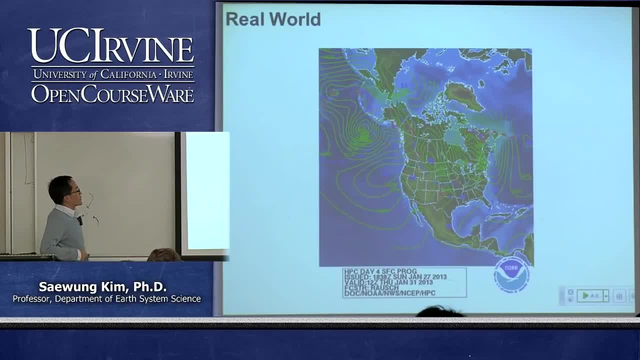 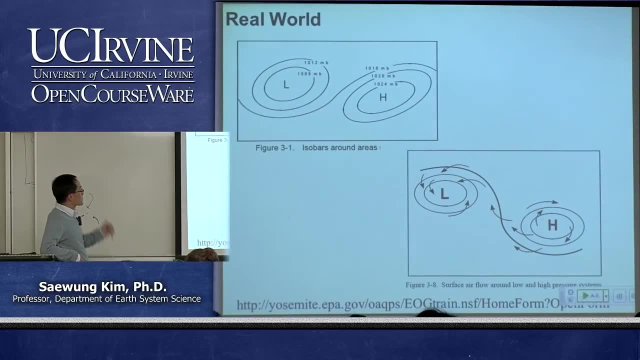 and then high pressure system working, then you can understand pretty much what's going on in terms of green schematic things in the weather system over the United States. So so again, this is another kind of photo- show that how air is moving in the high pressure system. 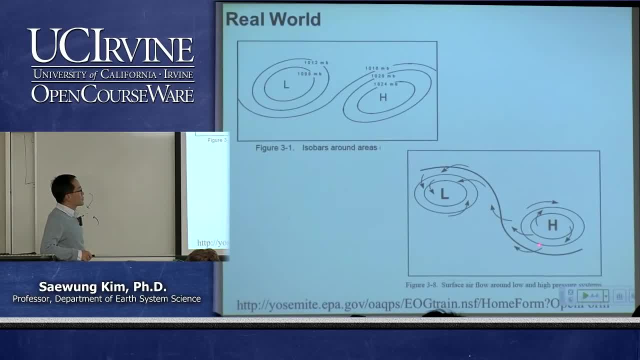 and the low pressure system over the surface. So air is going to be moving out from the high pressure system and then going into the low pressure system. So what I want to expect you guys is that if you just see this photo by itself, then you can just draw some arrow. 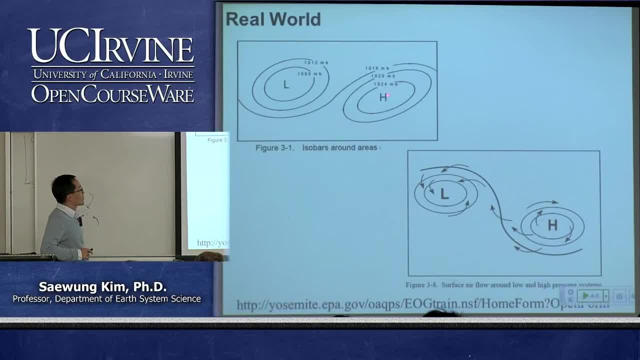 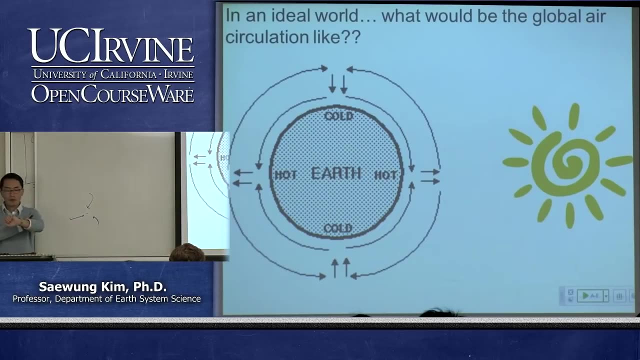 of the air motion, that air is going to be coming out from the high pressure system, And then you should know that direction of the air motion, that caused by the Coriolis force, Right? So that's it, And then. so let's take a look at now. 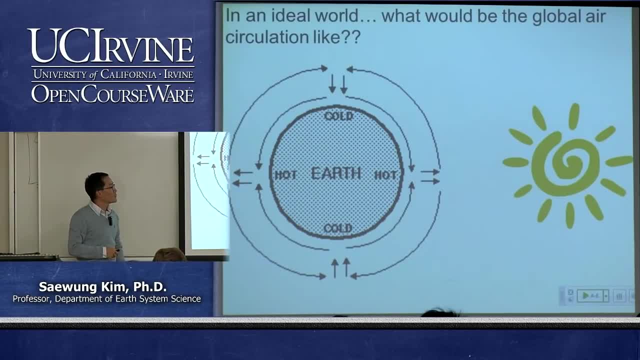 a little bit of a three-dimensional motion of the air, Kind of a. we talked about the horizontal air motions, Now let's discuss about some vertical air motion. So let's assume Earth is just like this, and then Sun is right there And then it is just heating up. 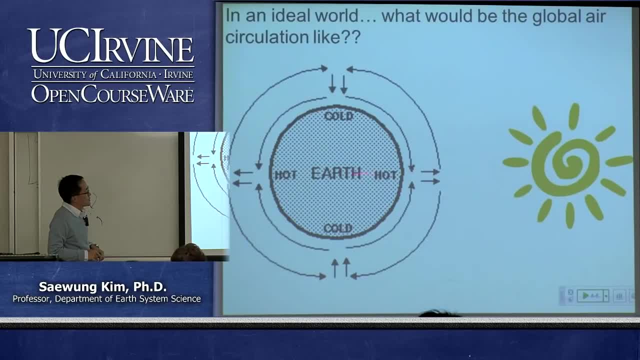 in the middle, Then equator region is going to be hotter than the polar region, right? Then what's going to be happening is that there's a convection going on because this is hotter, Air is lighter, and then it's going to be going up. 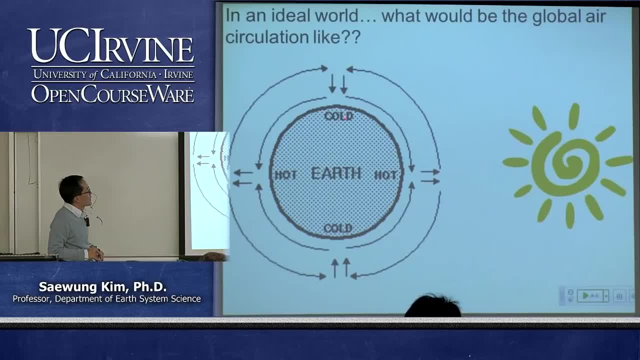 And then some other air in the polar region, because it's cold, will be filling in this space. that because air is moved from the surface to the above, And then that caused this circular motion, right? So basically this is the initial thought about the air motion. 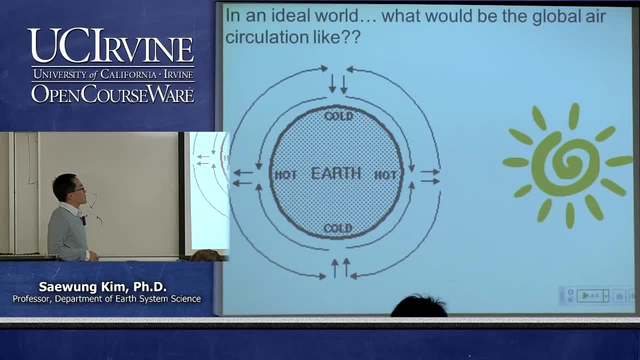 And then we call it Hadley cell. So the scientist's name called Hadley first developed this concept. So this is going to be the air motion. So this is the Hadley cell model. So in the equator air is moving up. 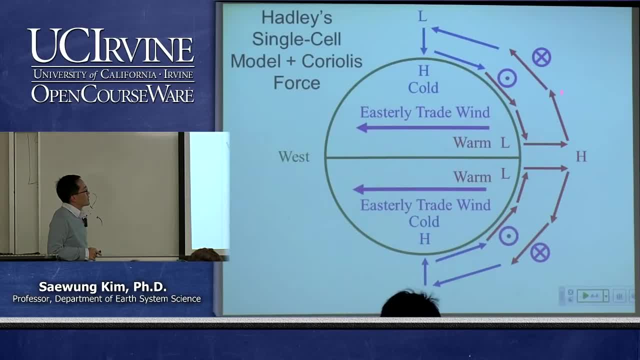 And then this in the upper atmosphere. then air is moving towards the polar region like that, But due to Coriolis force right, this air motion from this equator to the polar region is going to be to the upper atmosphere And then your right hand side. 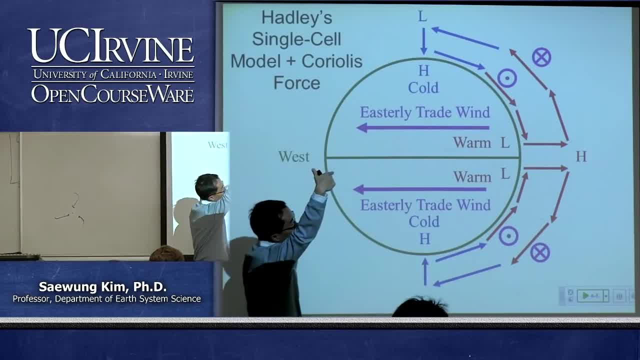 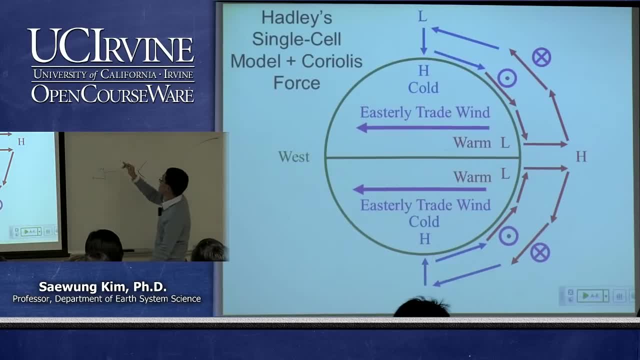 that's why this air motion is the backside of the arrowhead right, So the arrow right. So if you assume arrow just like that, so that's basically arrow is kind of from here to the screen, right. So that's why. 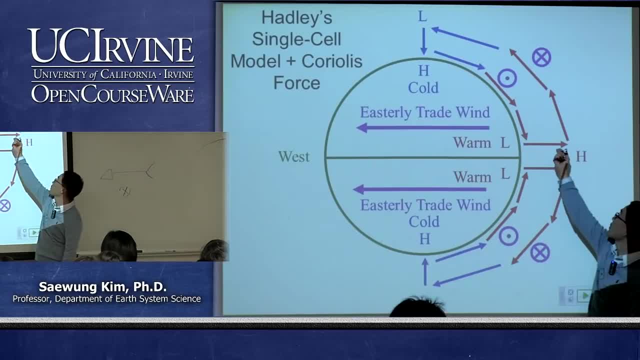 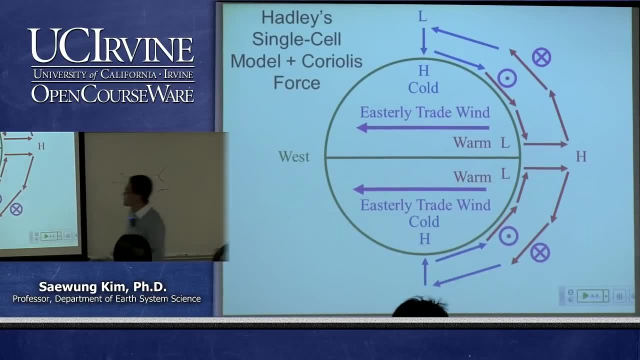 we just rotate this thing like this, And then if air motion is coming from this screen to your side, then it just looks like this: right? So due to Coriolis force, the air motion from equator to the polar region is going to be: 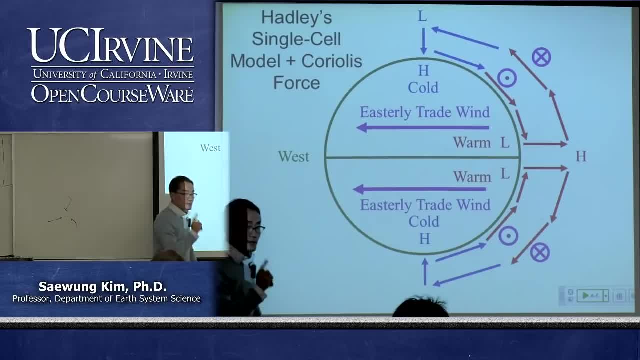 moving towards your right hand side. So this is what actually so the origin of the jet stream in the upper atmosphere. Very fast, air is moving from. let's see, this is the where is the east and west. So this is the west to east motion, right. 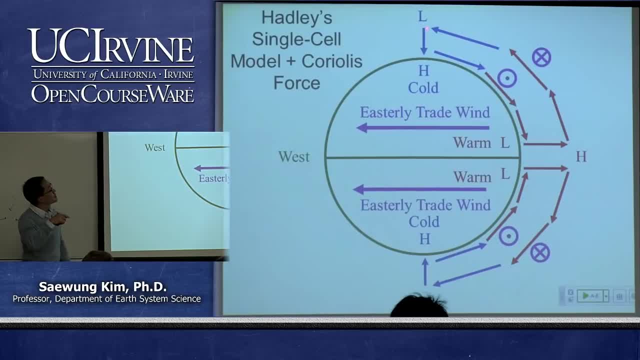 And then on the surface, because of the sinking air in the polar region moving towards the polar, to the equator, and then air is also affected by the Coriolis force, then it's going to be moving out from the screen, right, Right. 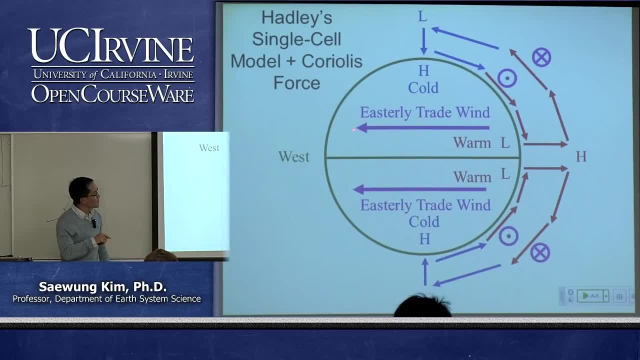 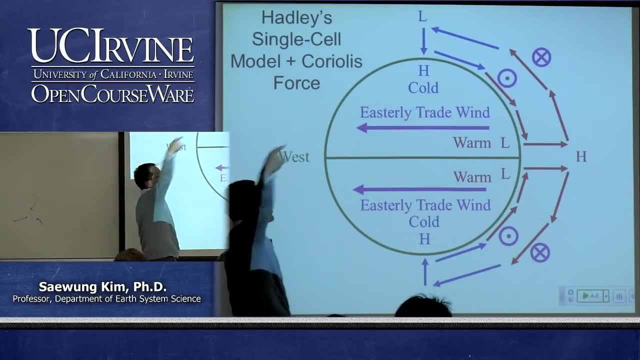 So on the surface there's an easterly wind there, and then on the top of the atmosphere there will be a westerly wind. that is going through the screen right, At least in the northern atmosphere. The southern atmosphere is. everything is a positive. 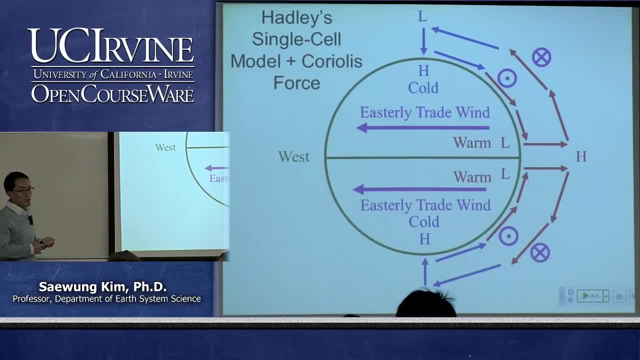 Okay, So this is basically hardly model of the air motion of the Earth, right? Confusing Too easy. You guys looking very bored, Get bored by that. Maybe you guys already heard about this thing. I don't care about this thing. 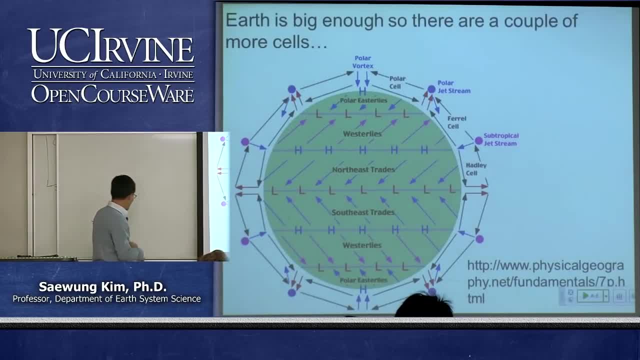 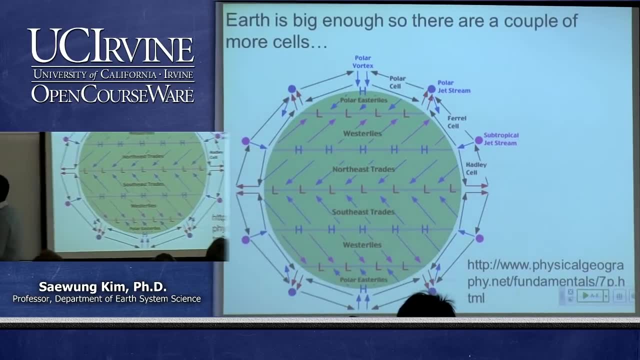 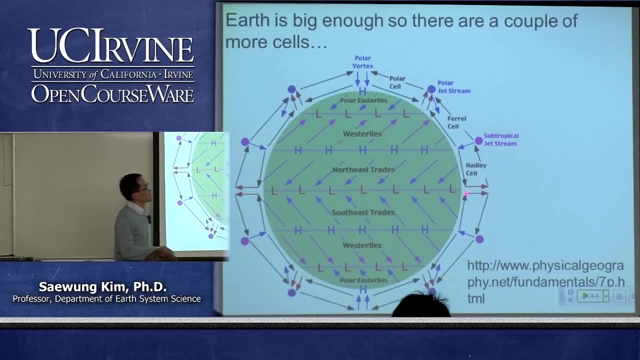 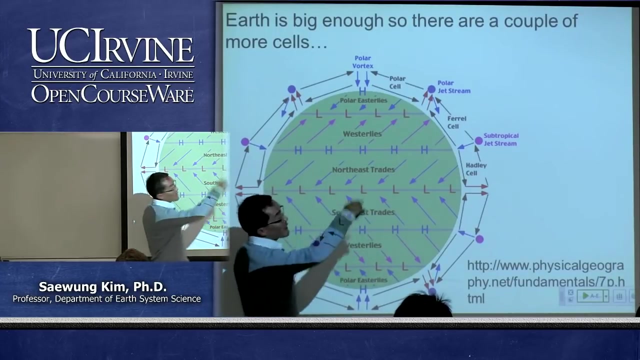 or something. But let's make it a little bit complicated because you guys look very bored by this simple model. But Earth is big, right? So Earth is so big so this hardly cell that initiated in the equator cannot actually move all the way out. 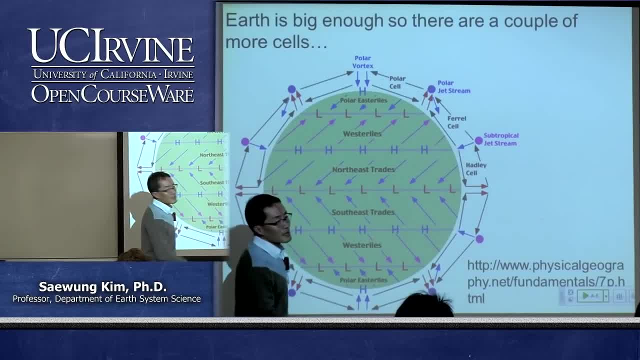 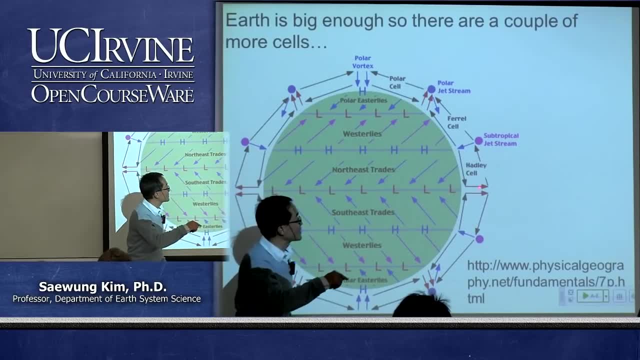 to the polar region. right, It is just making one cell in the one-third of the Earth's surface in the northern hemisphere. So basically this is hardly cell right here. that is, if it is small enough, Earth is small enough, then there will be one cell. 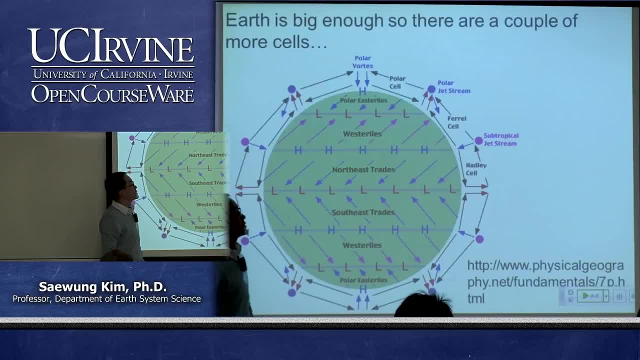 which is hardly cell who can happen, But Earth is so big. so one cell is happening here, then the other cell is sitting in the mid-latitude region and then there's another cell is going on here In the polar region. there's three cells in each hemisphere. 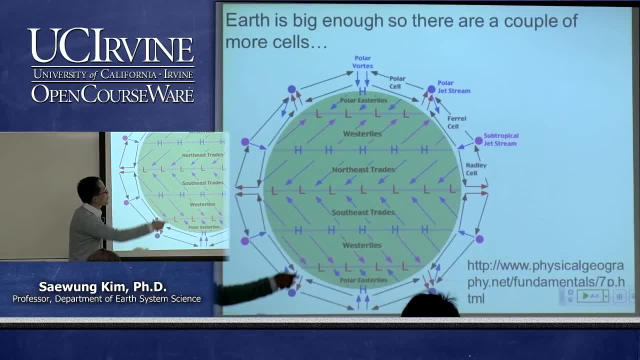 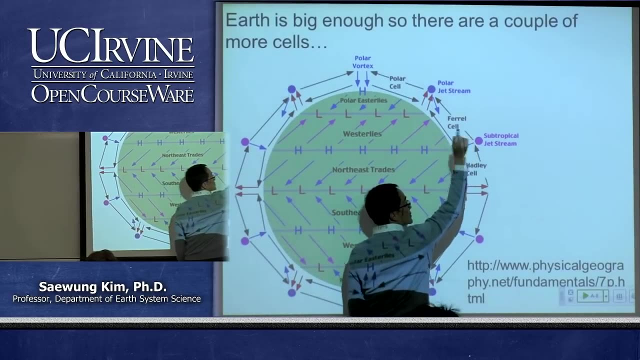 So overall there's six cells over the Earth. So we call it hardly cell which is near to the equator. So this cell actually makes this jet stream which is air is moving from to this side right, So from west to the east. 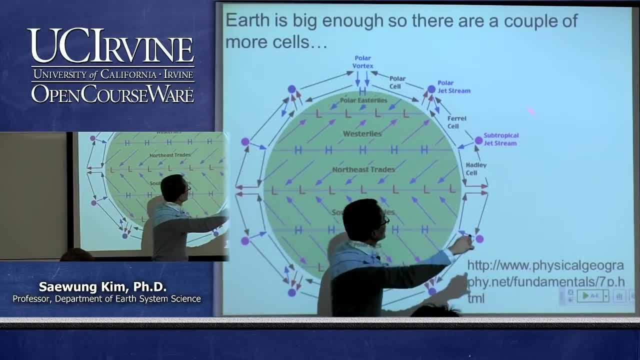 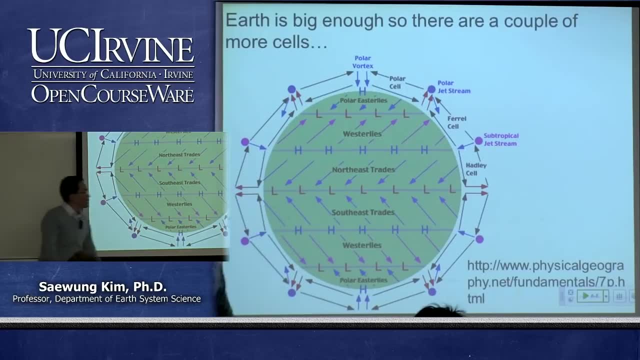 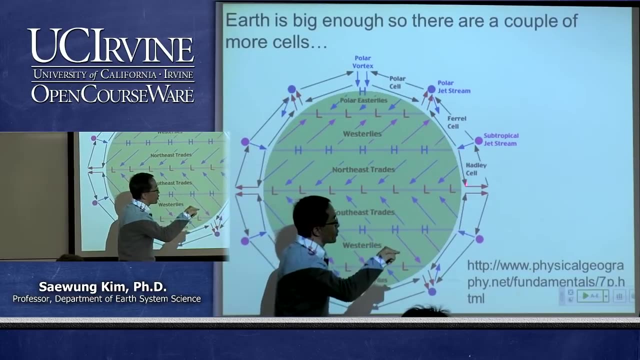 And that's the in the upper, in the upper troposphere, upper air. And then what this cell makes, the surface wind, is that because air is moving from higher latitude region to the lower latitude region, like this, and then, due to Coriolis force, air is going to be moving. 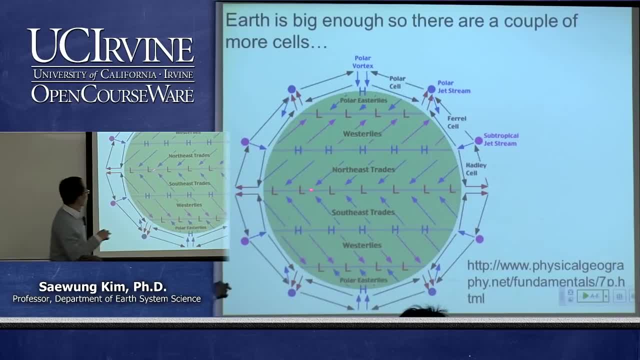 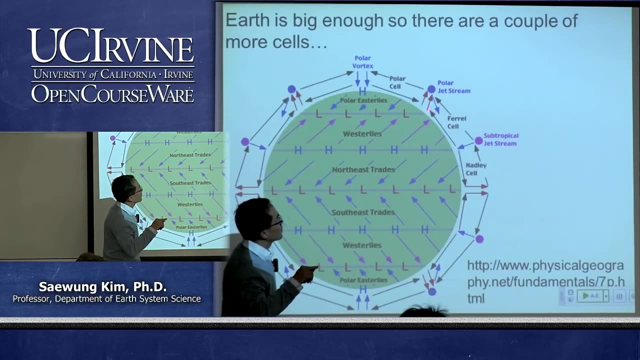 to your right hand side like this: Now, we call this wind as trade winds, right, And we call this the federal cell, which is because air is sinking right here and then air is going up, right up in this latitude region. So, and then this: 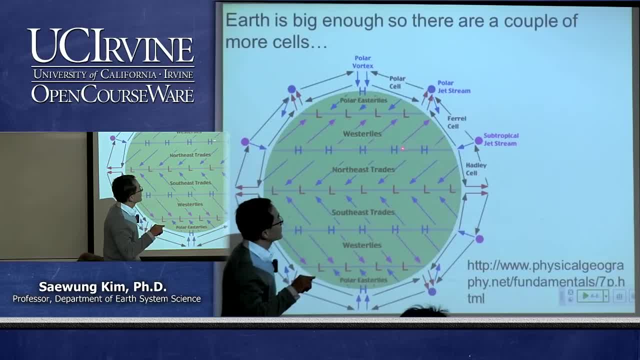 in this cell surface air is going to be moving from south to the north and then, due to Coriolis force, it will be bearing to your right hand side, and then again here there's another- jet stream is coming in the about 60 degree north and 60 degree south. 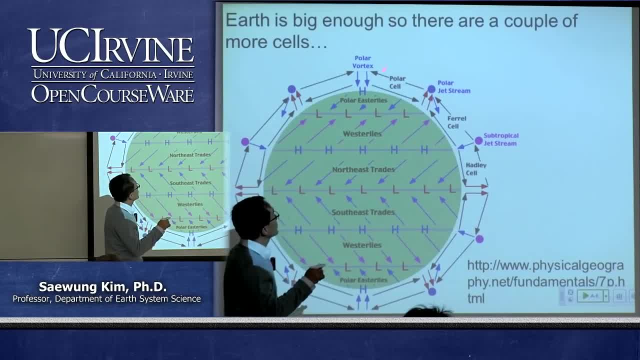 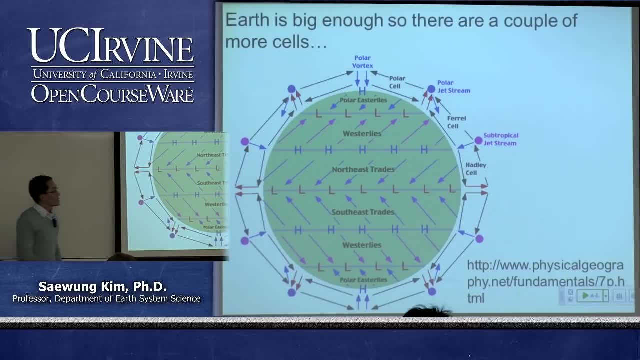 Okay, Then finally there's polar cell right here and then make another east wind. So this is overall wind distribution over the over the earth that is mainly caused by sun, is locating in the equator region. So obviously this is very conceptual question, conceptual model. 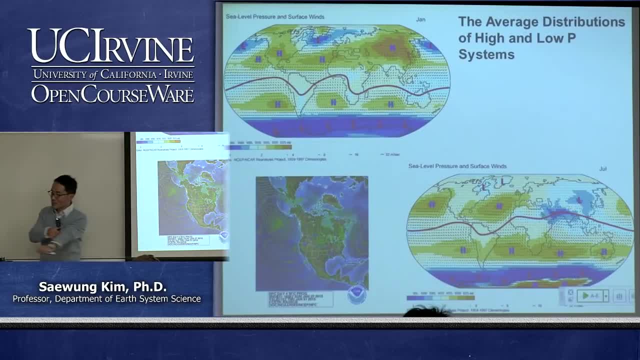 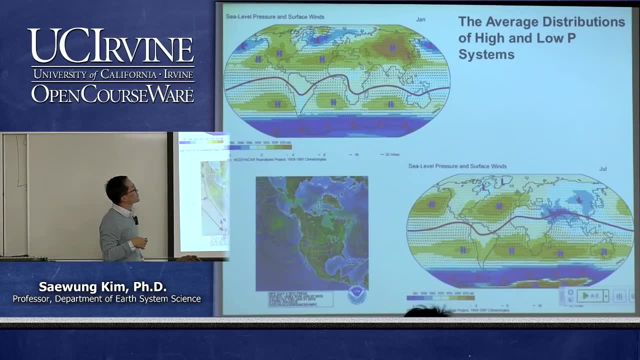 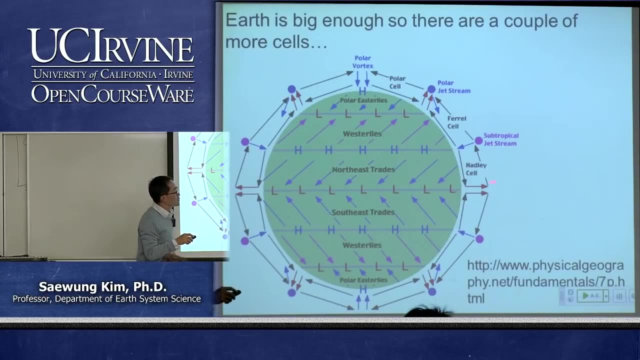 and then let's go to the real world example. So this is January, January pressure distribution. Let's, let's go back this thing again. So I didn't explain the low pressure and high pressure distribution here. So, because air is moving upward, so this is by definition. 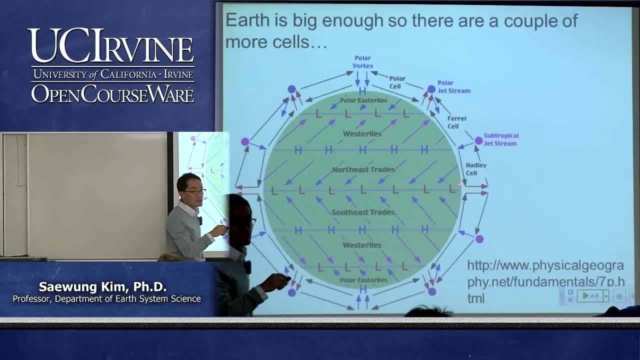 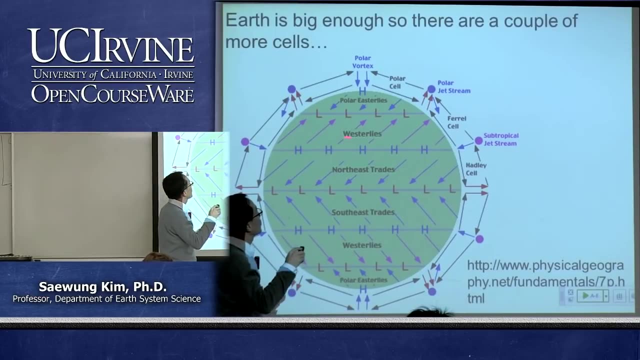 low pressure region right in the equator region. That's why over the equator there's rain all the time, because this permanent low pressure system sits in the equator region Okay, And then about 30 degree north what we call high pressure, permanent high pressure region. 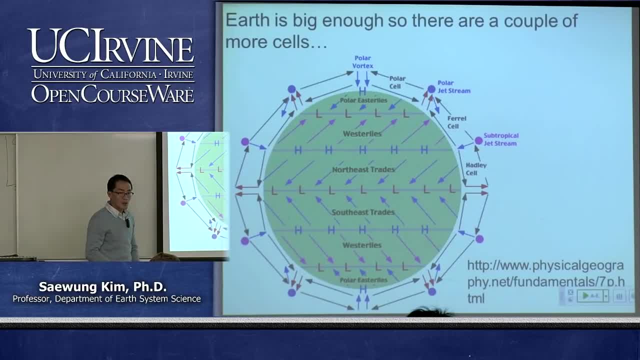 and then, because there's a sinking motion of the air exist right there. so there's a permanent high pressure system, usually located about 30 degree north or 30 degree south, either way, And then in the 60 degree, again there's- there's upward motion of the air. 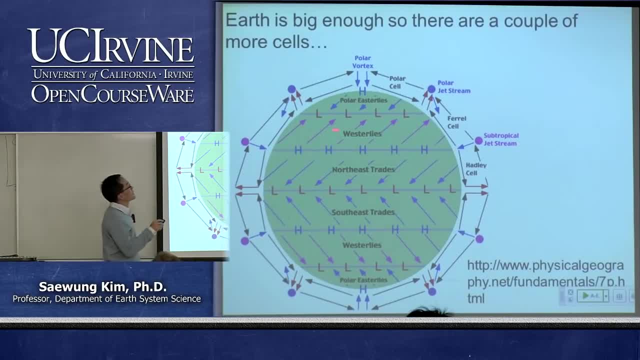 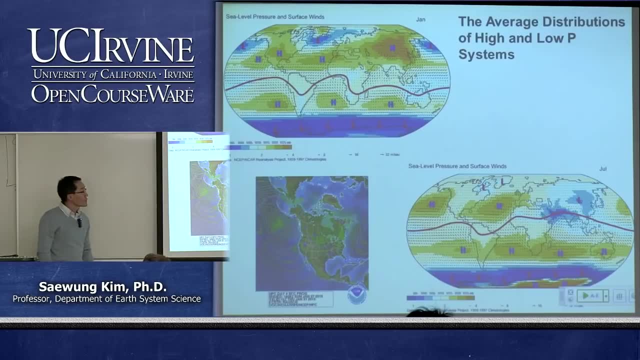 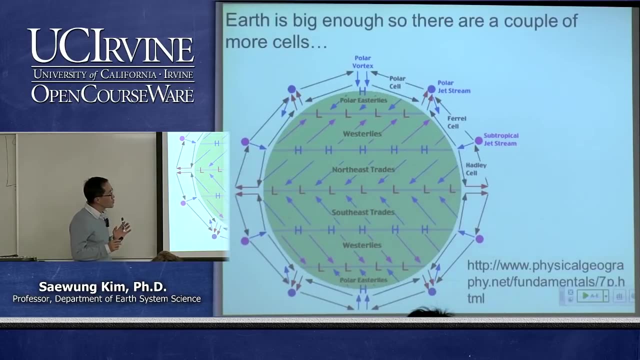 cause low pressure, low pressure system in the about 60 degree north or 60 degree south region. Okay, But real world picture is kind of mimicking this conceptual model, but it is a little different. so let's take a look at why it is a little different. 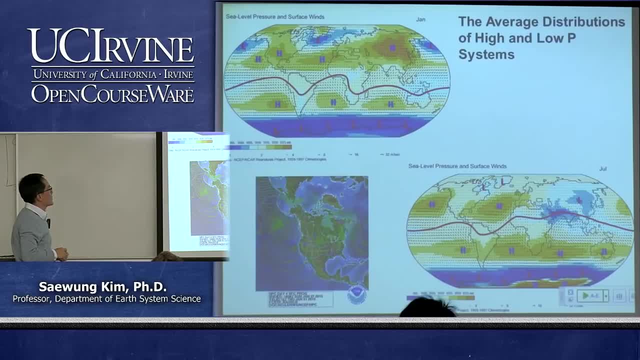 right So so this is surface pressure distribution over about 40 years, so from 1959 to 1997, in January and this is in July, right? So this red line right here is basically low pressure system and then basically this line right here, right. 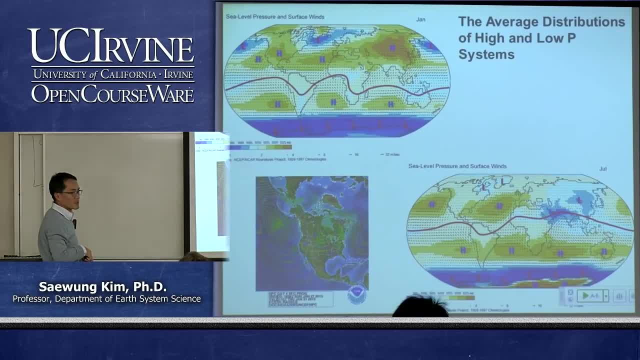 So why this is fluctuating like this at first, let's discuss about it first. anybody can guess it's not really straight line like this to make our life complicated. maybe that's it, but anybody season actually seasonal changes. this one and this one is seasonal differences. 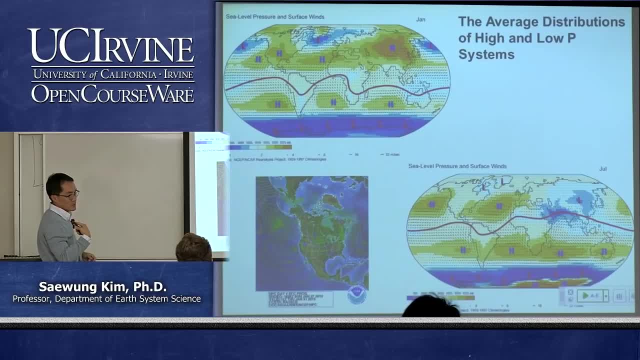 this is January and this is July, so this is basically our winter time distribution. so, first of all, this is a little bit south than the geographical equator, right. so right here it's a little bit south because in January sun is where a little bit. 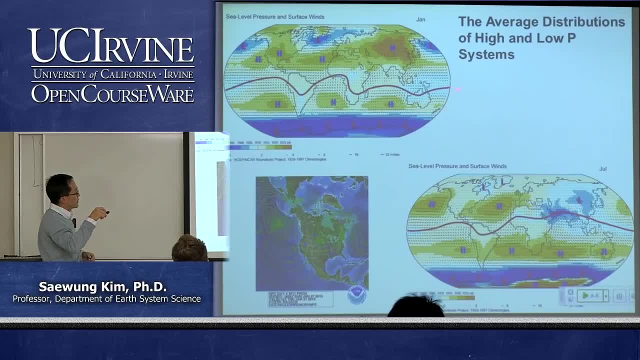 towards the southern, south of the equator, right. So sun is gonna be sitting right here. so this line, center line, moves, moves, move toward the south side, right. That's pretty clear. and this kind of fluctuation is happening due to distribution of land masses. so over 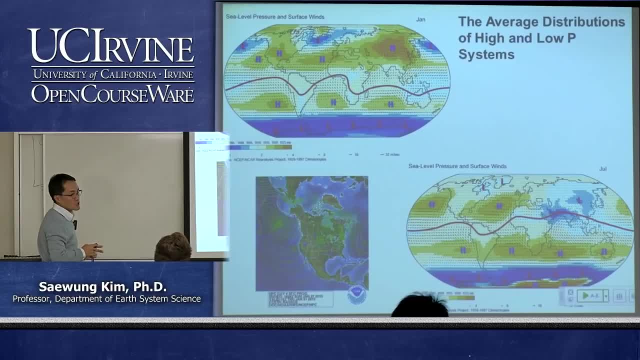 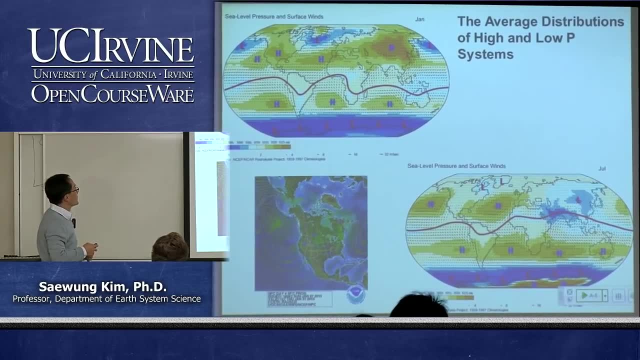 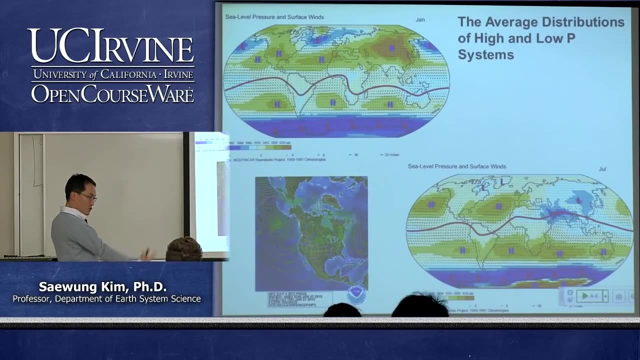 the ocean. so water, you need more energy to heat it up, right, but the land, you need less energy to heat it up. so that actually makes some differences in terms of the air motion too, because air motion is pretty much dictated by pressure system. and if you think about 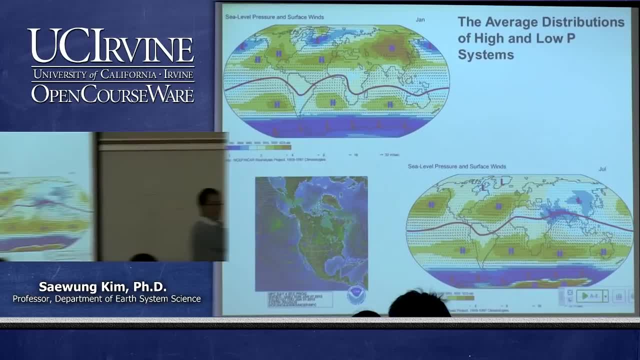 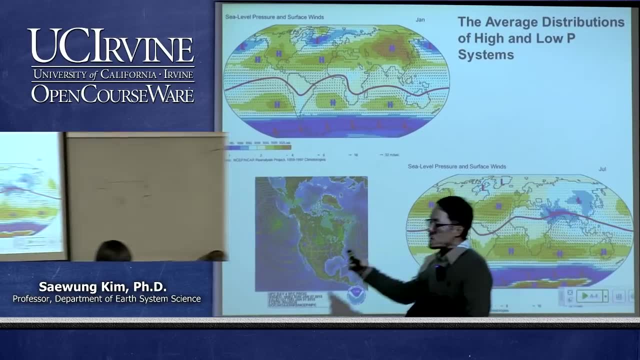 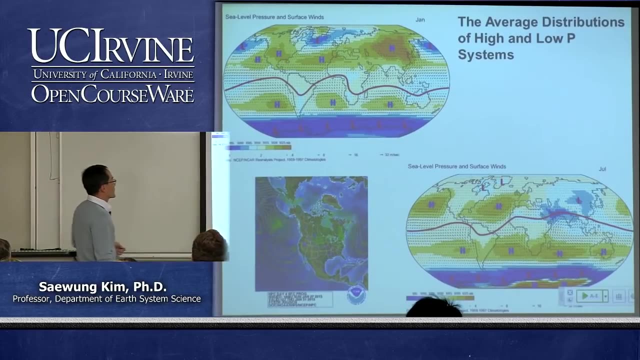 this ideal gas law: different pressure will gives you different pressure. different temperature, sorry about that. different temperature will gives you different pressure. so this land mass and then ocean distribution make your- at least not your- life, our life make very complicated as a scientist studying earth. so if so, 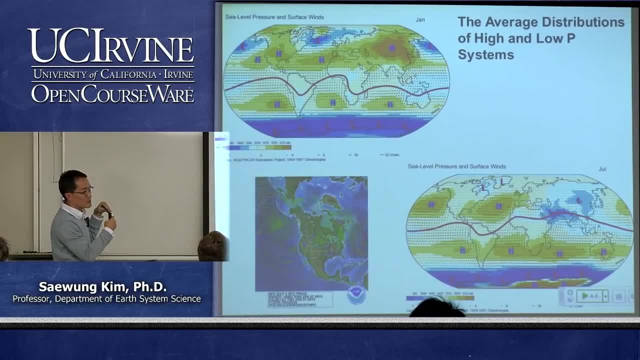 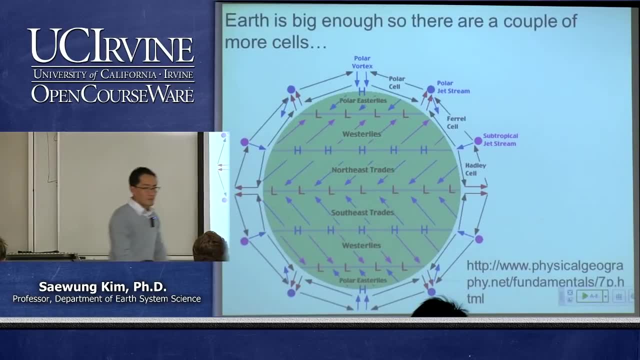 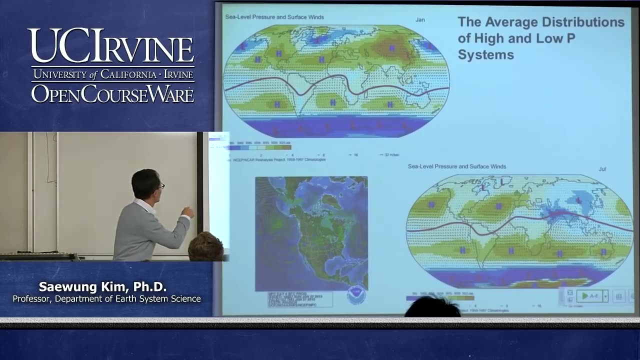 and then if you take a look at the high pressure system distribution and the low pressure system distribution, at least in the southern hemisphere, is very consistent with this conceptual model. right, you have high pressure system about 30 degrees south and then low pressure system, consistent low pressure system. 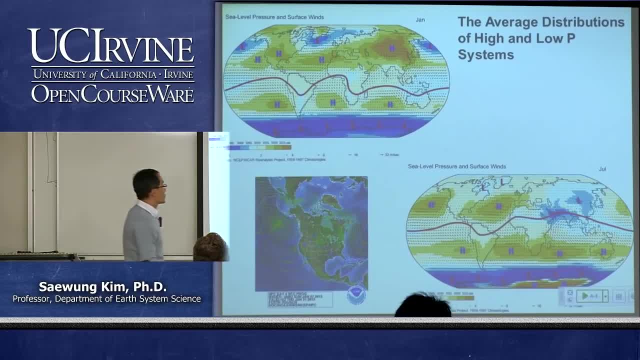 in the 60 degrees south right, but in the northern hemisphere it's a little more complicated. we have a high pressure system right here and a low pressure system right here. it's especially in the winter time. it looks like I agree with this conceptual model, but in the 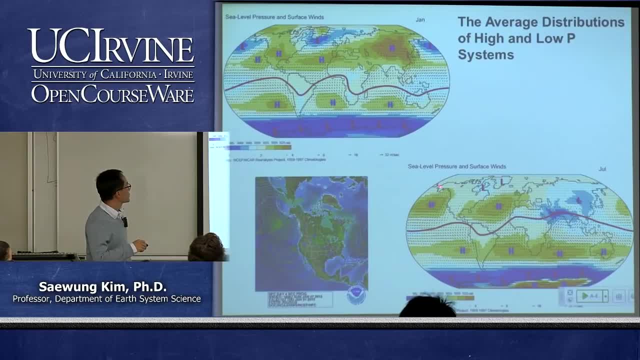 summer time, which is in July, we cannot really see this low pressure system right here. and then, if you take a look at the, this big chunk of mass of land, the high pressure system usually observed during the January and the low pressure system is observed during the July. 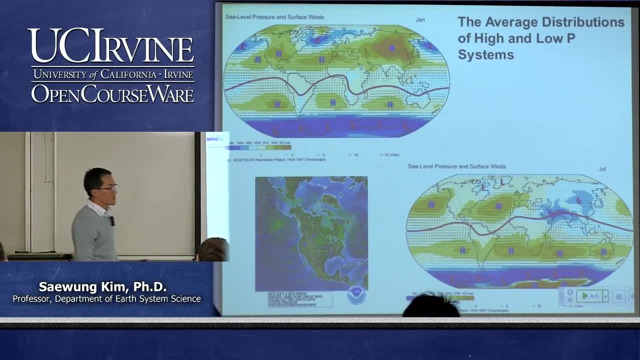 in the summer time. so this high pressure system and the low pressure system over the land is pretty much caused by land gets hotter during the summer time. that cause the low pressure system. so if you imagine that there's land mass and then sun is right there, then land. as I said, there's less energy to heat it up. so land is going to be heated up during the summer time, in July. then what kind of air motion is going to be happening? aboard air motion? and then that's, by definition, low pressure system. so this: 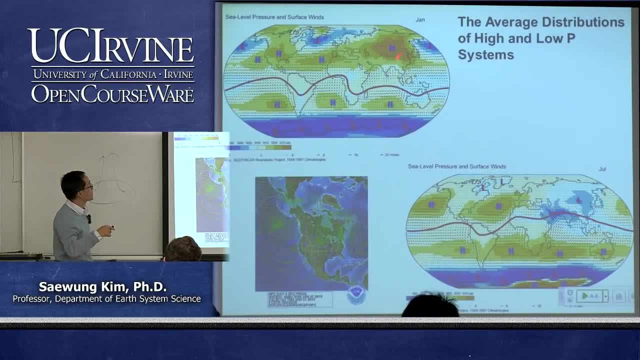 low pressure system over the land during the summer time and the high pressure system during the winter time is caused by kind of a this land, the temperature kind of differences between the summer and winter over the land, and then that makes this pressure system really complicated. and then this: 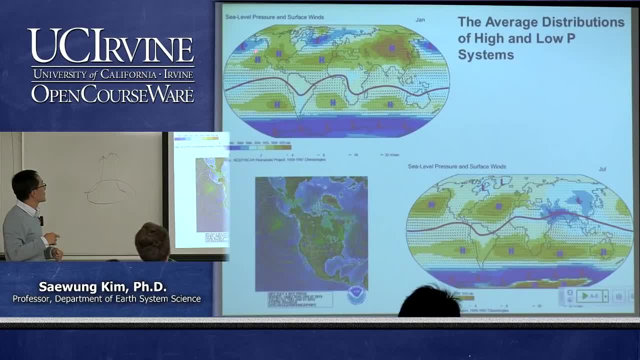 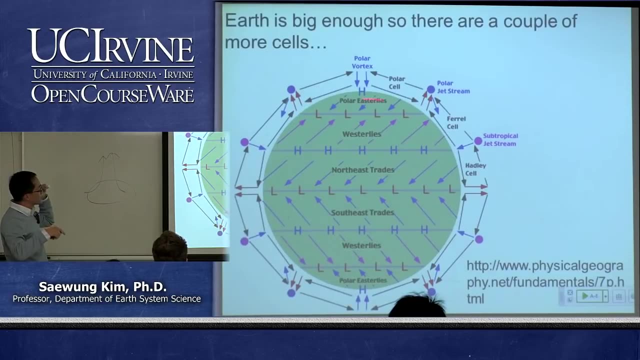 low pressure system is same thing too. so in the low pressure system during the winter, summer time, because this land over the northern American gets hotter, so this high pressure system get expanded, so this low pressure system that caused by this general circulation model is moved towards the northern side. 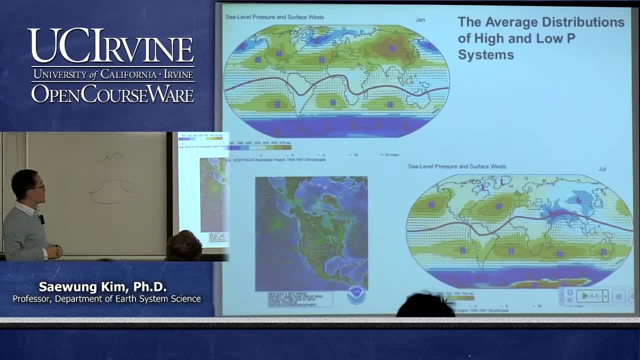 and in the winter time this low pressure system gets expanded to little bit towards south again. this low pressure system in the North Pacific actually cause a lot of rain in the Pacific Northwest, like state of Washington and Oregon, and sometimes this expanded to the Southern California. that makes the rain. 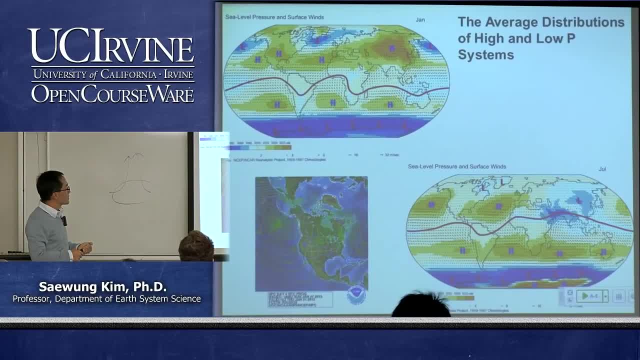 in the Southern California too. so the bottom line here is that there's a permanent high pressure and low pressure system out there and then, due to the land mass, heating and cooling, there's kind of temporary high pressure and low pressure system is evolved, depends on the system. 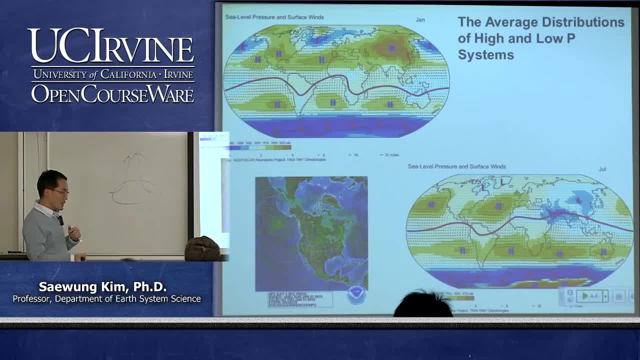 okay, there's a permanent low pressure high pressure system and then temporary seasonal high pressure low pressure system is happening in average and then those kind of high pressure low pressure system affecting our weather, also air pollutant, transport phenomena, so we'll discuss about it later. towards the 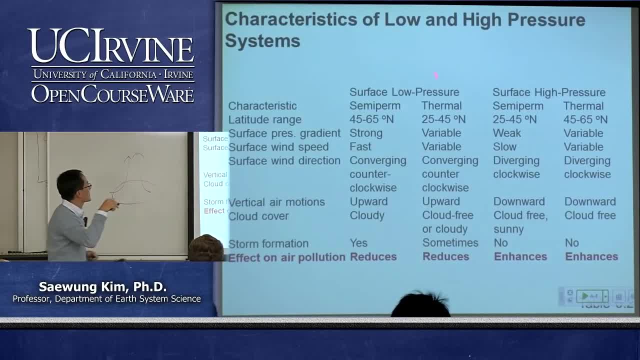 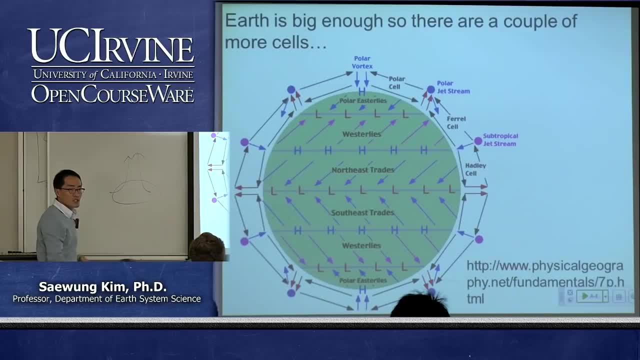 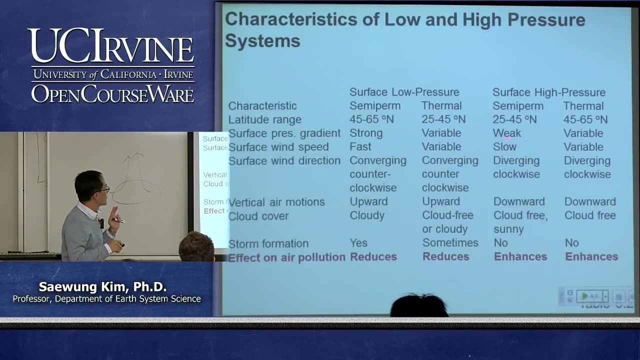 lecture or course. so this is summary. so this is semi-permanent pressure system that is caused by this general circulation. so in 45 to 65 there's always low pressure system, and then 25 to 45 N there's high pressure system and then there's 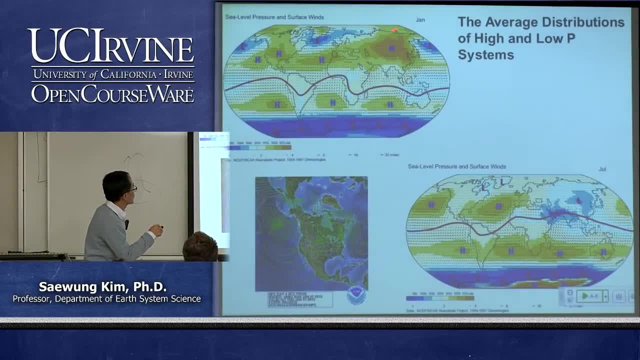 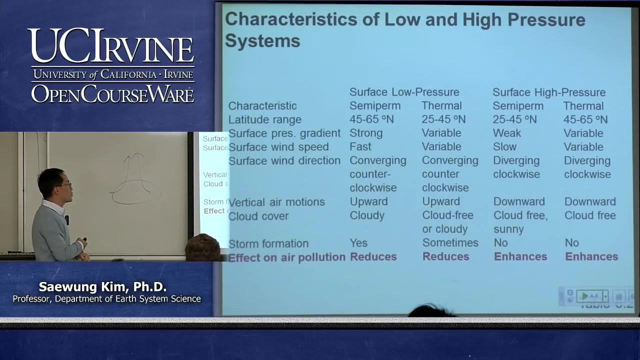 thermal high pressure, low pressure system that I explained. as I explained, usually during the over the land, during the air, because land gets hotter, the air is moving from the surface to the atmosphere. that cause the low pressure system. so that's what you call thermal high pressure and low pressure. 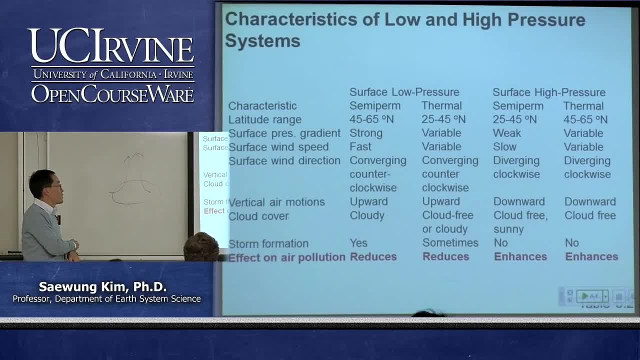 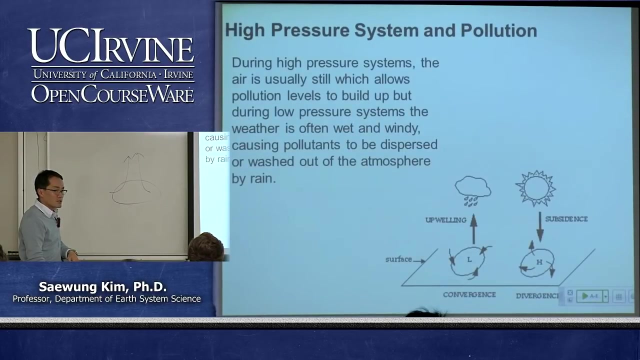 system and then implication towards the air pollution is that usually low pressure system reduces the air pollution. if you remember that London 1950 something 52, the London big smog episode it mentioned about high pressure system- is sitting over the London, then there's very calm. 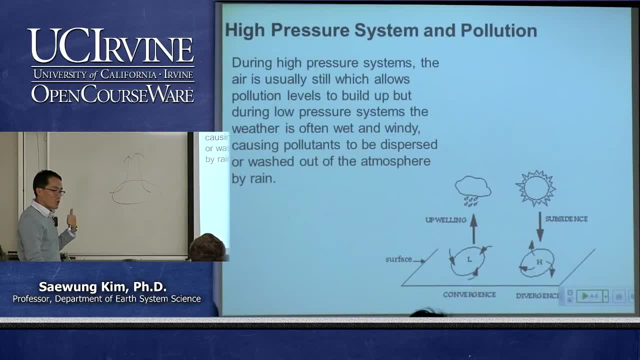 and clear day caused the accumulation of the pollutants over the surface. and then we watched: it was very calm day and clear day and then cause that accumulation of air pollutants over the surface again. the video clip that we watched this class also. the high pressure system was sitting. 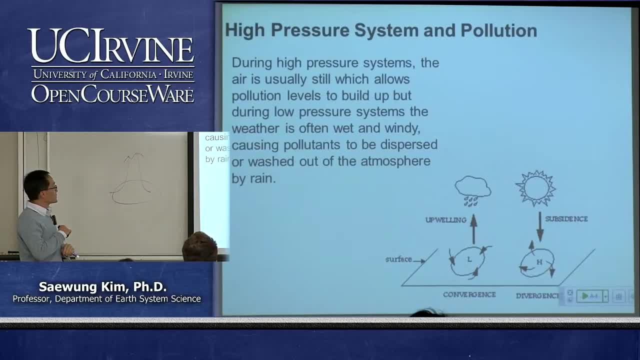 over the city and then air pollutants accumulated over the city surface right. so this is the example of high pressure system and then high winds, so air pollutants can spread out, and then low high pressure system. right here is kind of a push to the downward, to the air. 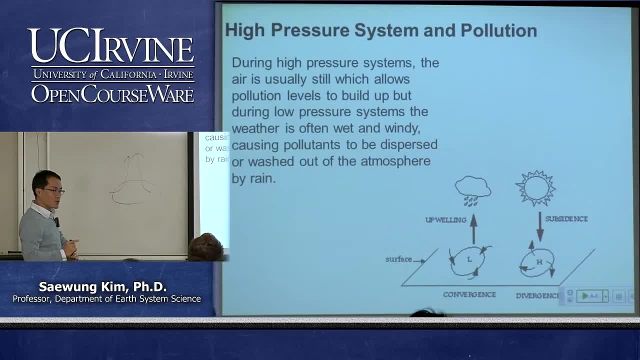 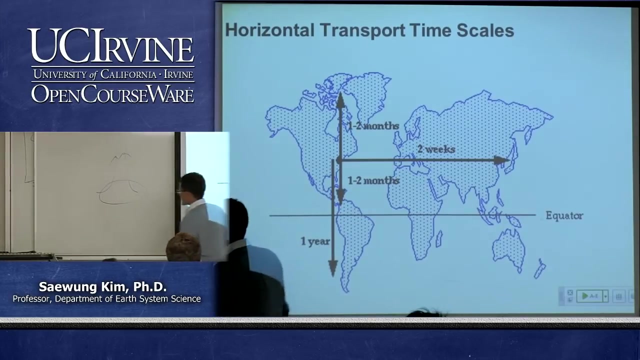 so kind of a: the depth of the air motion is shrinked in the high pressure system. so that's kind of a how the weather system and then air pollution is tied into one thing, right? so this is bottom line again. summary slides about the air motion, maybe this: 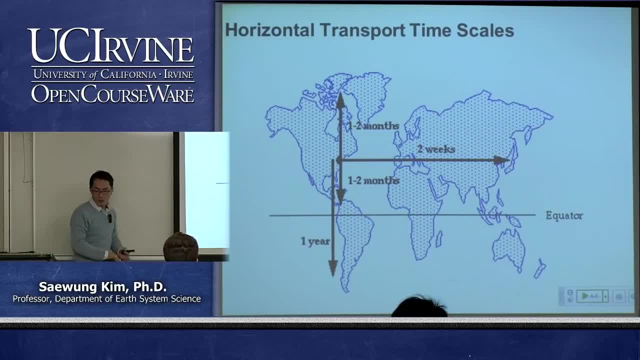 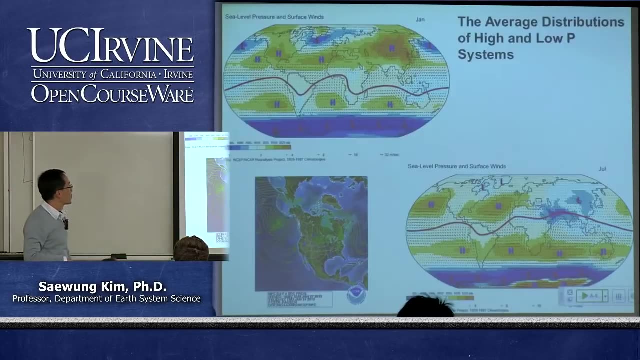 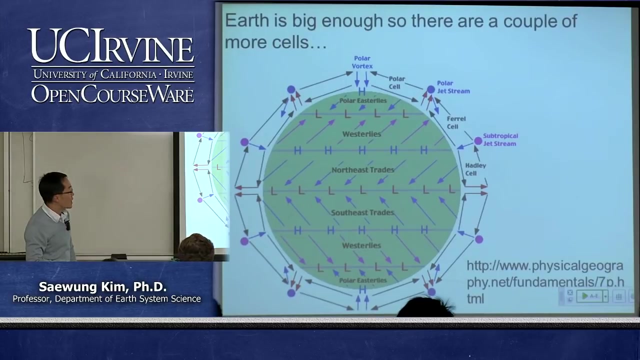 is, this is not the last slide, so. so basically this right here basically blocks the air mixing between northern hemisphere to southern hemisphere. so if you go back to this plot again, so sun is right here, and then because of this kind of a motion of the upward motion, 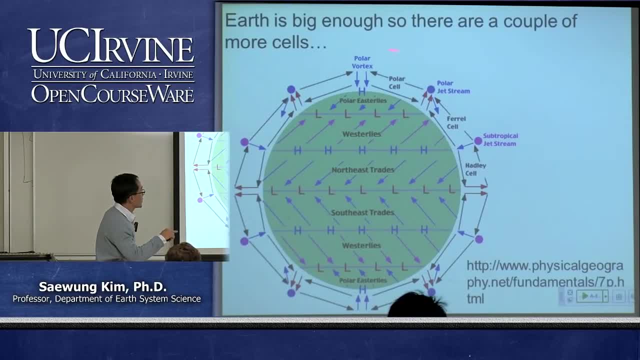 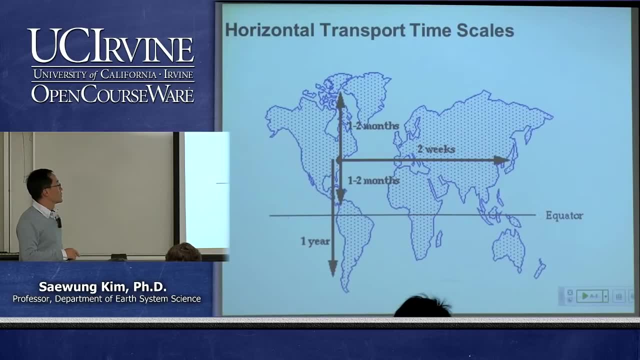 of the air near the equator. basically this blocks the air, the pollutants mixing. so it takes really long time for air pollutants or other atmospheric constituents to mix from northern hemisphere to the southern hemisphere. so it takes about a year to mix the air between northern hemisphere and then. 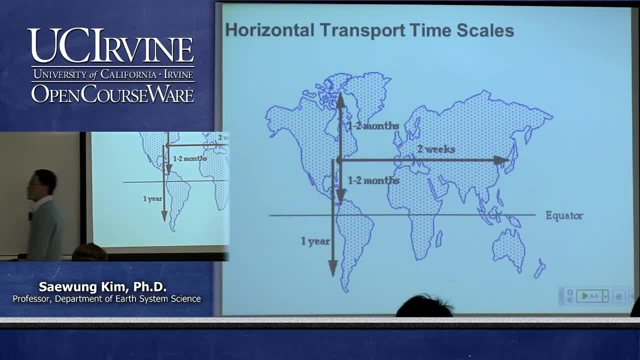 southern hemisphere. so let's assume that air pollutants that lifetime from the northern hemisphere, then if, according to this time scale, then that specific air pollutants cannot be observed in the southern hemisphere because this air circulation model dictate that it takes about a year to actually completely mix in the 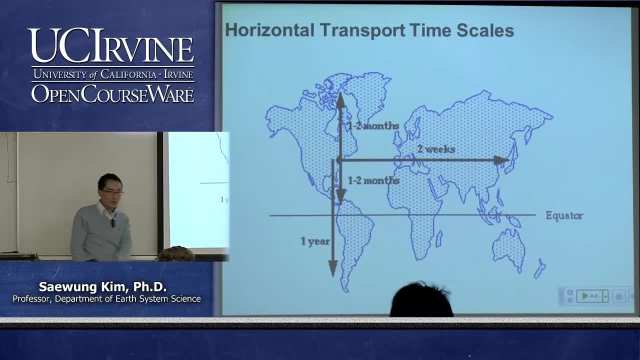 northern hemisphere air pollutants. so if it's far much shorter than one year, then you cannot. that specific air pollutants cannot be transported from northern hemisphere to the southern hemisphere, right? so that's how you can relate with the lifetime of the air pollutants, and then this in the 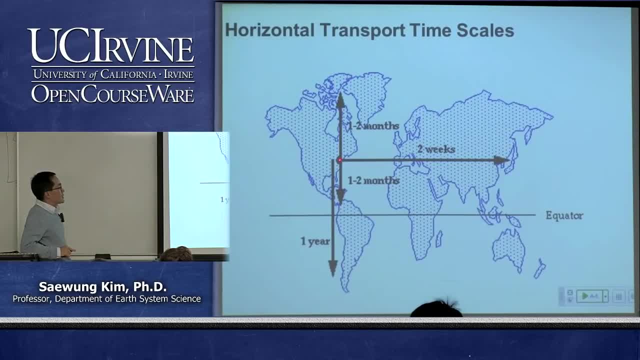 this north to south motion, but this westerly motion, so from north america to europe, asia to the us. it is much, much more efficient. it takes about two weeks from air masses transport from from the west east, all the air motion if affected by the coriolis. 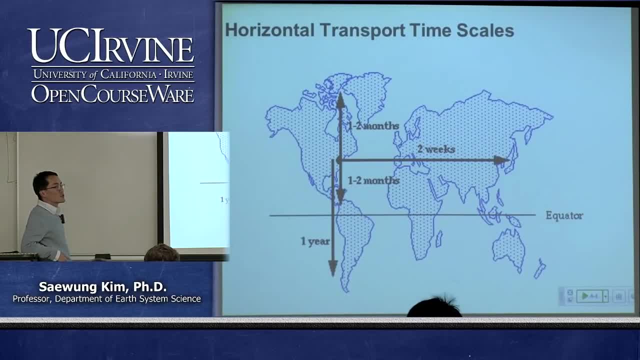 force, also the jet stream. so that's why that people in the west coast of the united states complain about the air pollution from china or south of the us, because it's much more efficient transport of the air pollutants from the west to the east side. okay, so. 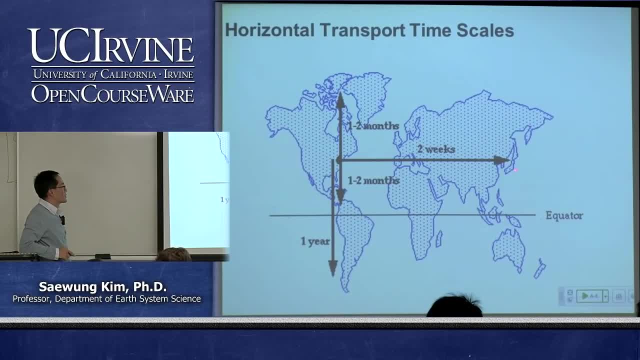 even in the, even in the far east asia, if you just if you take a look at the border between the big cities. so i think west part of china is mostly mountain and then most of the chinese population located in the west, so it's always from in. 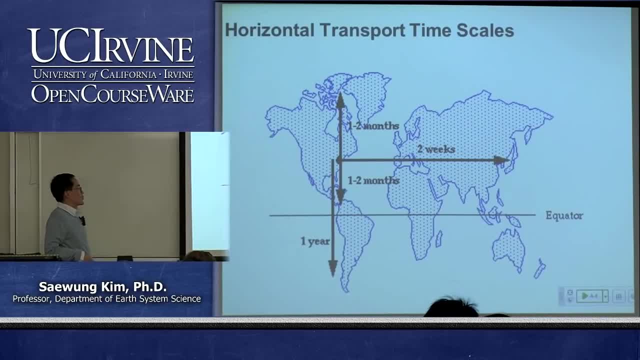 a grand schematic: from west to the east. so actually the air pollutant transport from china to korea, and then korea to japan, and then china to japan. it's always from west to the east. so this is what, how air motion dictates, air pollutant transport. 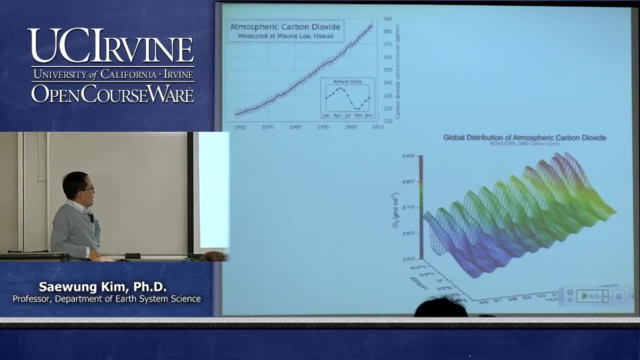 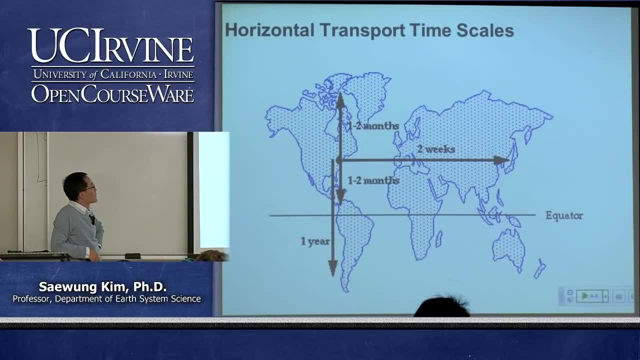 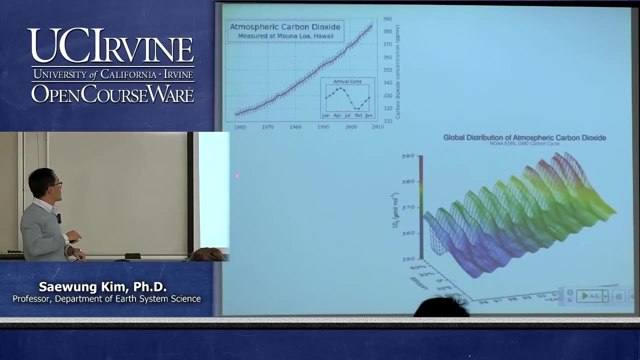 so this is another example of the y meteorology. and then this time scale, this plot, at least this one right here. so basically from 1960. so this is mauna loa, hawaii, which is northern hemisphere right, has been increased past about 50 years. 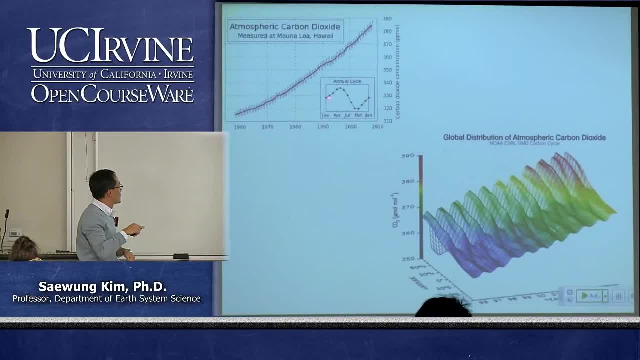 right, and then it has CO2 concentration about april, let's see in the northern hemisphere, and then october is the lowest point of CO2 in the northern hemisphere and then there's annual cycle right here is caused, and then- this is one point observation in the 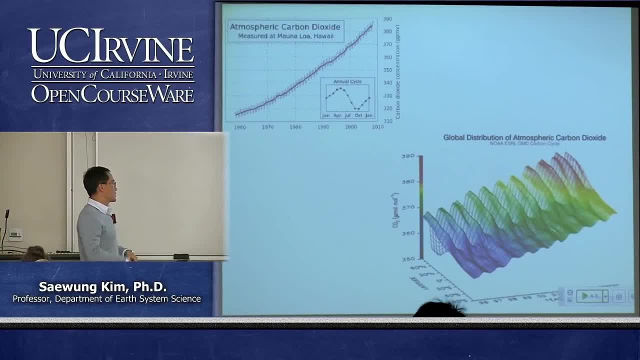 northern hemisphere and then, after doctor killing, started this experiment. this network of CO2 observation has been expanded to everywhere over the earth. so now we have this low CO2 concentration, about 350 to 390 ppm, and then wake up. now time to wake up, i told. 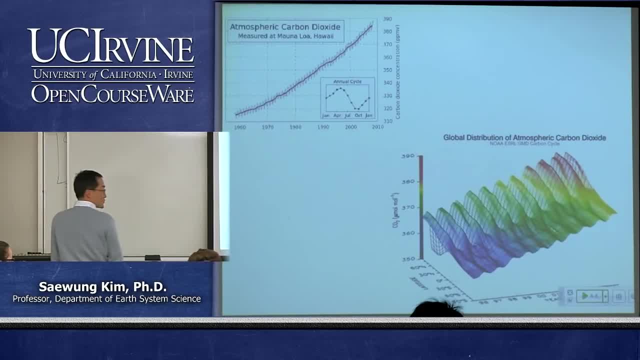 you that i already finished to compiling the midterm right. so you, this is the equator right here. so this is the equator right here. right then, this is northern hemisphere, from 0 to 90 and then 0 to 90 south. so this is southern hemisphere. 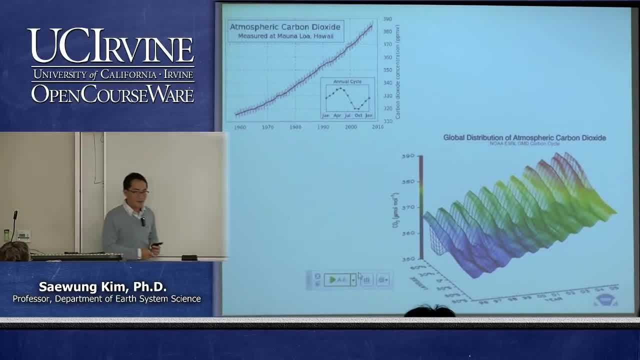 so this is from 96 to. let's take a look how many most striking thing you can see out here. can i yep, go for it? the equator is getting more and more carbon dioxide. equator is getting more and more so if you follow this. 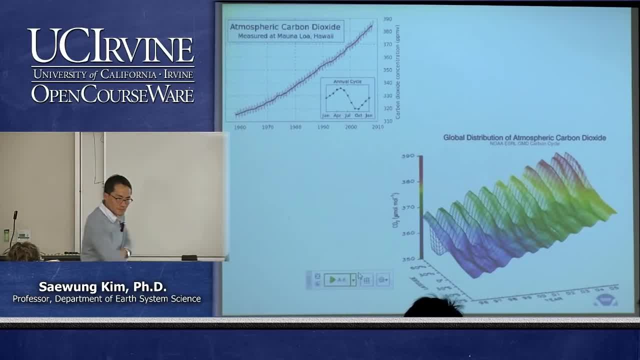 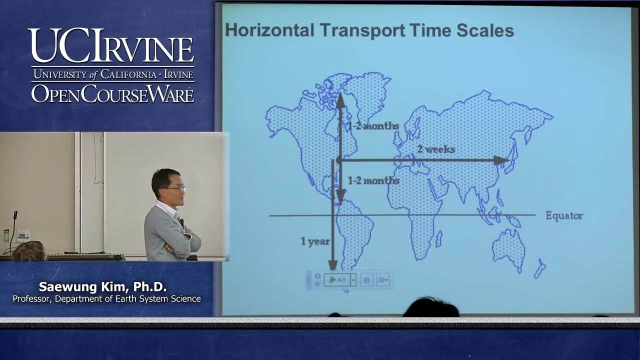 line right here. so basically, the increasing trend of CO2 is everywhere right in the equator, and so the equator is higher than southern hemisphere in terms of CO2 concentration. so why is that? let's go back here. so why northern hemisphere CO2 concentration is? 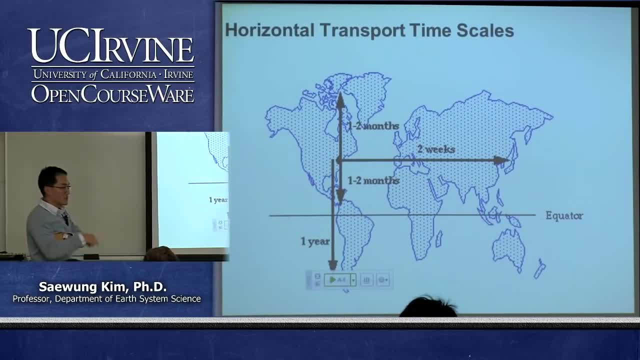 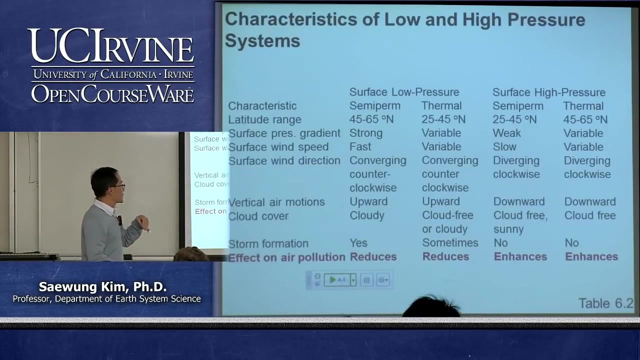 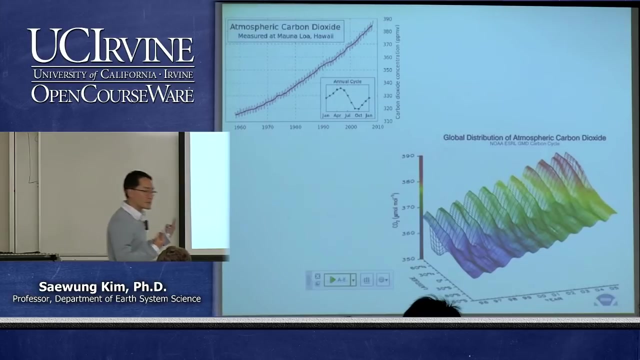 higher than southern hemisphere. where is coming from people, right? so where's more people living from over the land, right? we cannot live over the surface of the ocean, right? so there's more people obviously in from this plot, right? so any other thing can. you can observe here: 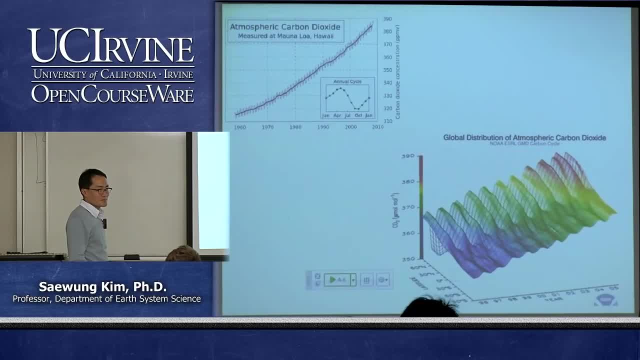 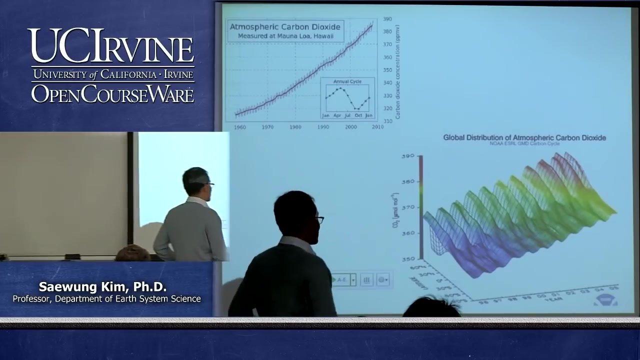 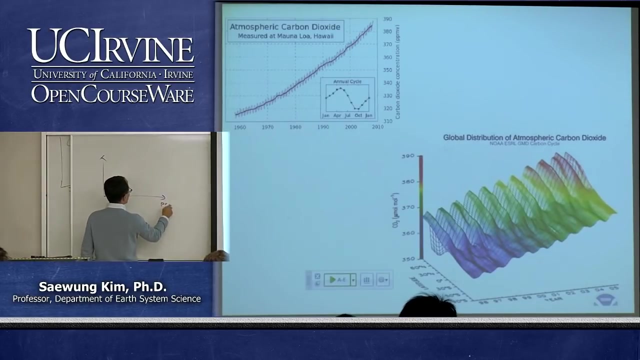 any other. no, so this fluctuation between winter to summer in the northern hemisphere is bigger in northern hemisphere or southern hemisphere. so northern hemisphere is bigger, right? why is that so? if you think that? so basically this is, let's say, this is december, this is january. 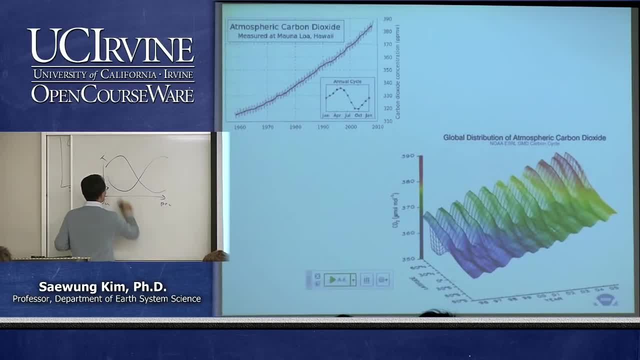 and then you get this amplitude of the fluctuation. so if you take a look at this you can get the information, best information, out of it. so your amplitude in the southern hemisphere it's southern hemisphere, the northern hemisphere, it's. so from the one plot you can get. 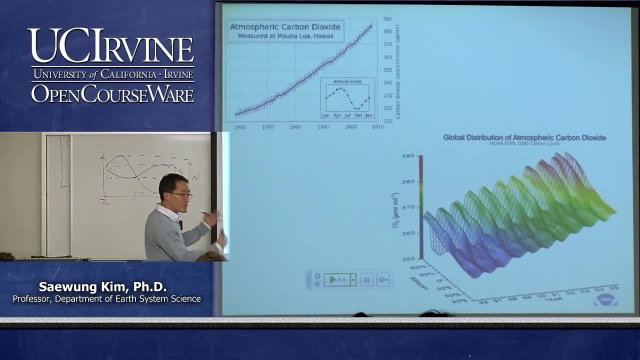 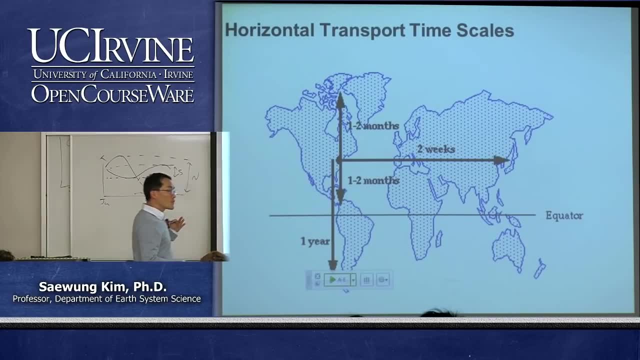 a lot of information out from the one plot and then you can tie- this is chemical observation. but still you can tie into this one chemical observation with totally different kind of thing, which is air mixing time scale. right, so you can understand one simple observation. this is not simple. 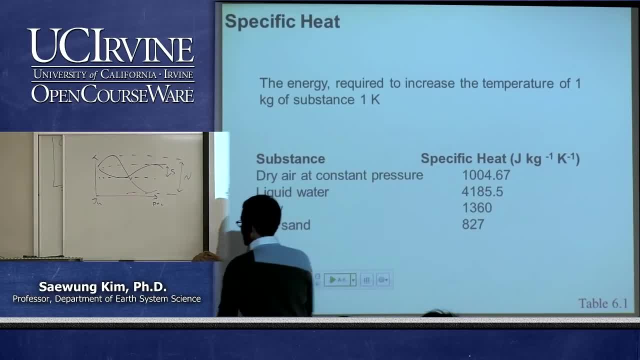 one observation: okay, so specific heat. so this is fancy word, but if you take a look at what that words meaning, then that's not really the answer. so you can see that this is the temperature of the one Kelvin, right? so for example, water, you takes a lot. 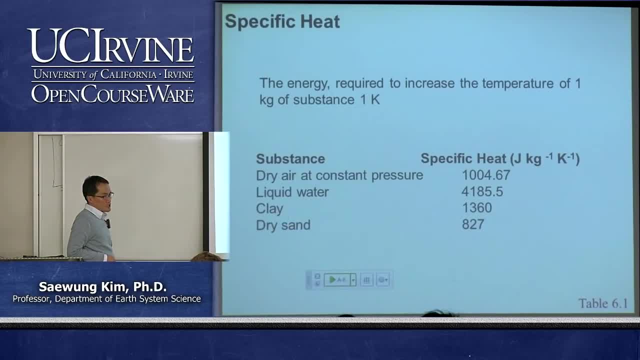 of energy to increase one Kelvin of temperature. okay, if you take a look at the number. but, for example, dry sand or clay, which is basically land, it takes less energy to increase one Kelvin of temperature compared with water. right, so that's the what you can learn from. 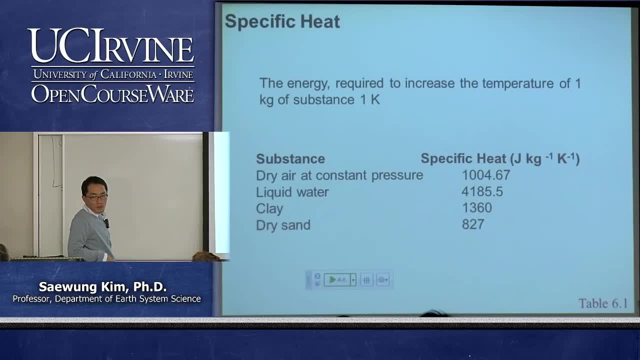 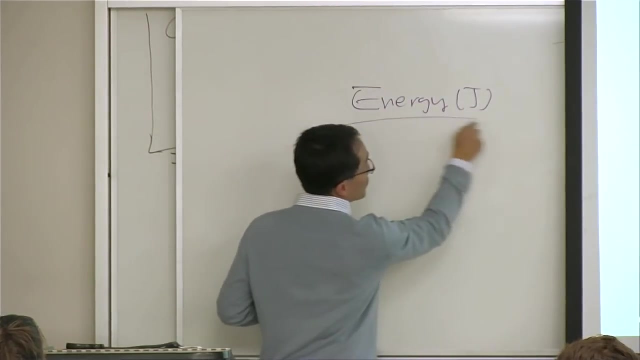 this numbers? yep, if it takes less energy, does that mean it has a smaller specific heat or greater specific heat? smaller number means that takes less energy? because, yeah, yeah, so basically this is right here. so this is energy, which is joule per kilo mass, which. 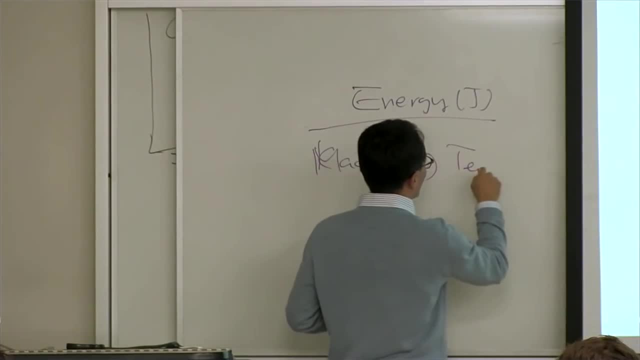 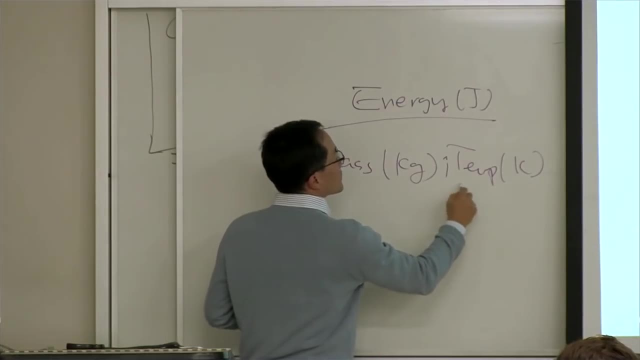 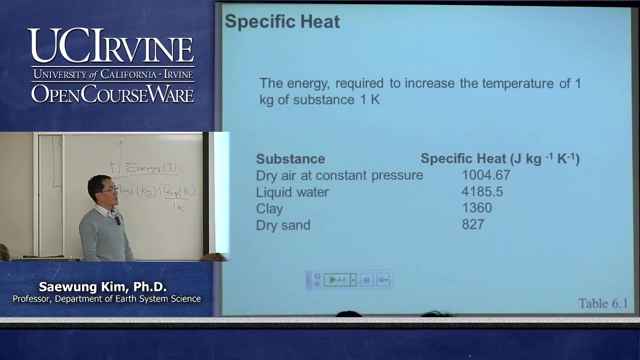 is kilogram in here and then temperature Kelvin. so if you want to increase one, so one, one Kelvin of temperature if you, whether you need higher energy or last energy, counting right. so basically, land needs less energy for temperature increase. for if you think the other way around, 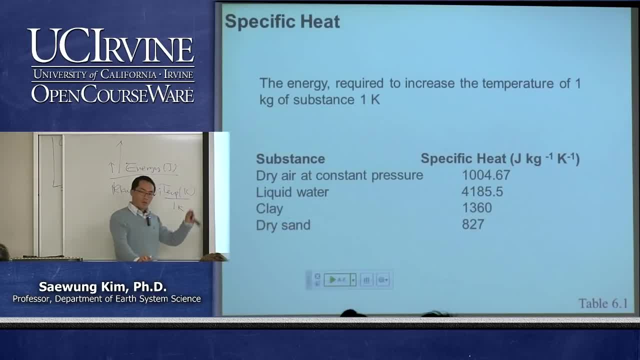 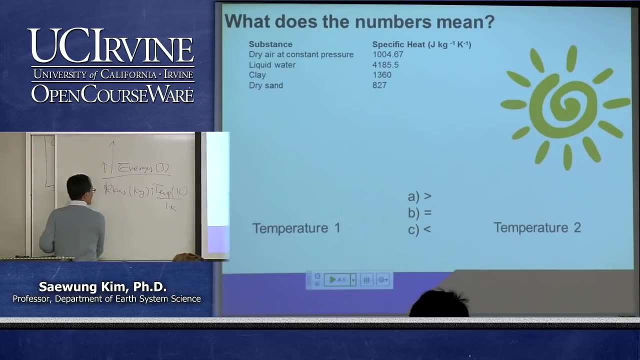 then if there's the same energy is given to land and water, then land is going to be heated up much faster than water, right? so from this number let's take a look at how this thing will affect on the air motion. so you have land here. temperature. 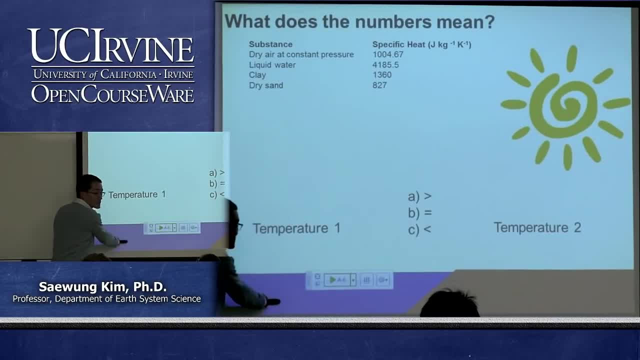 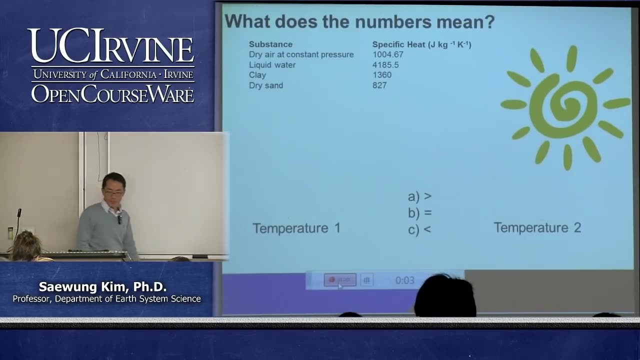 two water here, then water has higher specific heat right than the land. so during the daytime sun is up. then which temperature is going to be higher over the land? temperature two: over the ocean temperature one: who doesn't have the i clicker? today everybody has i clicker. 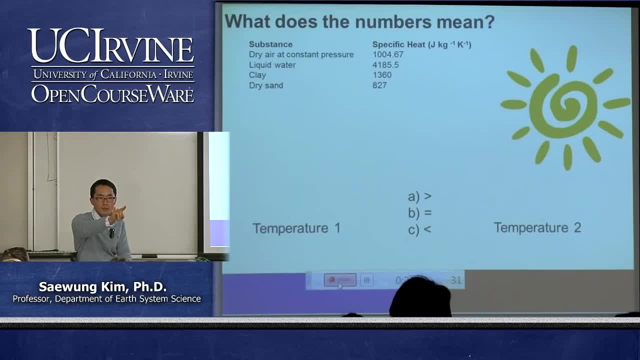 one, two, three, three. would you? hey, ian, would you do some how many students are? would you count the how many students are here? just try to compare the number that i got and then how many i clicker responses that we actually have today. confusing, i thought. 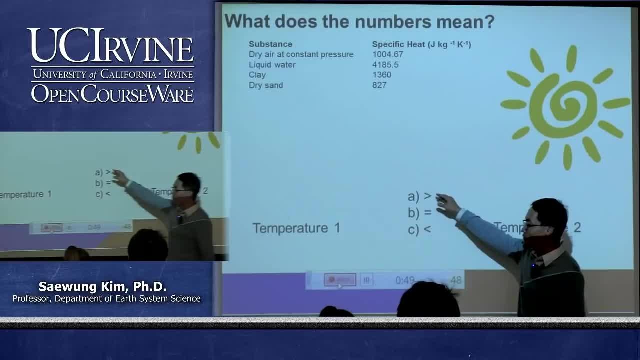 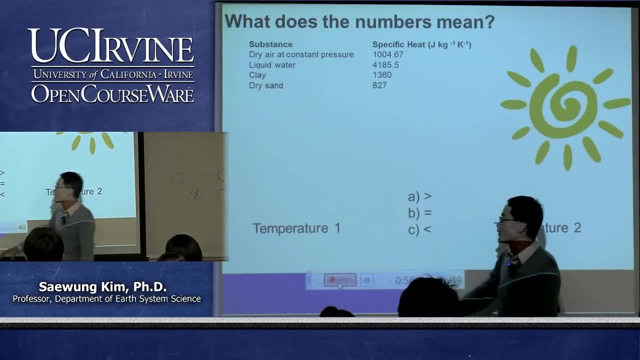 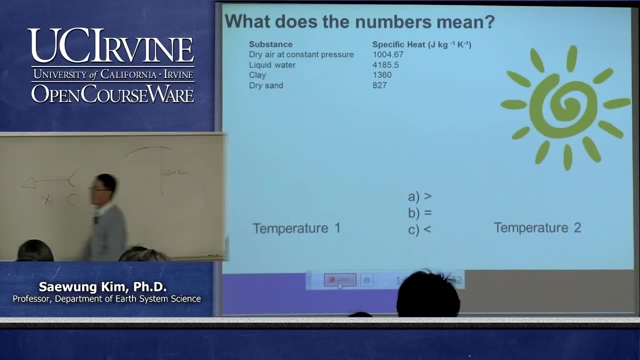 it's pretty straightforward. so a is temperature over the ocean is higher than land, b is same. and then c is temperature over the land is higher than temperature over the ocean and the specific heat of the land is much less than over the water. right, you don't? 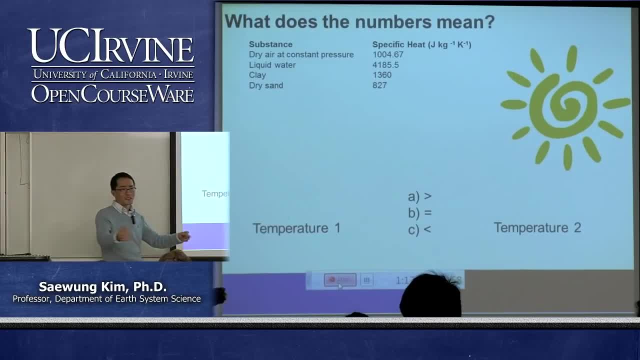 need to even think about that specific heat. what you do when it gets hot over the beach: you jump into the water. right, why you are doing that. i got the only answer 68. so how many students doesn't have the i clicker three, i think we. 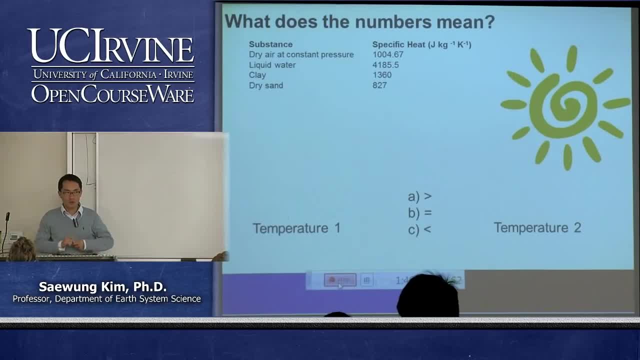 missed three people here, so we need to figure it out who those threes are. so let's take a look at the answer. so there's b- same- and then mostly c- okay, so yeah, i give you the answer right. so why you jump into the water? because 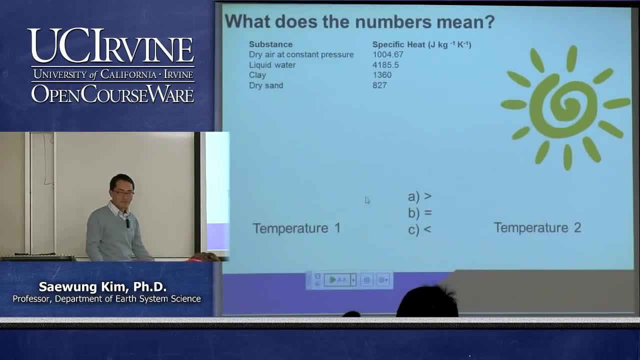 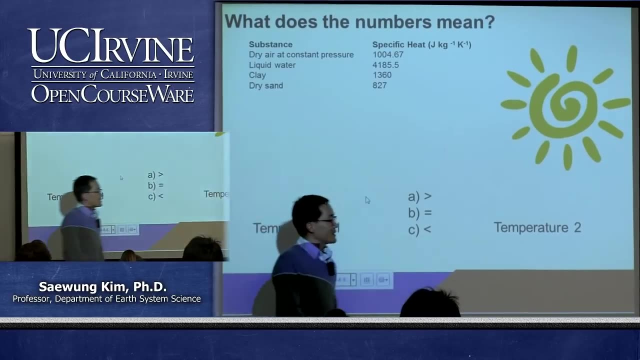 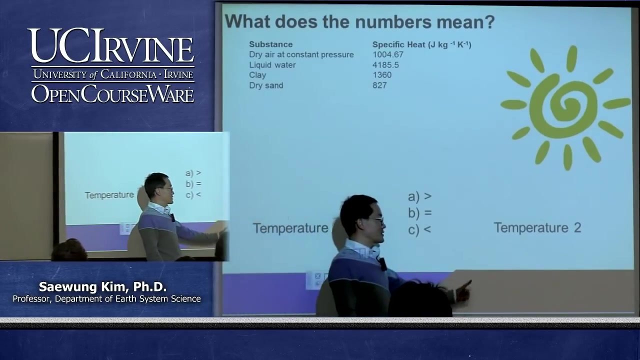 land is hotter than the water, right. so then let's take a look at, let's discuss about a little fancy way, right? so specific heat over the land is less than the water right, which means that it takes less energy to increase temperature over the land than the. 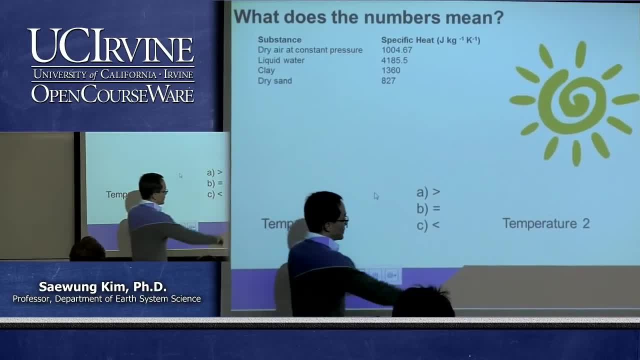 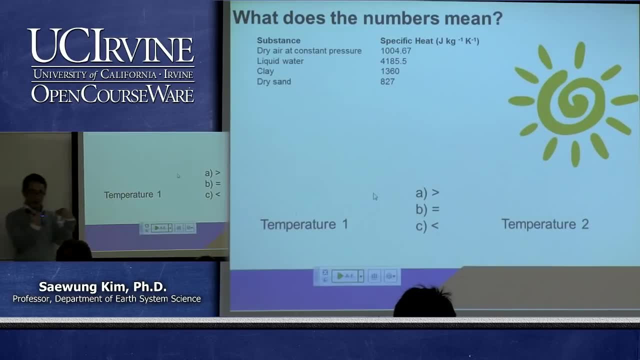 water. and then, in theory, that over the surface of the land, over the surface of the water, takes the same energy, right? and then, if you take a look at the temperature increase than over the land, temperature increase should be higher, right? that's why, over the land temperature. 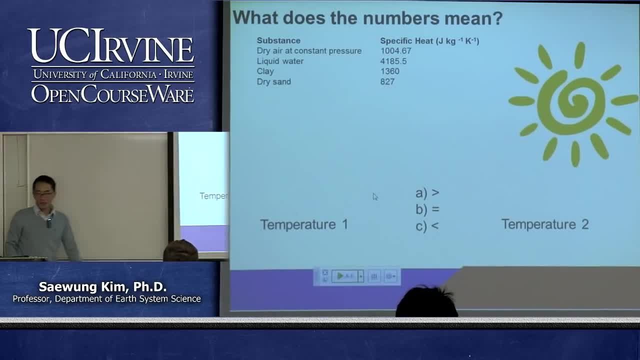 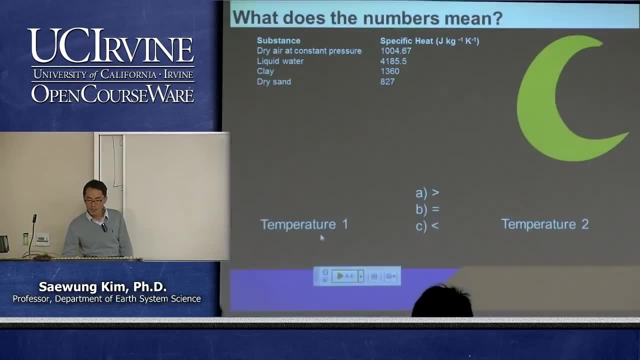 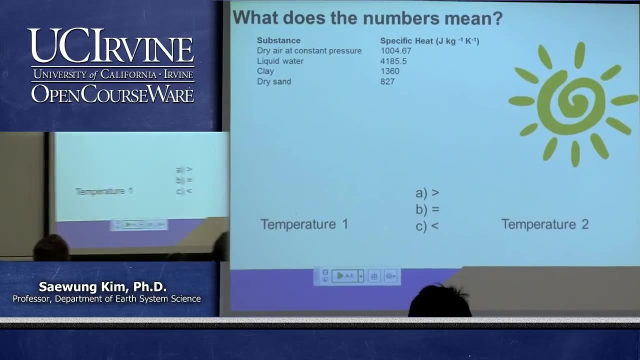 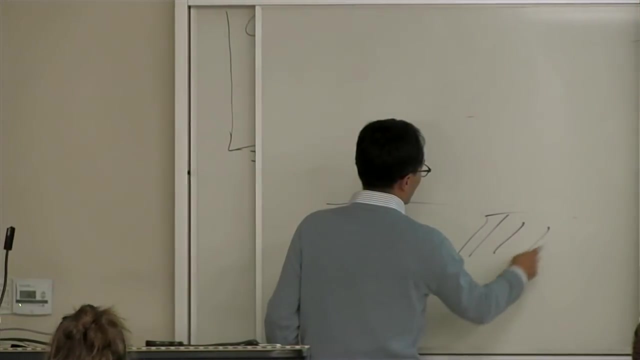 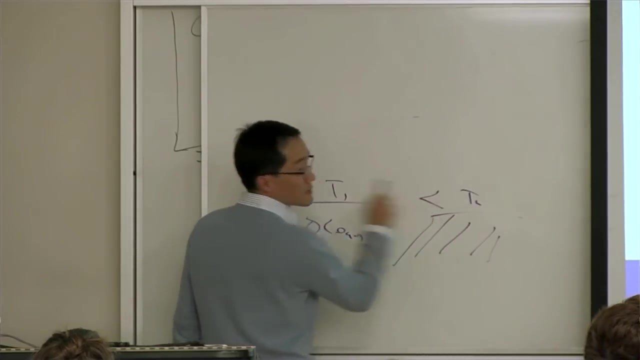 is higher than the over the ocean, right. so this will cause the circulation of the air, which basically that the air is moving up, right. so during the so temperature two, temperature one: this is higher, so air out here is lighter, then it's gonna be moving up, right. 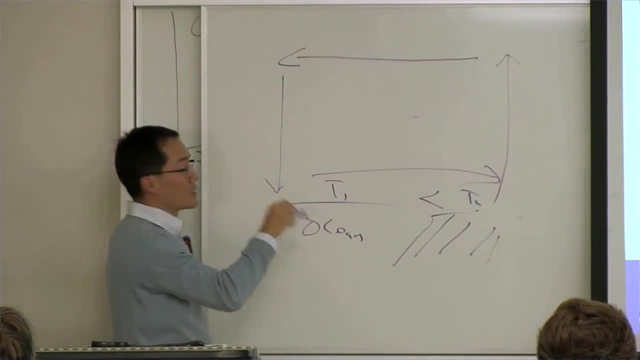 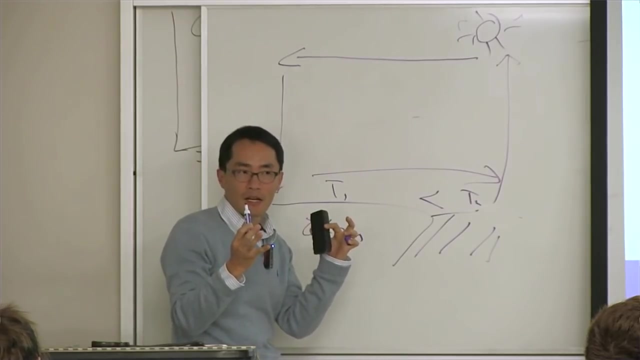 sea air breeze, a sea land breeze is happening during the day time. it's a it's not really high pressure, yeah, you can understand that way, but it is kind of a little bit kind of local scale phenomenon. that's why usually gets the wind, even in the sunny day, high pressure day that usually wind from the sea is blowing into the land during the day time. okay, this is kind of small scale circulation near the beach. right, let's do it again just for fun. what's going to be happening during the night? so cooling? 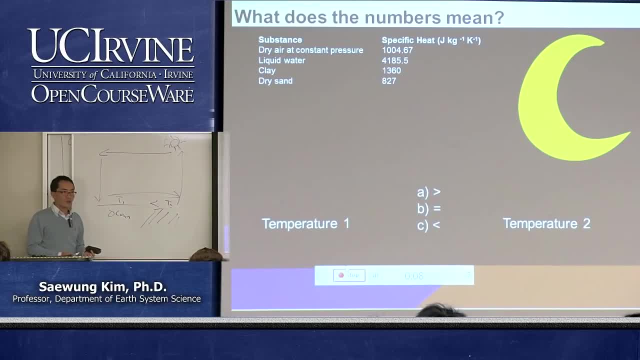 is same thing, right? so cooling of the land is going to be much faster than the water. okay, that's one thing you need to remember. so, temperature of the temperature of the water, temperature of the temperature of the land, which one is higher? we have 62 one. 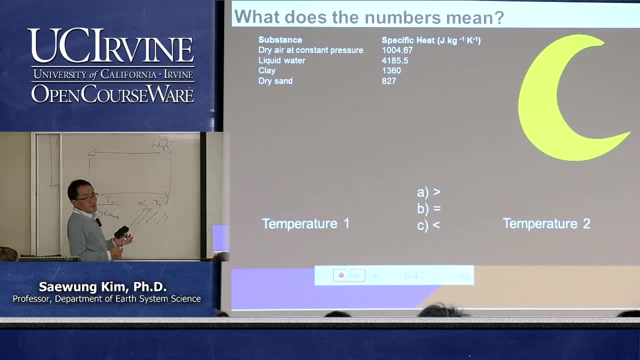 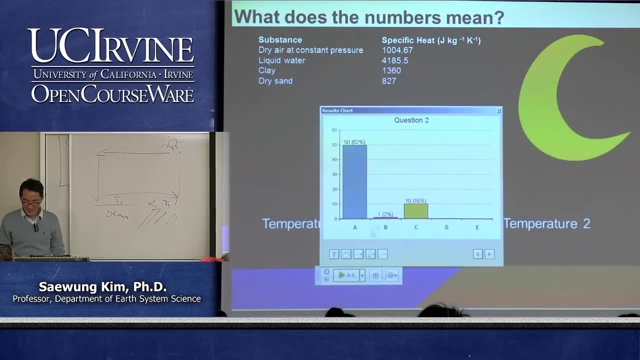 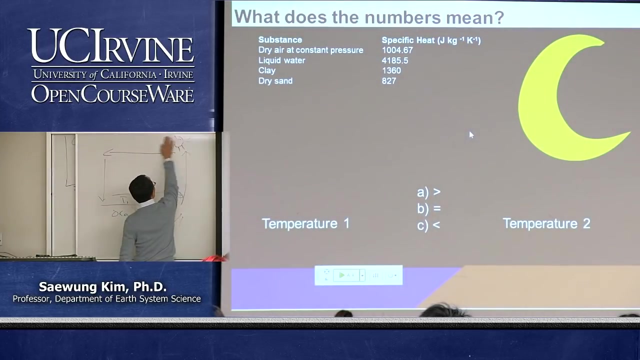 more. it was 62, just before you try to mess up. all right, 61, I will stop this. still 10 people, doesn't get it okay, let's try again. so sun goes away. right, then, these two are cooling down right water and land, and then 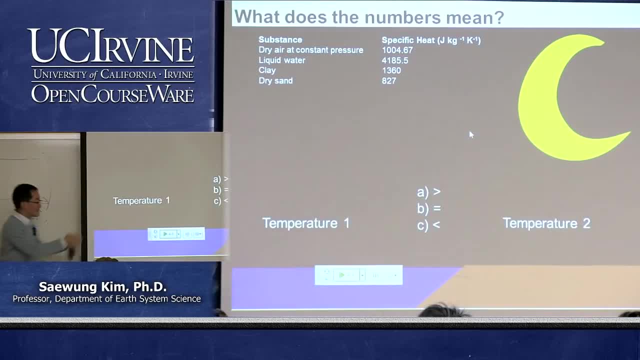 you gotta think about this thing the other way around. right, it's gonna dissipate energy, right? so basically water can contain more energy than the land. okay, so basically water can keep more energy, so the cooling down over the water is much slower than over the land, okay. 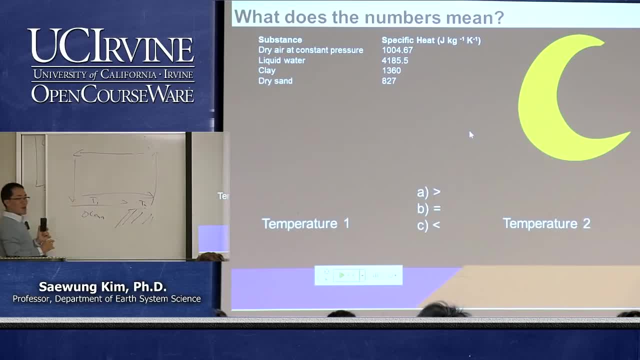 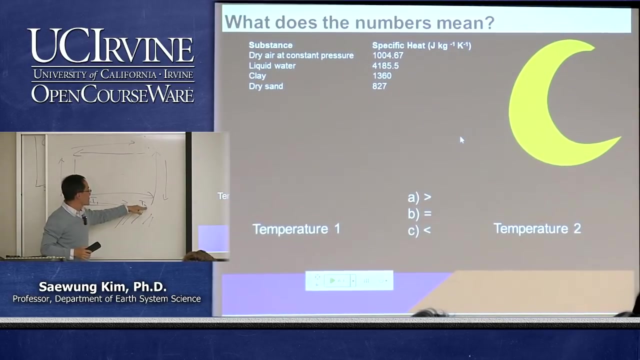 so usually nighttime temperature is the other way around, then what's gonna be happening? the other direction of the circulation during the timeline. okay, so this is why, in general, you can join during the night that the wind direction of the beach is from the land to the ocean. 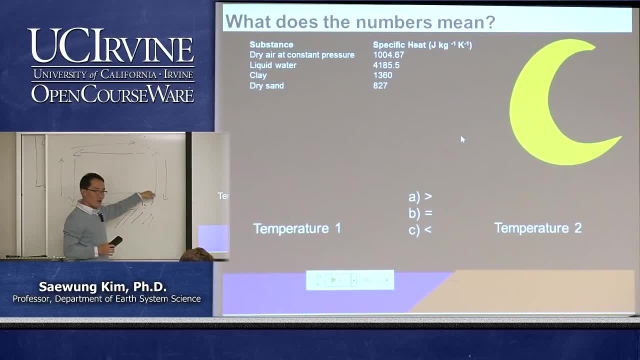 and then during the time from the ocean to the land. so we will discuss about implication about land ocean circulation after the exam and then Thursday we will discuss about the summary slide that I will upload tonight and then there will be exam next Tuesday.